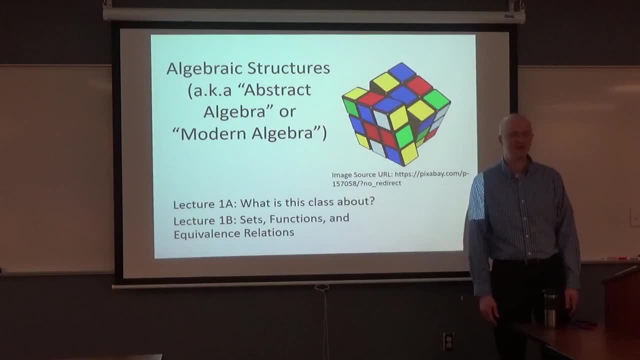 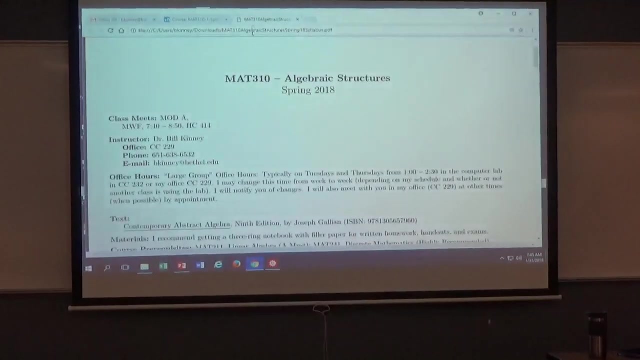 Break up the long class period from 7.40 to 8.50, and that's long for a math class, too, 70 minutes total. So, typically, we'll probably break the lecture into two parts, and I do have lecture 1A and 1B listed here. But today, it'll sort of all meld into one, since we won't have a quiz today. But, typically, to break up the class, help make the time go by, help you pay attention, we'll have a quiz right in the middle of the class. So, we'll probably have like 30 minutes, 30 to 35 minutes for lecture 1A, or lecture A. 5 to 10 minutes for the quiz, and then lecture B will be out at that point. So, let's go over a few quick things on the syllabus. The first quiz on Friday could involve some questions about the syllabus. 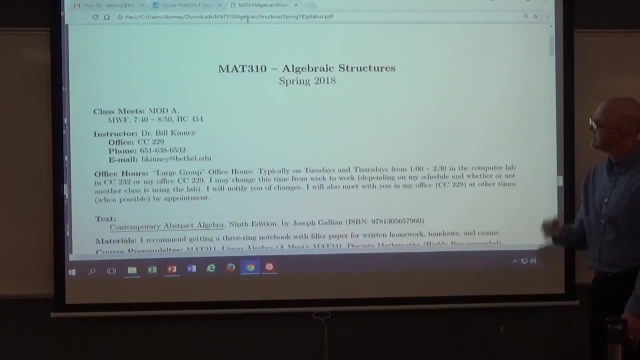 And zoom in a few to there to see some things. 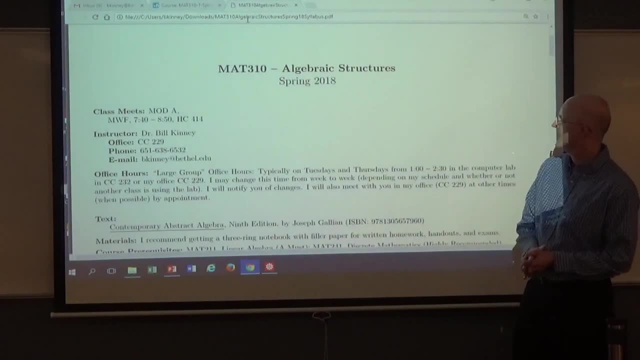 I just want to highlight a few things. First of all, I hope you all know where my office is anyway, but if you don't, CC 229 is by all the other math and CS professionals. 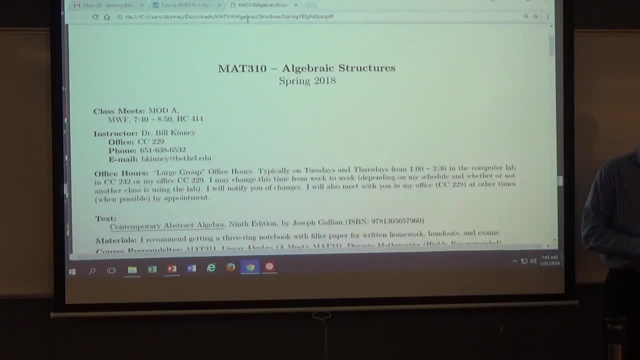 Office hours are going to typically try to be in the Happy Lab. CC 232, most typically. 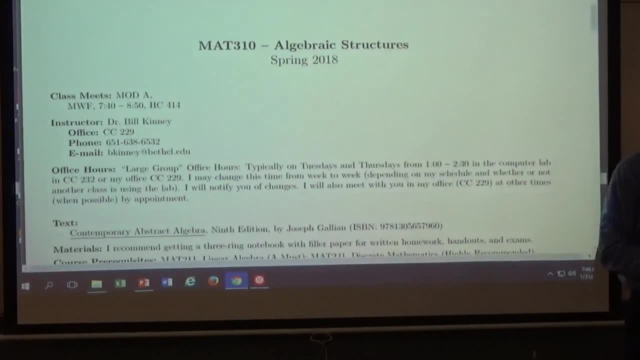 Tuesdays and Thursdays from 1 to 2.30 is the official time. But that could flex a little bit. I'll try to send you a note if it needs to flex. But you're also free to email me if you'd like a personal meeting, if that time doesn't work for you. And we can try to meet personally. 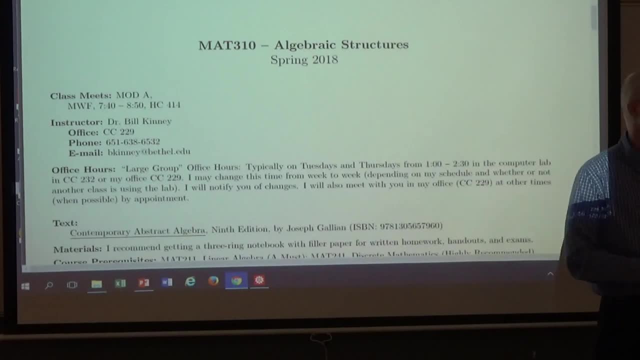 This is a class that is pretty tough, and you're going to want to work together. 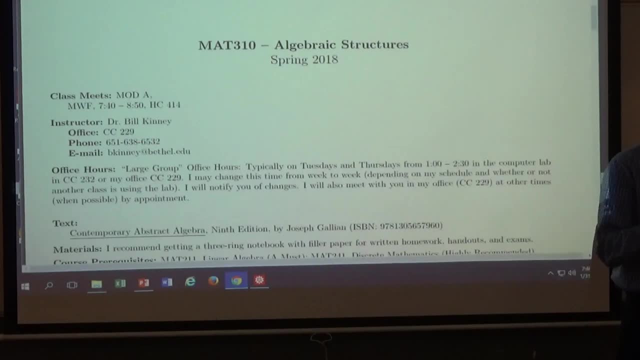 Form groups to... Problem solve together. Not copy each other's solutions, but instead problem solve. Try to figure out how to solve the problems. How to write the proofs. And then you go and you write them up on your own. Though I don't think it's a bad thing if you ask a friend to check over your work. That would be fine as well. Give you advice. 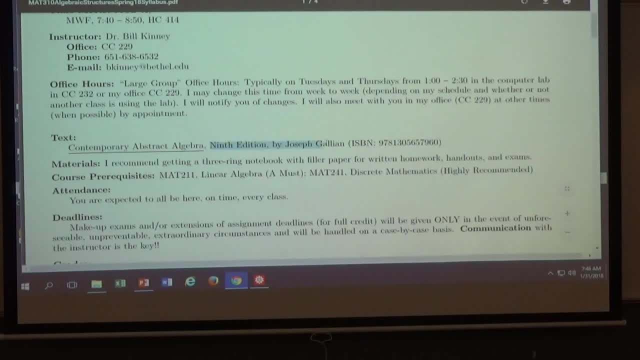 Our textbook is Contemporary Abstract Algebra, 9th edition by Joseph Gallion, who I believe is still at the University of Minnesota of Duluth. Not too far. 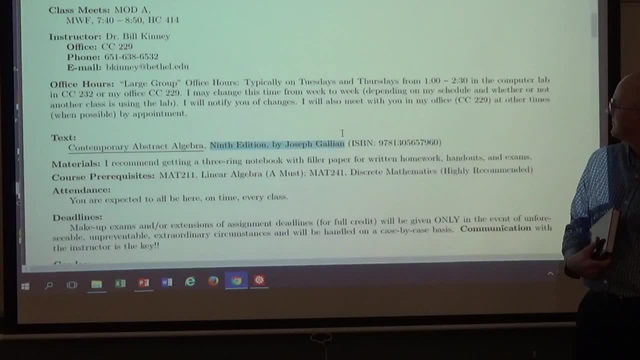 Not too far away from us here in Twin Cities, Minnesota. Here it is. 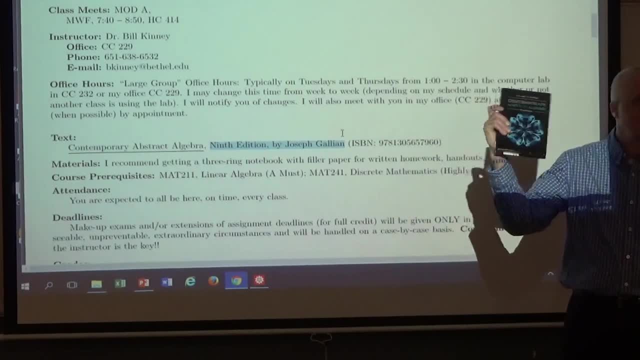 Maybe you can find a cheaper copy online. I don't know. This hardcover copy. If it's new at least it might be kind of expensive. Could be some used copies out there. 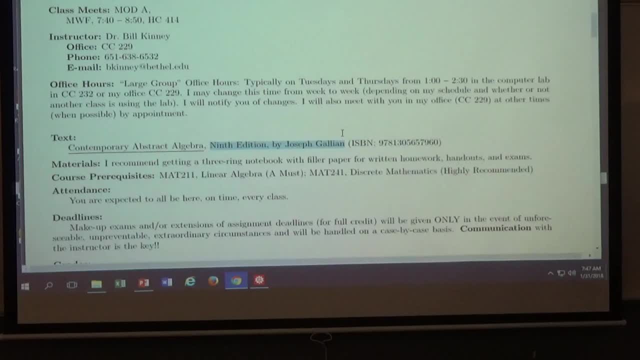 You're certainly welcome to do those things. But you do want to make sure that it's the 9th edition and hopefully has the exact same homework problems. If that's not the case, then you would want to make sure that you get that fixed right away as soon as you can. 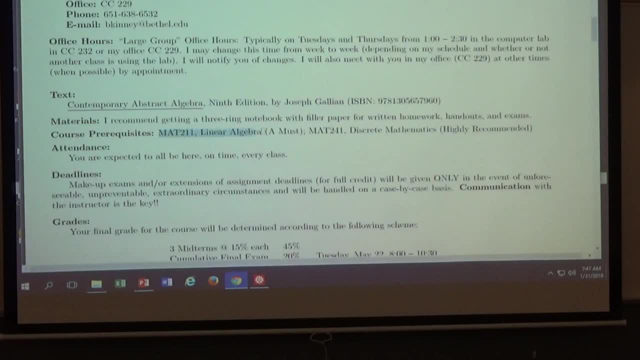 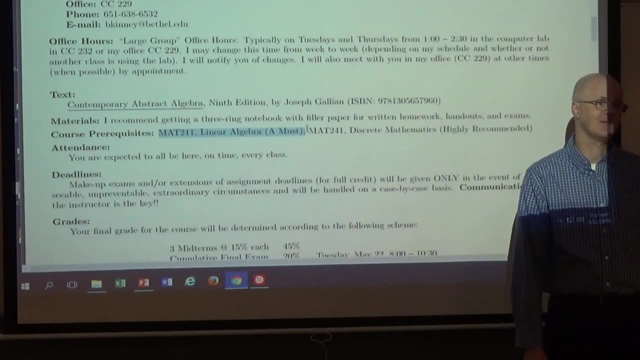 Good requisites. Linear algebra is a must. If there's any class this class is most like, it's most like linear algebra. Especially the stuff about vector spaces. That's what this class is most like. It is abstract in nature. 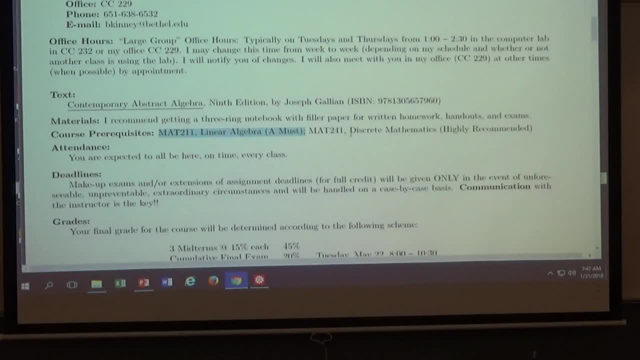 Discrete math. Well, you probably all have it anyway. I suppose it's possible one or two of you might not. It's highly recommended. Maybe not officially a must. Though maybe with the prerequisites it turns out you have to take it before this class anyway. I don't know for sure. I'd have to look that up. It's somewhat similar to discrete math in that it is discrete to a large extent instead of continuous. 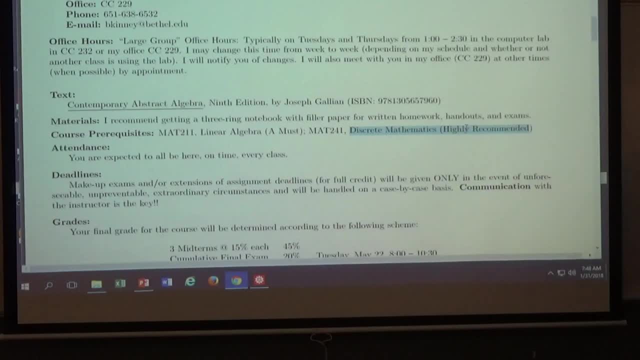 And we do do a lot of proofs as we do in discrete math. 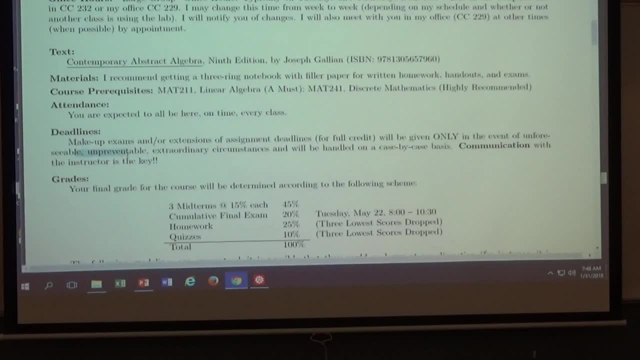 Deadlines. Oh, you're expected to be here. Deadlines are only in extraordinary circumstances. You get an extension. You get an extension on something. So make sure you communicate with me. If you live off campus, you know, if you have a day where there's some snow, you should plan ahead. But, you know, certainly if you do get stuck in a big traffic jam that doesn't move, that can be a situation for an extension. 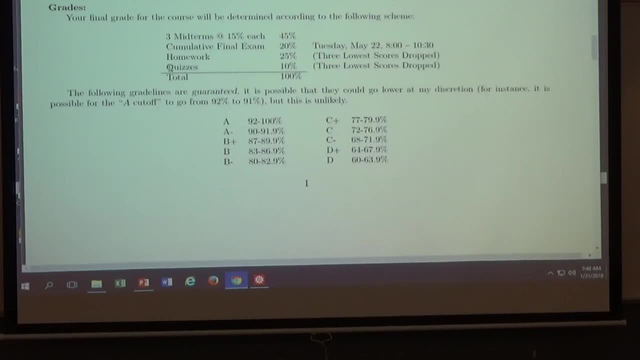 I'll let you look over the grades distribution here. Again, we do have quizzes that are going to correspond to 10% of the grade total. I will drop your three lowest quiz scores and your three lowest homework scores. The other thing to notice is that the final exam is Tuesday, May 22nd from 8 to 10.30. It will be in this room. We do have a late final exam week this year, maybe even later than the ordinary. Although I think it was maybe late last year, too. Nothing I can do about that either. Nothing I can do about the early time. 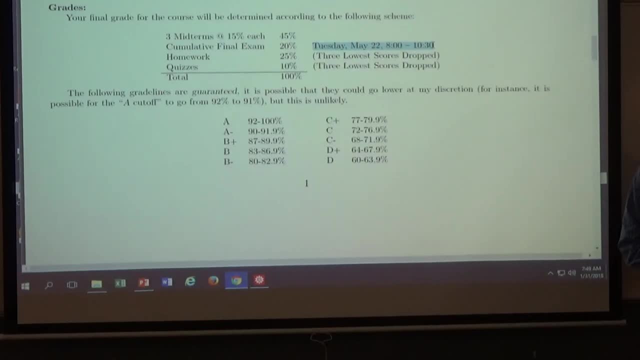 Nothing I can do about the late final exam week. It's partially because we have so many breaks during the semester, okay? We do have, you know, Good Friday off, we have Easter Monday off, we have spring break, we've got advising day, that kind of thing. That's all part of what pushes it back. 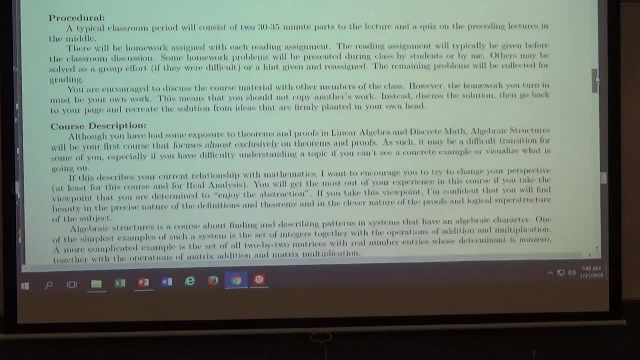 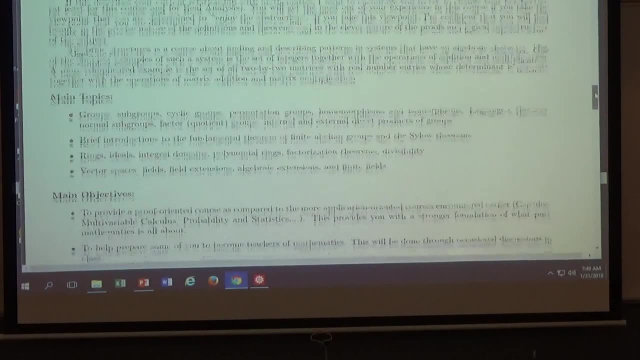 I'm going to let you read about the procedure and course description on your own. You could be quizzed on a few things related to this on Friday. Topics are going to make more sense. Later in the course, looking over these topics, it probably doesn't make much sense. You don't know what these things are referring to. 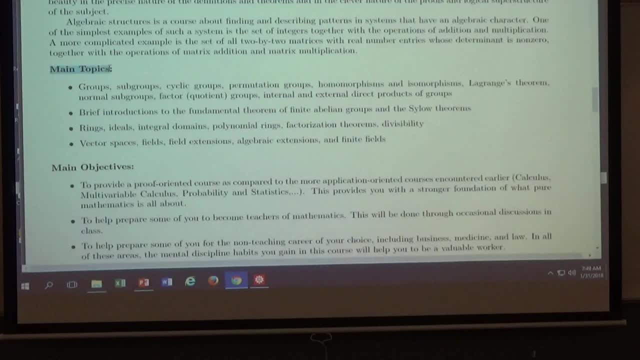 The most important thing about having this topic section is for if you go to grad school, for example, 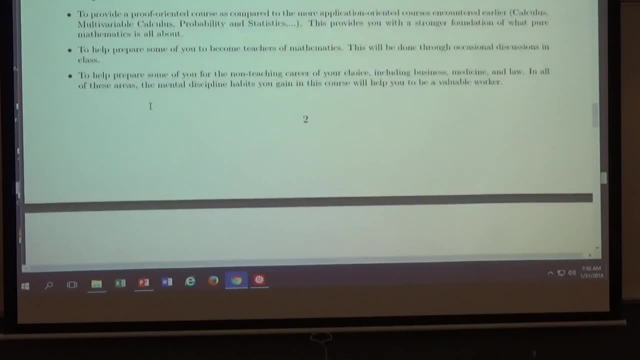 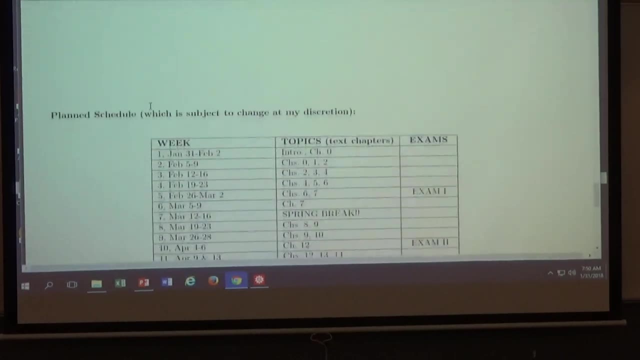 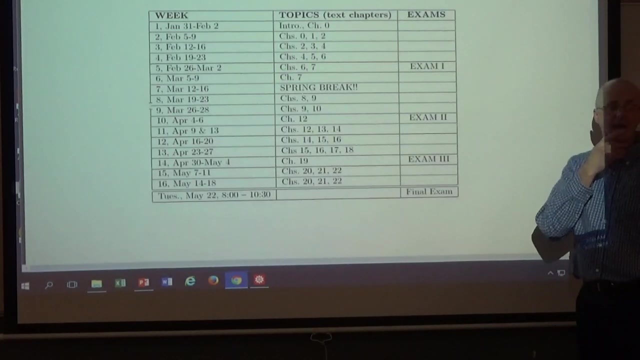 so that they know what topics that we cover. Objectives, accessibility, appeals, learning integrity, all those things you should look over. And this schedule is not super informative as far as topics go, but they do the highlighting. You can look at the exam weeks. I'm not picking exam dates yet, but I've been picking exam weeks. So exam one is going to be February 26th through March 2nd that week. Sometime during that week, either Monday, Wednesday, or Friday. 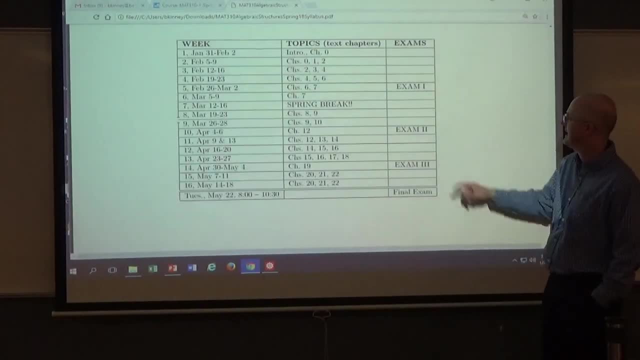 Probably leaning more toward Wednesday, but I'm not guaranteeing that. Exam two is going to be either April 4th or April 6th. Easter, I believe, is the first this year. April 1st. 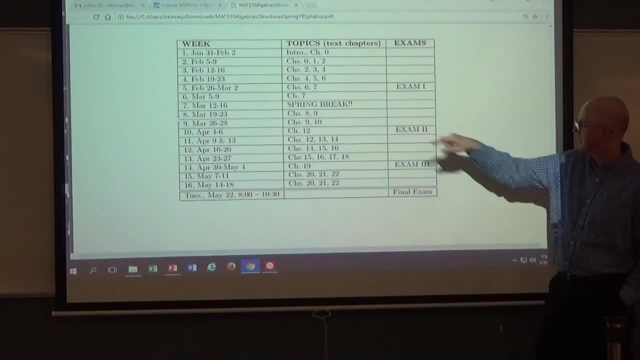 So I believe that's the week after Easter here, so that's either a Wednesday or a Friday. By the way, this is a Monday, this is a Friday. 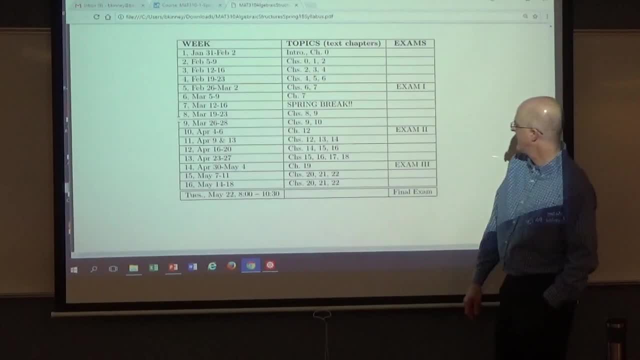 Wednesday, that week, we have the advising day. And then exam three would be the week of April 30th through May 4th. And then your final exam weekend at that time. 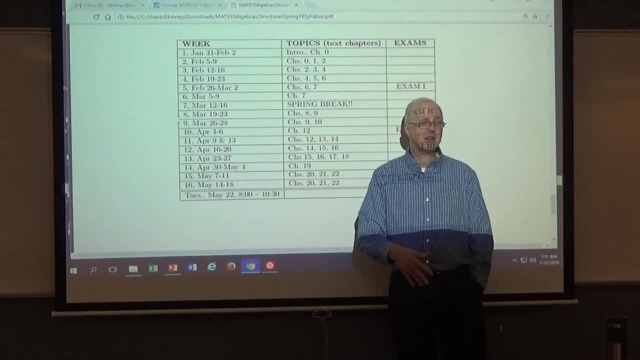 I do give you longer than the official exam time. That goes from 8.15 to 10.15, but I give you 15 minutes early and 15 minutes later. Not that I'll necessarily make it longer, 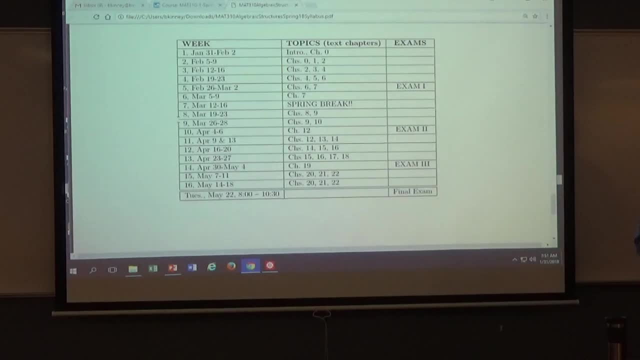 but just in case you want more time. I give you a little bit more time for that. 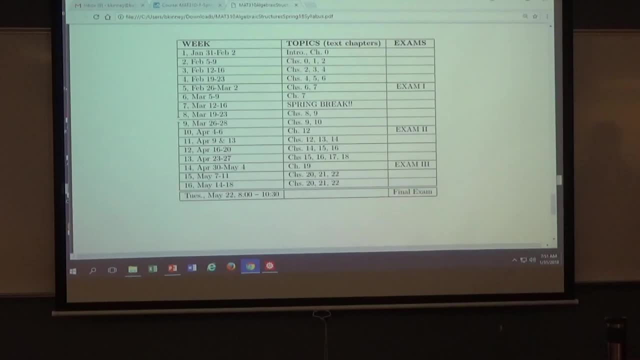 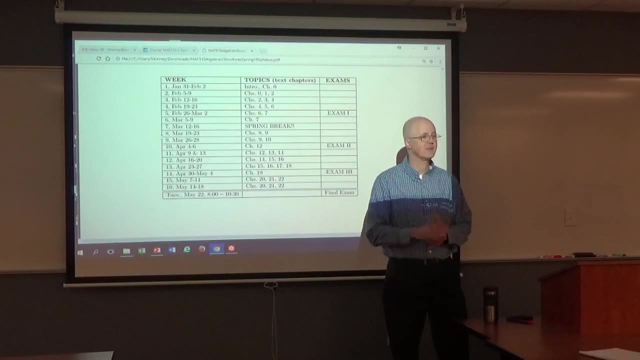 Do you have any questions? Even though we are videotaping this class, I want you to feel free to ask questions. If you've got a question about something, probably somebody in the future has got a question about something. So please go ahead and raise your hand. 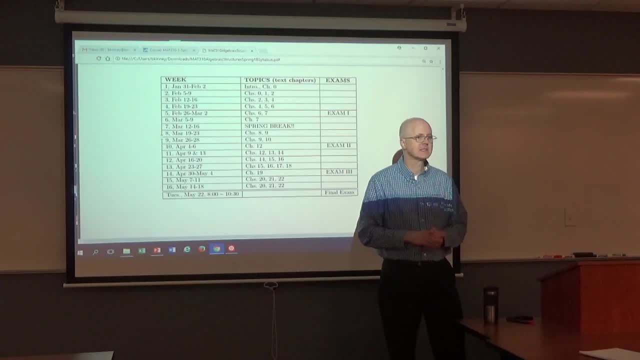 And if for some reason I'm not seeing you, maybe even go ahead and speak up. Okay? 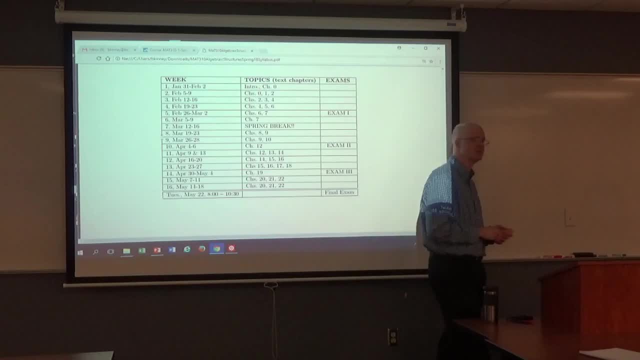 I do want this to be a class where you can feel free to ask questions, even though I'm doing it in basically a lecture format. No questions so far? 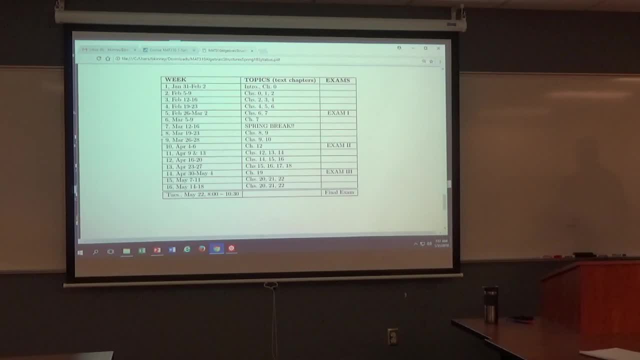 I'm just wondering about the edition of the book. If you have the eighth edition but can look at the homework problems from the ninth edition, do they cover the same things? The topic should be pretty much the same, yeah. 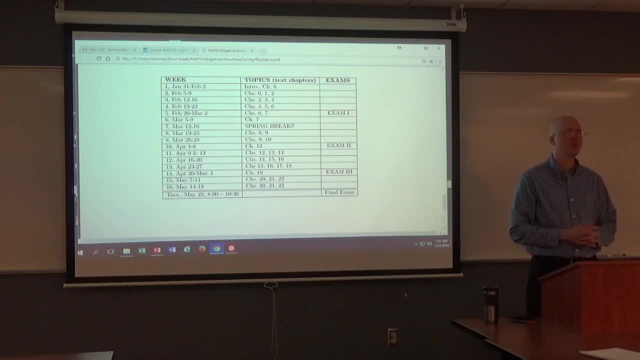 So the problems could differ. The references to further reading at the ends of chapters could be different. But probably the basic reading is pretty much the same. Okay? So you can look quickly to see if you see any big differences. Okay? But yeah, you do want to make sure the problems are the same. 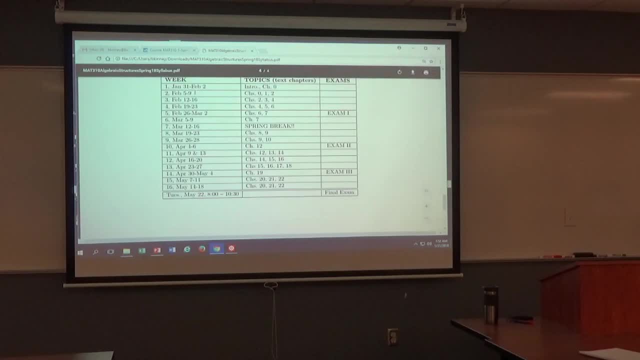 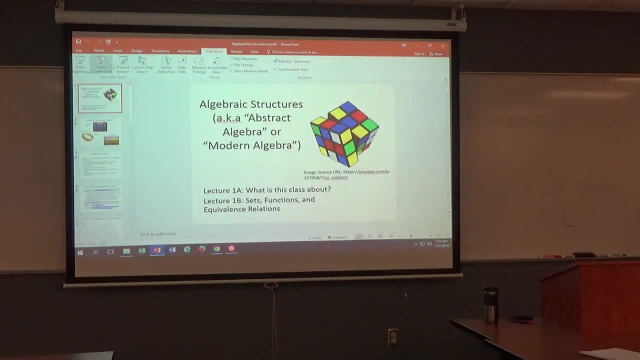 And borrow the problems from somebody else if you want to stay with the eighth edition. 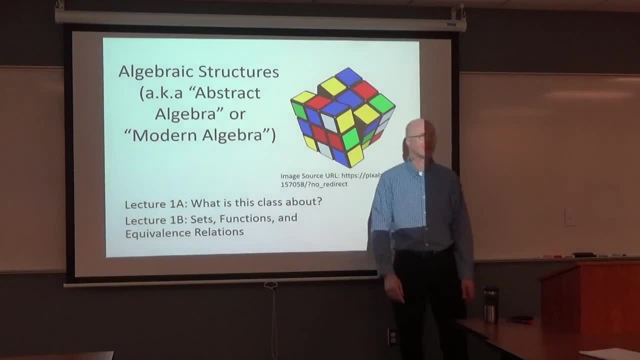 What is this class about? What is this class about? 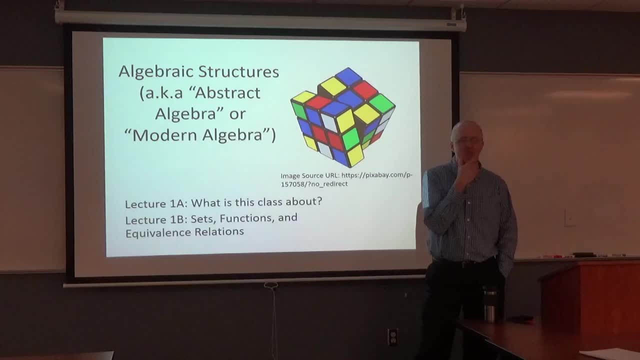 Let's see, how do I remember when I was your age? Well, when I first experienced hearing about this class, it was the year before I was going to take the class, I was taking differential equations. 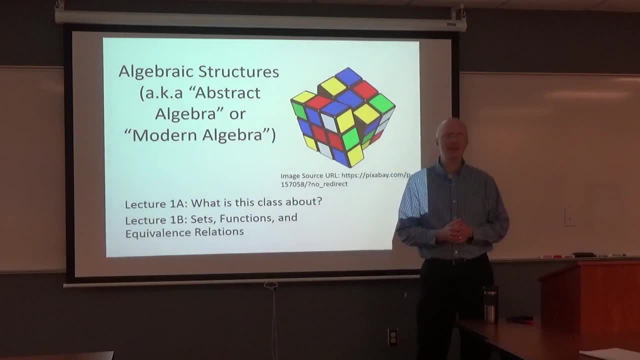 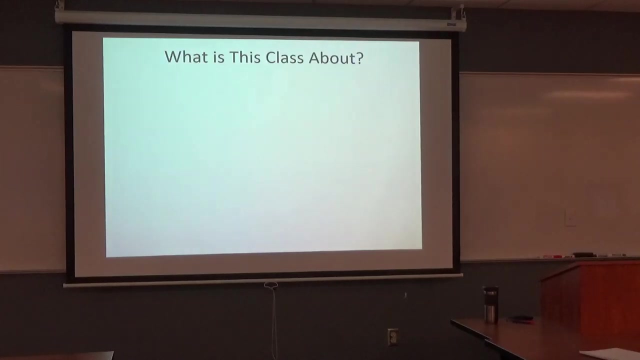 And I was doing pretty well in differential equations. I was talking to the TA in the course. And the TA said, oh, yeah, I'm in this really tough course called algebraic structures. I'm like, well, what is that about? What is algebraic structures about? And well, here's what she said. She said, first, groups, an image like this came up in my mind. 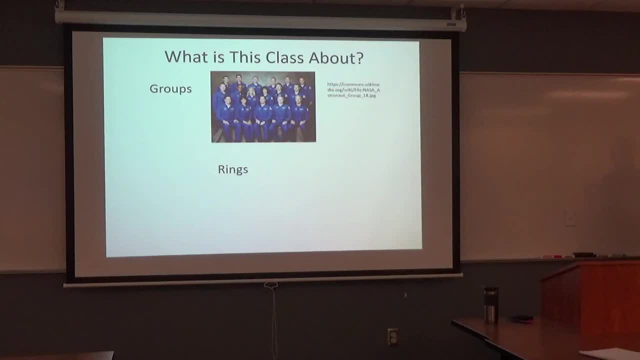 Rings. And well, I'm a Lord of the Rings fan. 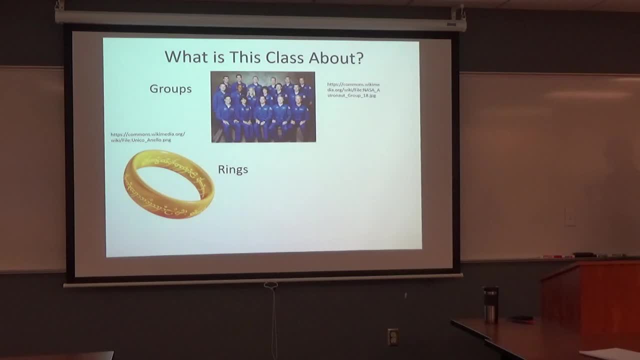 This image came up in my mind. And fields. Of course, that kind of image came up in my mind. Groups, rings, and fields. Okay, so I literally was thinking it must be related to these things. I was, okay? I was very naive. 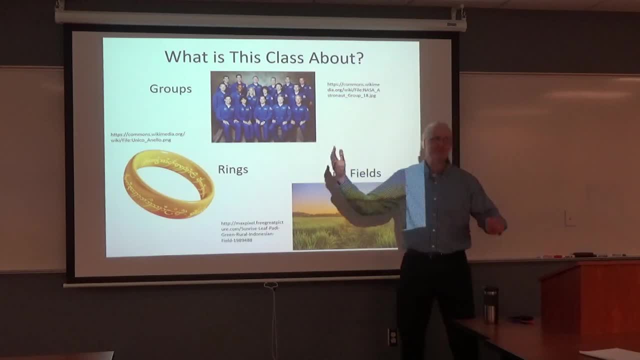 Of course, I thought you could make them mathematical. I thought with the groups, maybe you talked about group dynamics or something, 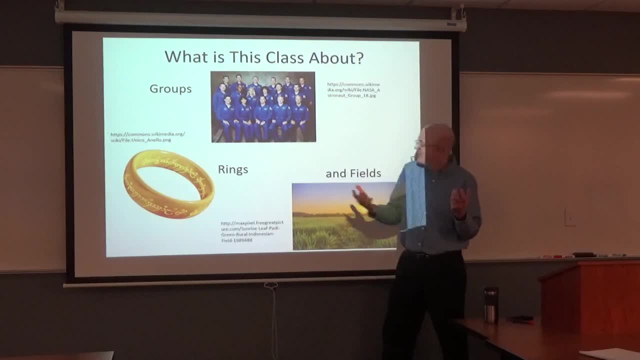 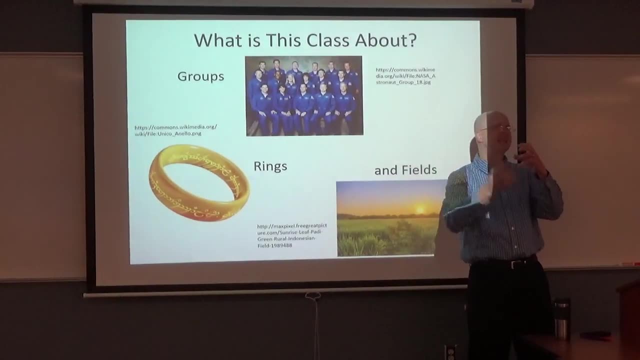 the mathematical theory of group dynamics. With rings, you know, of course, I knew it wouldn't be the one ring. But I was thinking, okay, maybe there's rings in space, and we're studying these rings somehow. And fields, I don't know. 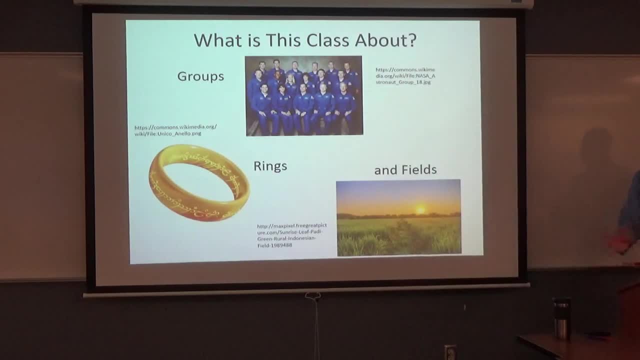 Maybe you're studying how fields can go up and down. But that's not what groups, rings, and fields mean in algebraic structures. 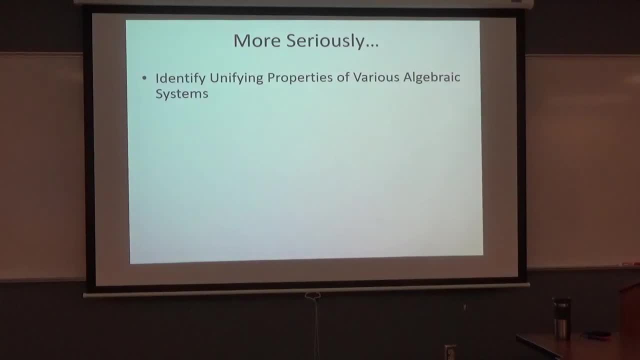 More seriously, it's more like vector spaces in linear algebra. Okay? 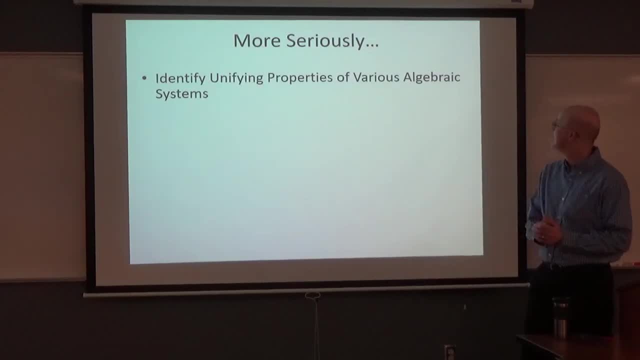 We're going to be identifying unifying properties of various algebraic systems. 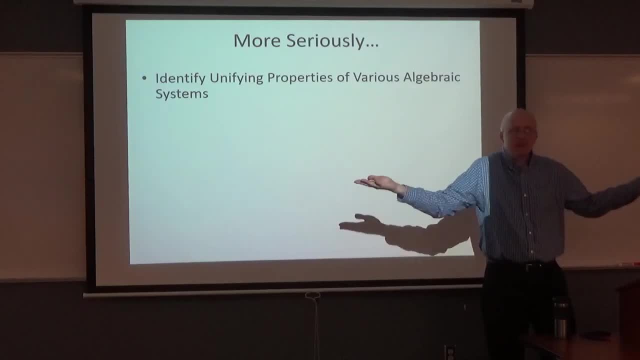 The names groups, rings, and fields are just the names we give to these things. Why? I don't know. 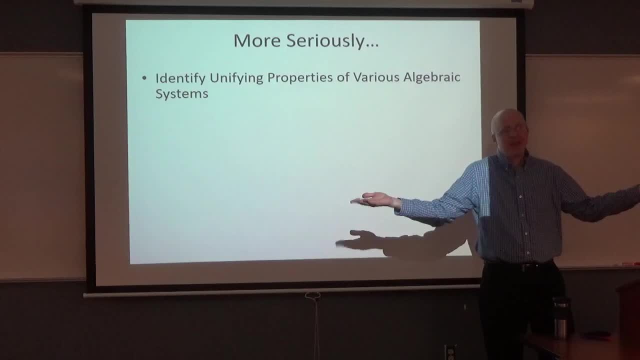 I guess it would be a good historical study to try to look back in time to understand why people gave the names that they did, groups, rings, and fields. 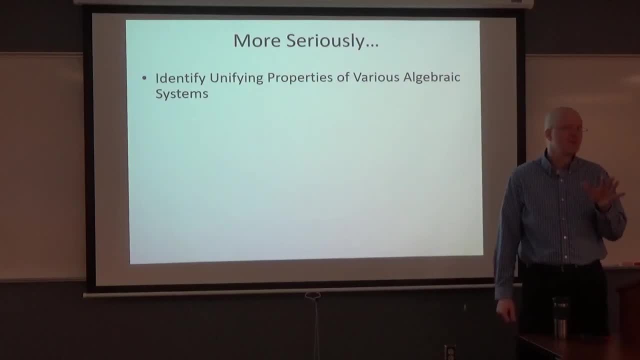 Actually, I think groups makes the most sense. 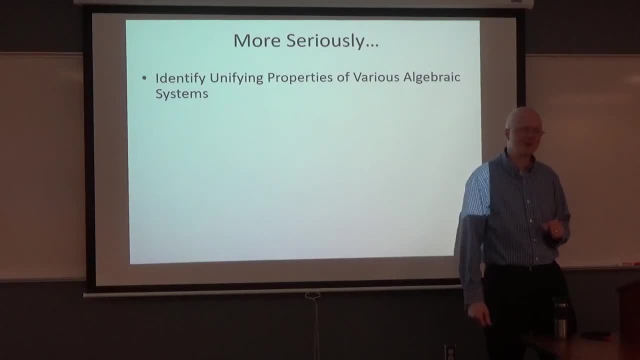 I mean, when we get into it. Rings and fields, it's a little hard to understand why they chose those names. We're looking for those unifying properties. We want to develop mathematical slash algebraic structures, sometimes called axiomatic systems, based on these properties. What kind of properties am I talking about? Let's actually ask you. 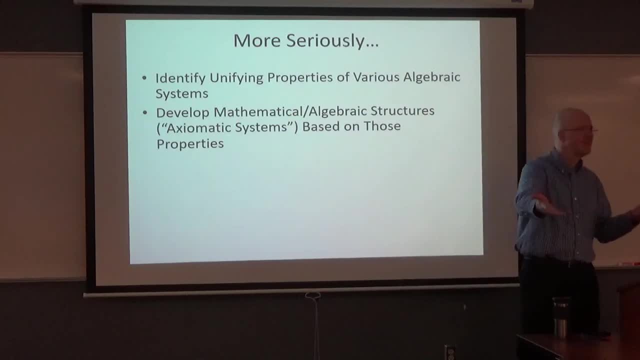 What do you think I'm talking about? Do you have any idea? What kind of abstract properties? They have names, and you've probably heard them before. Do you think you know what I'm talking about? You can think back to vector spaces. What are some of the names and properties of vector spaces? Orthogonality. Orthogonality, that is a property 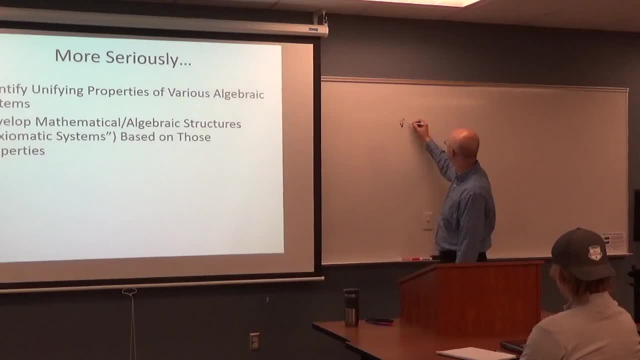 that vectors can have. What about this property? 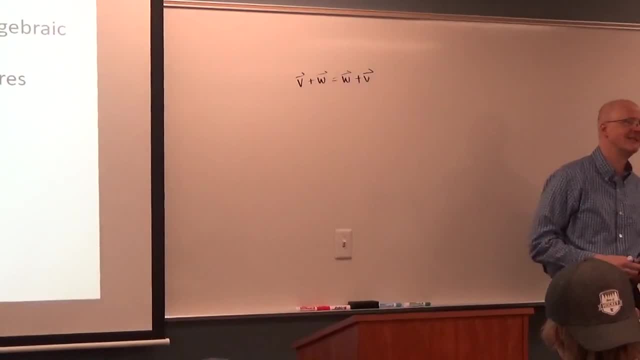 What's that called? Commutativity. 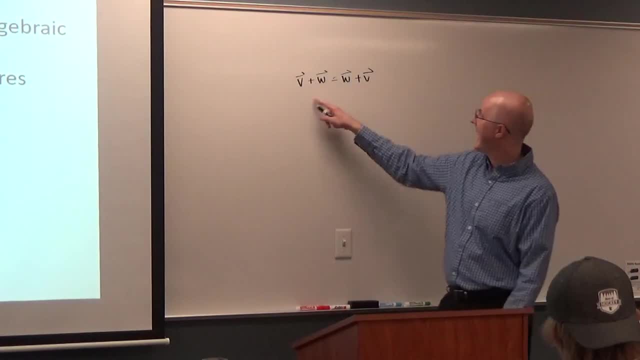 Commutativity. Commutative property. You can add in either order. The V and the W can commute back and forth. 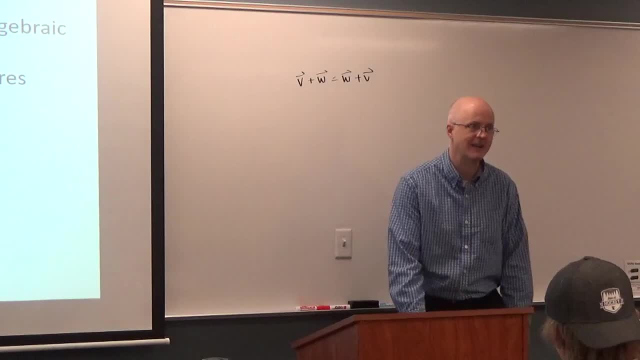 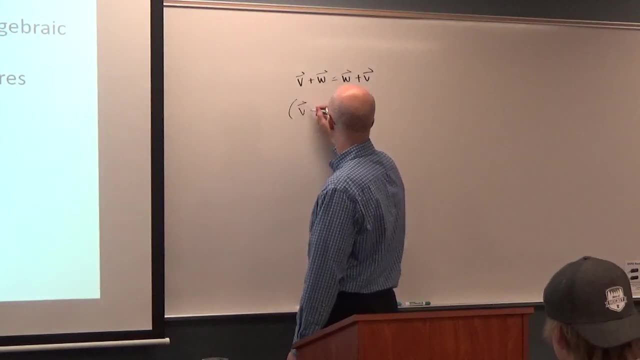 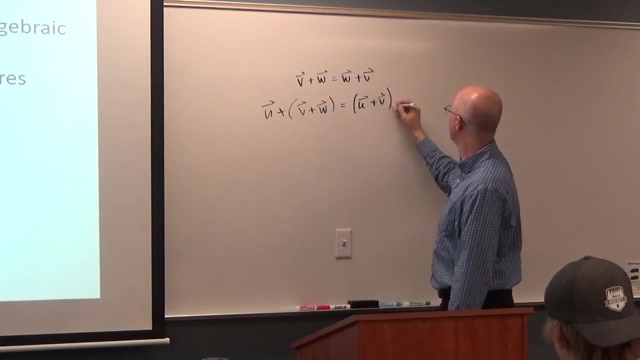 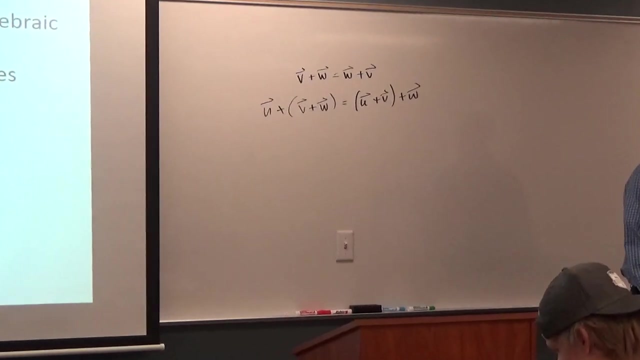 It doesn't matter. You get the same thing. There's a reason for that name. Commutative. Commuting back and forth. What about this property? What would you call that property? Associative property. Associative property. 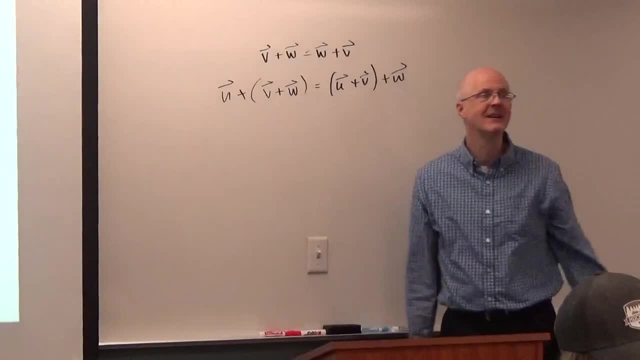 There's a reason for that. You're associating, and it doesn't matter how you associate. 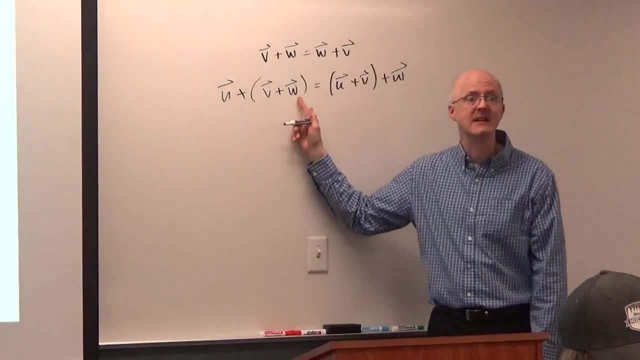 When you use the parentheses this way, of course it means add V and W first before you add on U. When you write the parentheses this way, you add U and V first before adding on W, and it doesn't matter which order you do it in. That's the associative property. That's what I'm talking about. 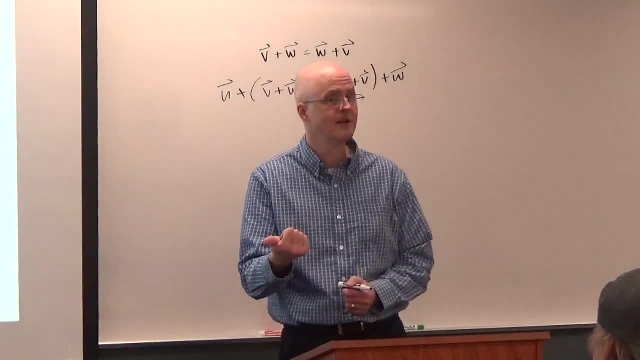 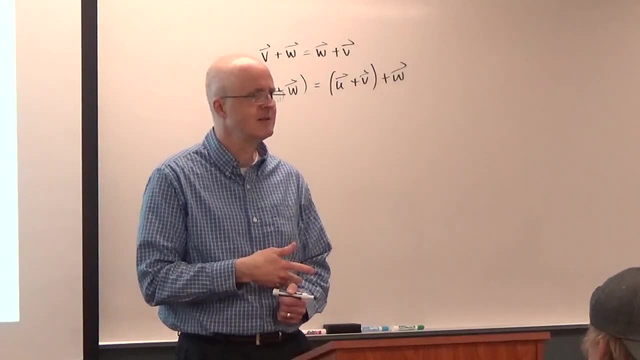 There's also the distributive property. The existence of the zero vector, which has a special property that you add it to any vector, you get that vector back. 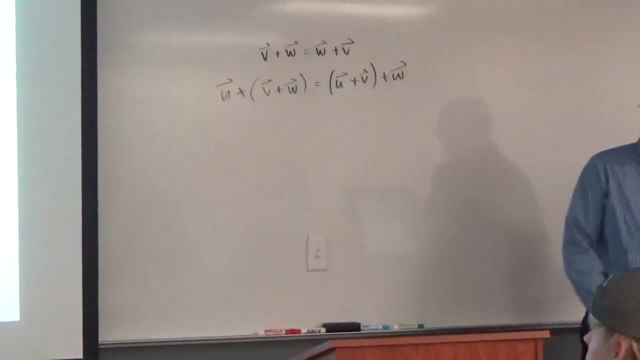 That's what I'm talking about when I talk about unifying properties. 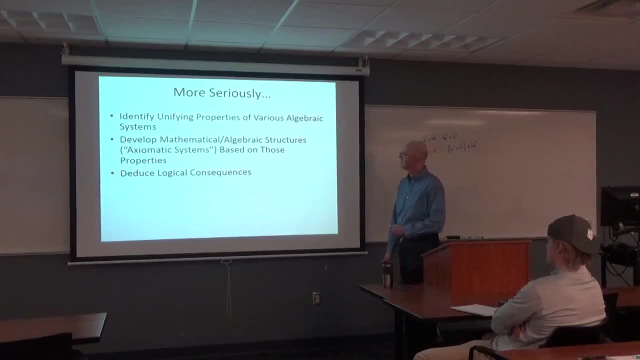 We want to deduce logical consequences. Use your deductive thinking skills to ultimately understand and prove things 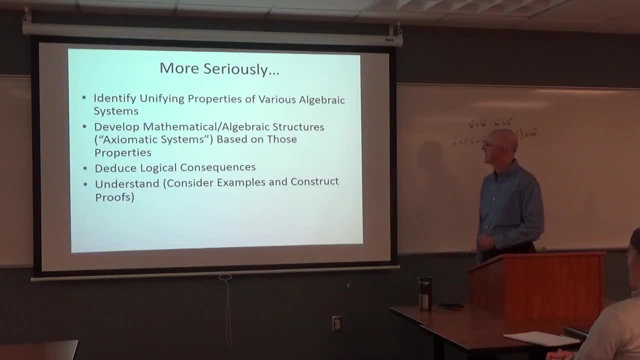 that are not logical. Considering examples and constructing proofs are our main tools for understanding what's going on. 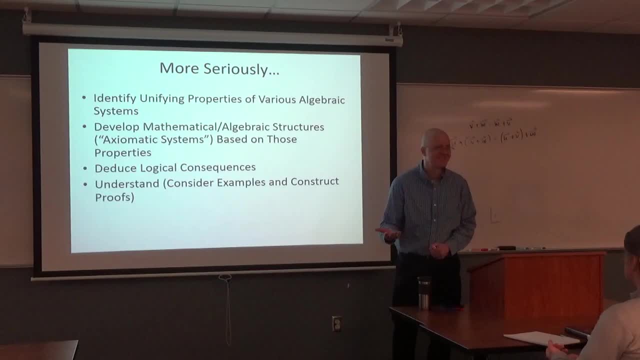 You can learn things as you do proofs. Proofs are not just exercises to do just because the teacher says so and you get graded on them. 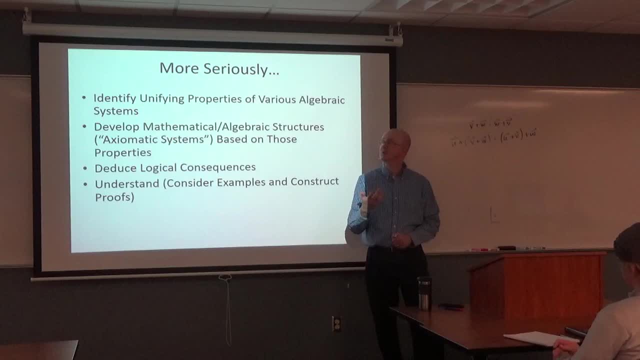 You can actually learn things. That's how you learn the most, in fact, about the subject is by doing the proofs and considering examples. 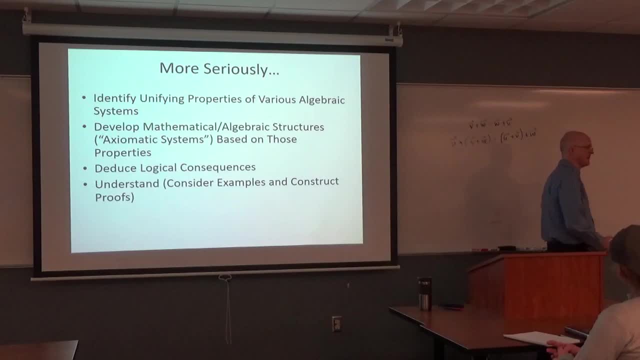 Examples definitely are a necessary thing for learning, for most people. And then apply them. Make use of the theory for various problems. 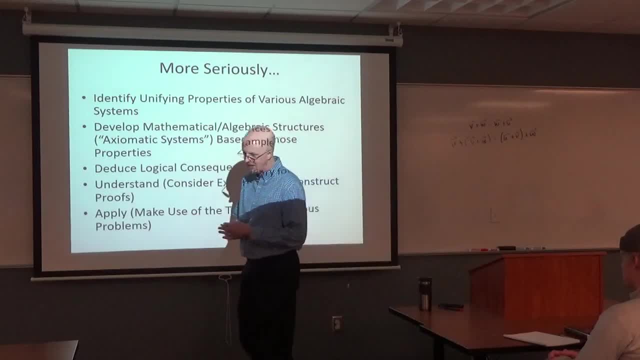 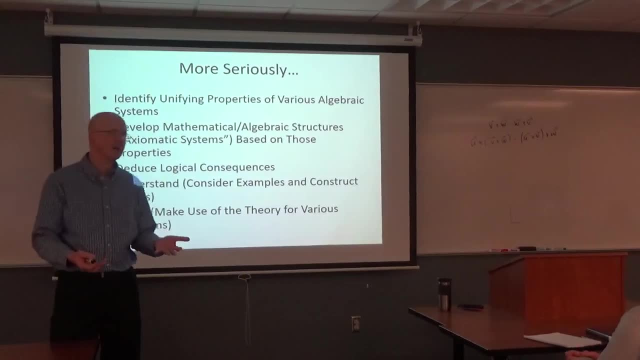 Now, when you say apply in math, I know because I was this way, I was thinking always in terms of, okay, can I apply this in, say, the business world, or can I apply this in understanding the world, science, engineering, that kind of thing. 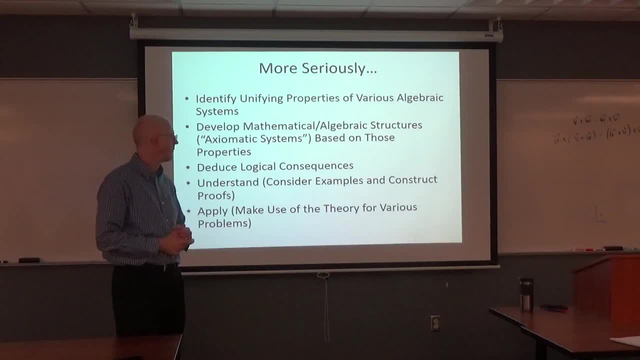 And that certainly is, a reasonable thing to think about with application. In this class, it's not going to be so much that way. When we apply the ideas in this class, it's really to help us understand things deeper. It is, I suppose, our main application you could think of that we do. The book has got plenty of other applications, but the main application that we do is probably to something that sounds kind of mundane, factoring polynomials. 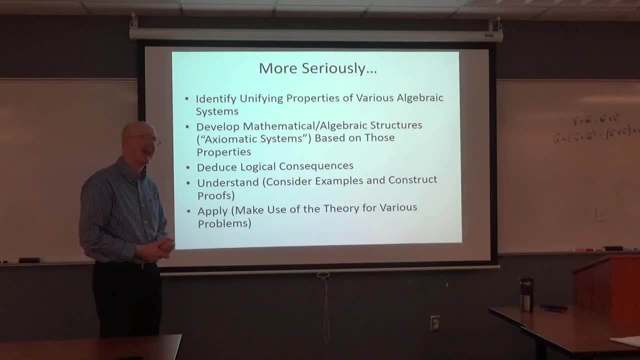 Okay, later on in the course, long about April or so, we'll be doing a lot of theory that will help us factor polynomials better than you've ever factored before. So that might sound like kind of a mundane application, but it is an application. Factoring does have its uses. Helping you find roots through polynomials is a useful thing in general. 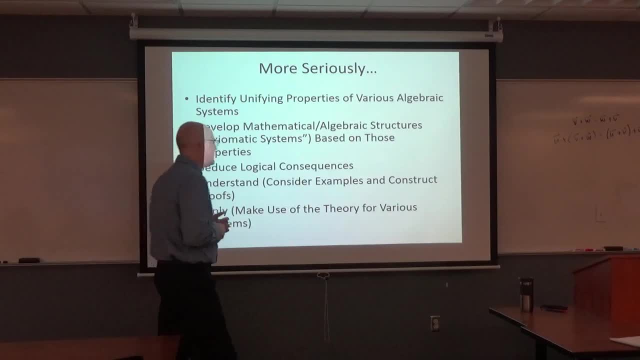 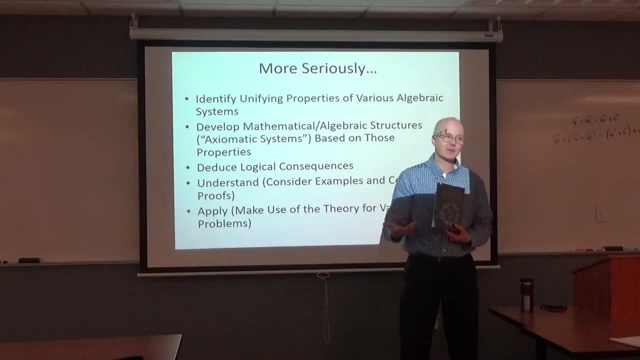 But that will be our main application. The book, however, has got plenty of real life applications that are alluded to. And if you've skimmed over chapter zero, you should have seen something about some of those applications. 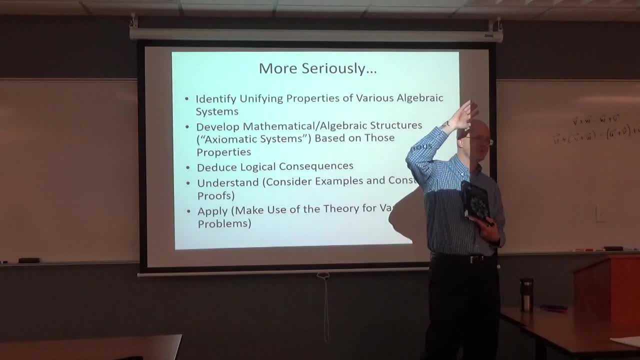 Anybody want to volunteer what those were? Did you skim over chapter zero? Related to something on the back of books. ISBN codes. Okay. 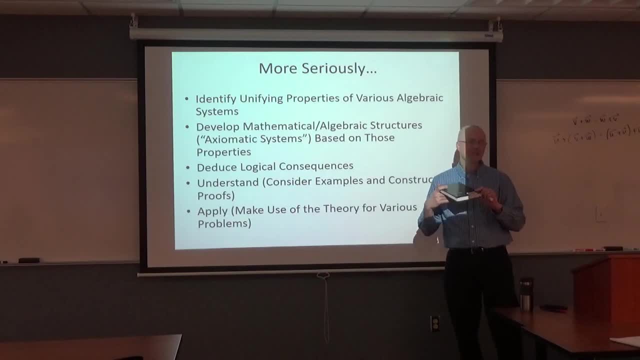 Now, we usually just scan ISBN codes these days. But back when they were first introduced, sometimes when you were buying things, people actually had to type them in. But people make mistakes when they type things in. What happens if they make a mistake? The way these codes, the ISBN codes, are set up is in such a way that you can catch mistakes if somebody actually typed them in. 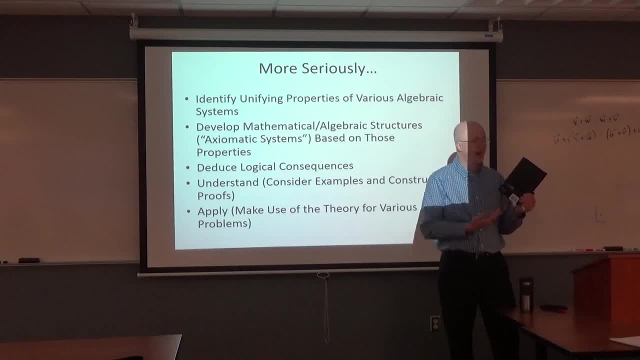 Okay. And it's the number theory of how those are set up that allows the mistakes to be caught. 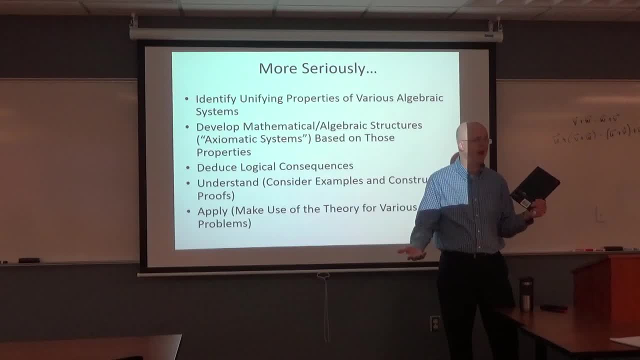 Not necessarily all mistakes, but a lot of common mistakes. Can be caught. Okay. That's one application. That might seem mundane. 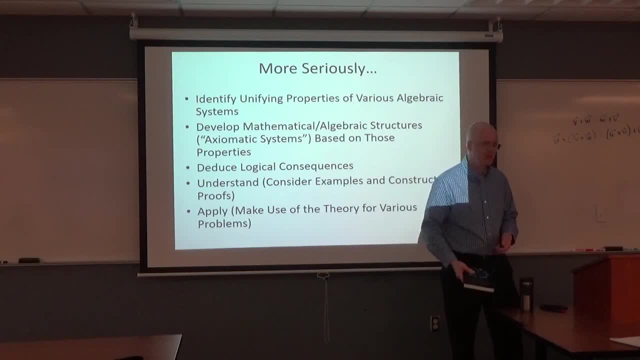 But a related application is to cryptography, which is very, very important. All your Internet transactions need to be secure. They need to have that information scrambled in some way so that somebody doesn't intercept your credit card number, for example. Number theory and related group theory help with the construction. With the construction of cryptographic systems that prevent your identity from being stolen. Okay. 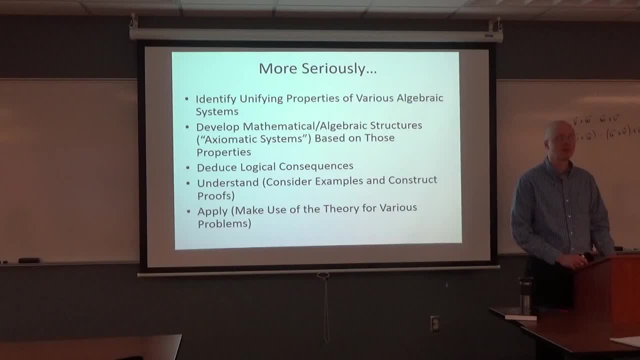 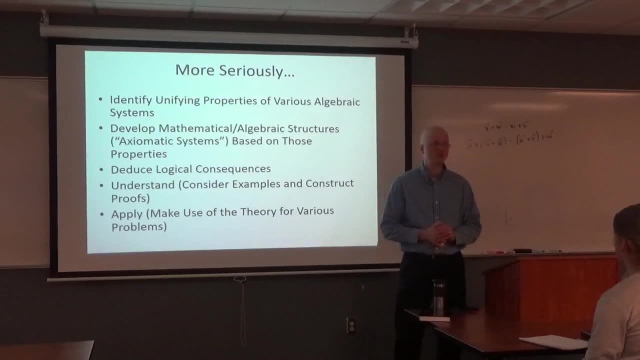 So that's a couple of things that the author highlights. We did in Foundations of Math here in January have a few students who actually did projects related to those things. So those could be future projects for your Foundations of Math if you haven't taken that. Okay. As most of you have not. 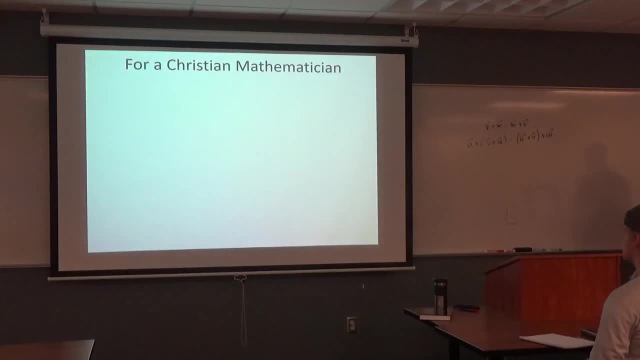 Perhaps next January. For a Christian mathematician, 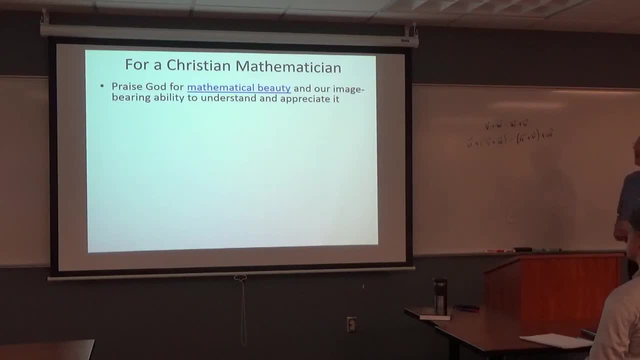 I would say there's more. I want to praise God for mathematical beauty and our image-bearing ability to understand and appreciate it. 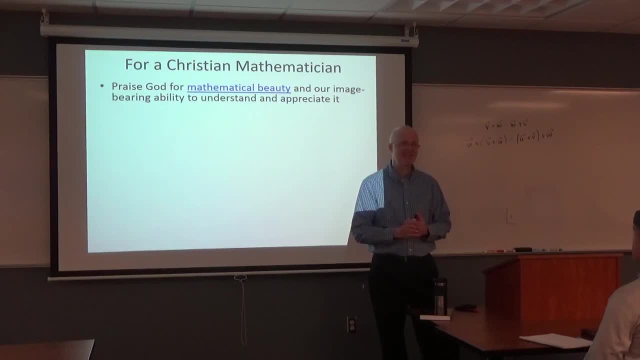 You can appreciate it if you pray about it. Okay. 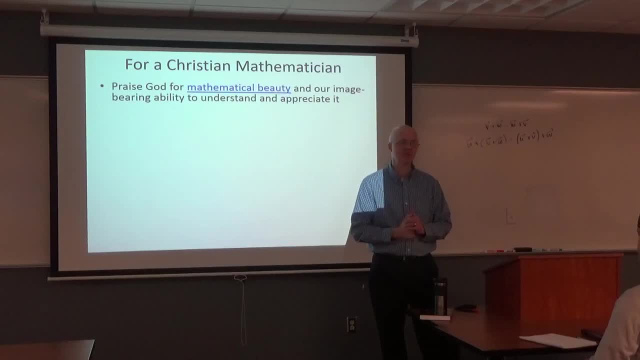 Of course, there's the frustration that we all experience when we're first learning something. 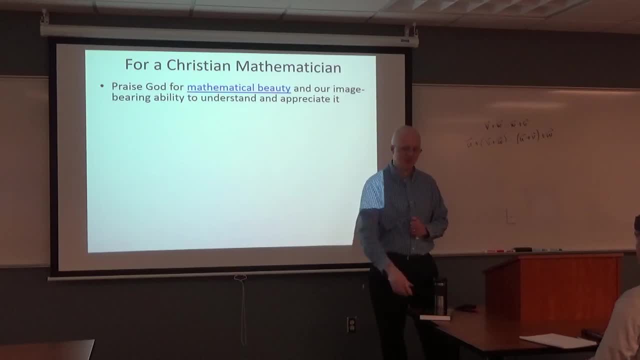 And in frustration, you might want to throw it in the garbage or something, but don't. 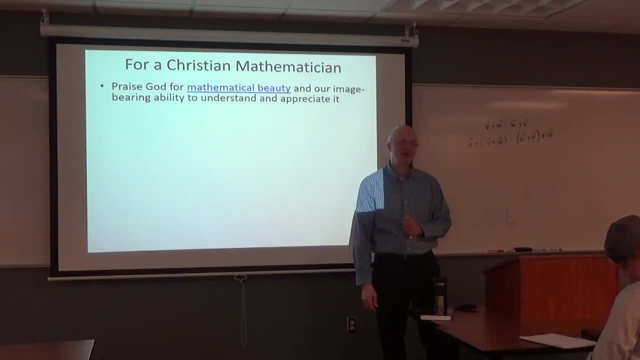 Sometimes this appreciation doesn't happen until after the course is over. Maybe not even until years later, but I hope it does come at some point for you. 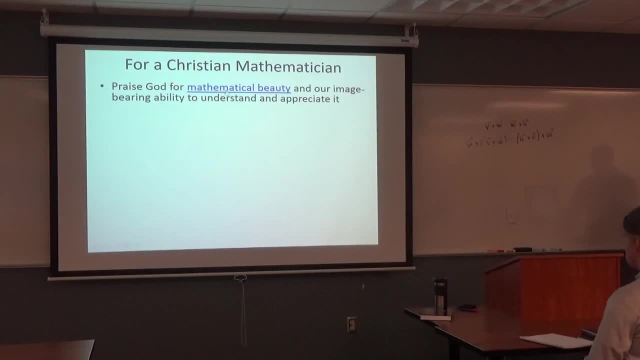 By the way, these blue things here are, there is often a Wikipedia article. 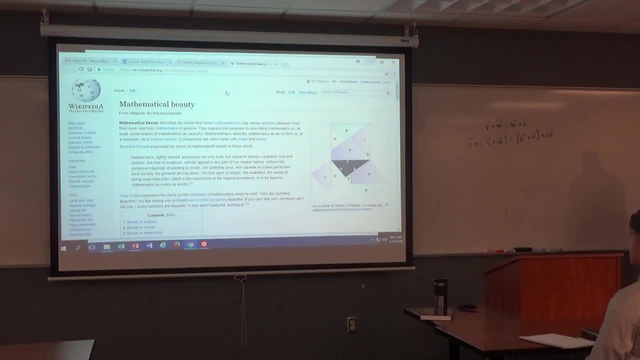 There is a Wikipedia article about mathematical beauty of all things. 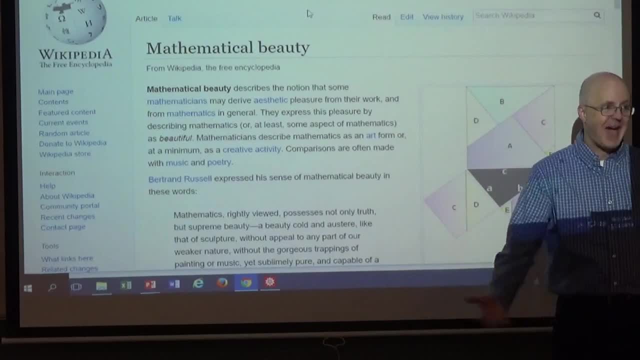 There is an aesthetic nature to math. Patterns. Visualizing things. Can all be part of appreciating mathematical beauty. 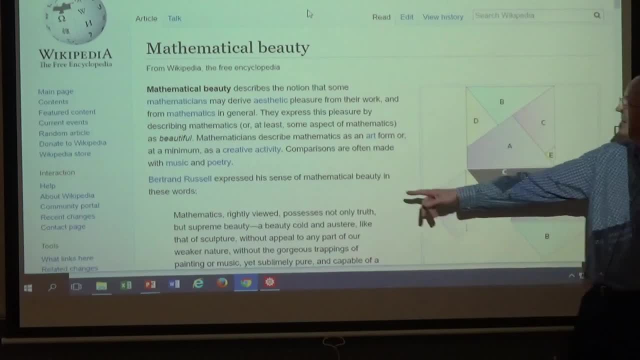 The creative activity. Did you ever think of math as being creative? 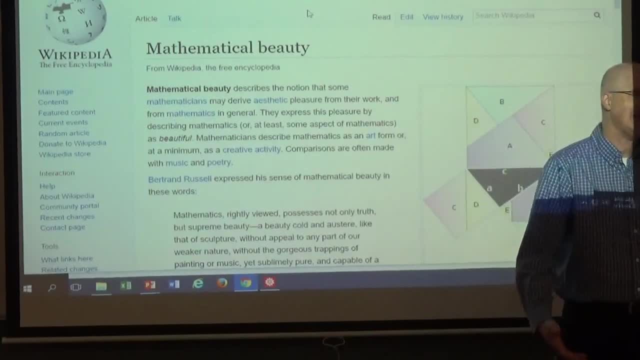 Well, when you're first discovering it or creating it, you are doing a creative activity. 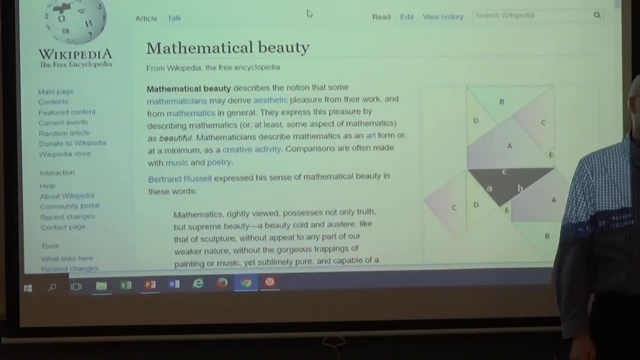 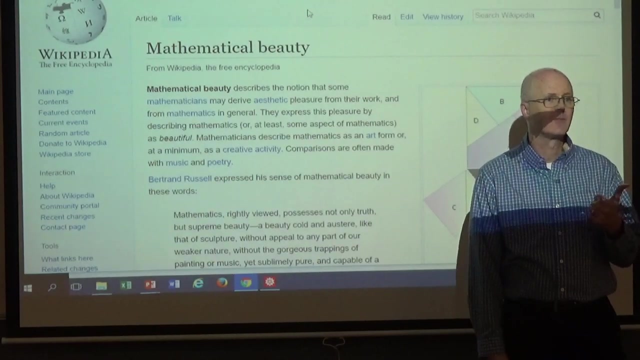 You are trying to figure out something new. Which, by the way, is what PhDs in math have to do. They have to do something new that nobody has ever done before. And significant, too. That could be solving a problem that nobody has ever solved before. Which often does involve using a lot of advanced theory. Could be developing a new technique for something. 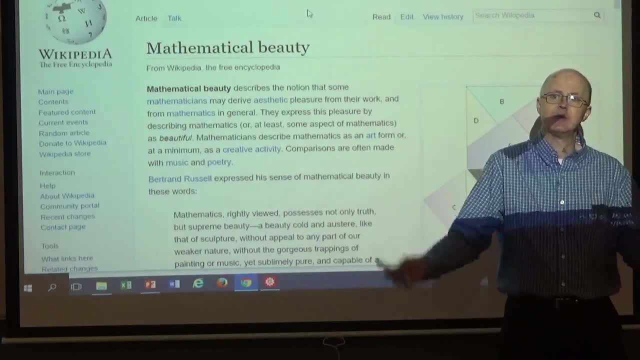 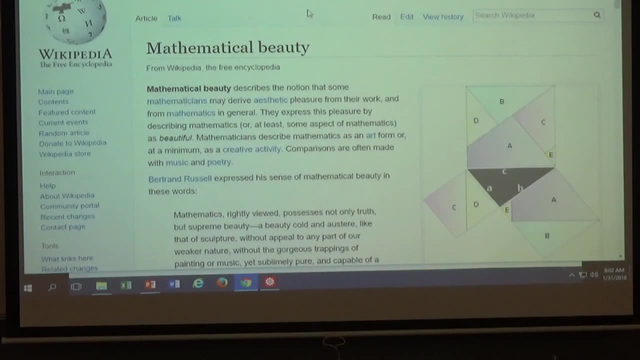 And if you're really ambitious, it could be maybe even trying to completely develop a new theory of math. A new area of math, I should say. That's what PhDs in math have to do, is they have to come up with something new. Which sounds kind of scary, but when you really get into it, if you get into it far enough, it's not as scary as it initially sounds. 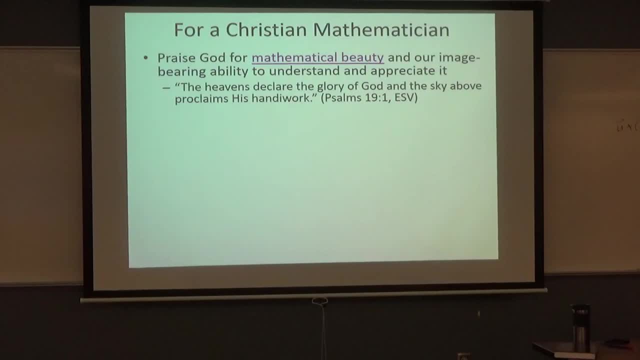 We can praise God for that. The heavens declare the glory of God, and the sky above proclaims His handiwork. Not just the sky above, but also math, I think, too. 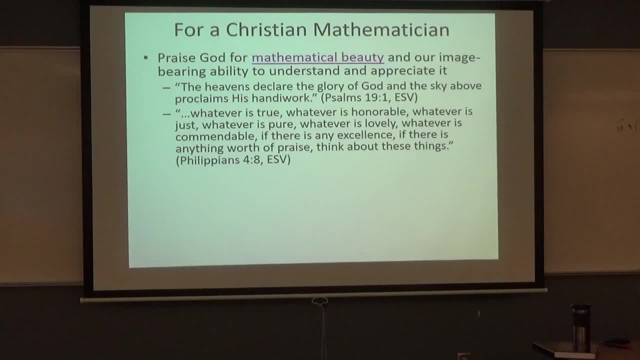 Whatever's true, whatever's honorable, whatever's just, whatever's pure, whatever's lovely, whatever's commendable, if there's any excellence, if there's anything worthy of praise, it should be worthy, not worth. Think about these things. 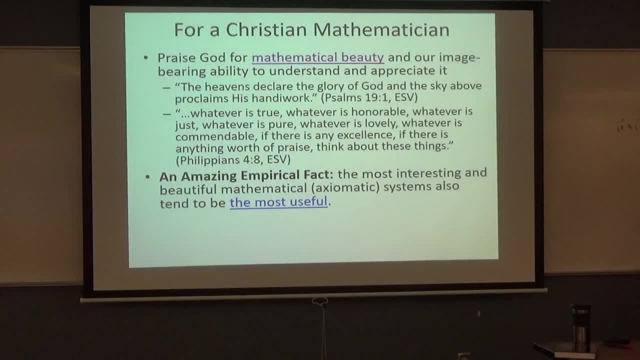 Here's an amazing empirical fact. This is true. By the way, what the word empirical means, based on experience, not based on logic, the most interesting and beautiful mathematical or axiomatic systems also tend to be the most useful. One example is complex analysis involving complex numbers and quantum mechanics. 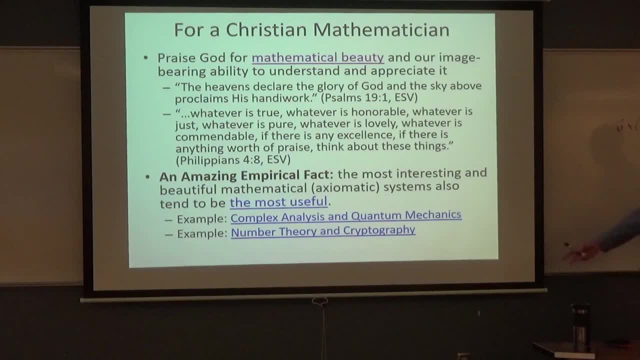 Another example is number theory and cartography, which I already alluded to. 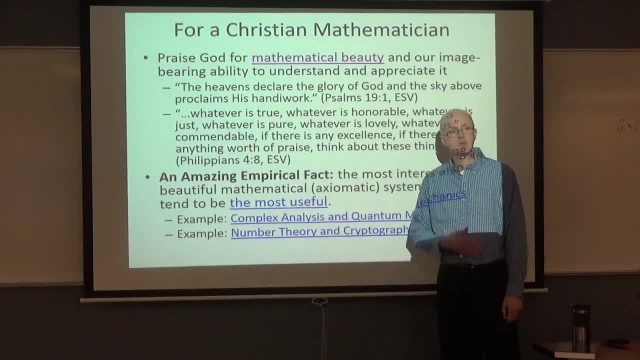 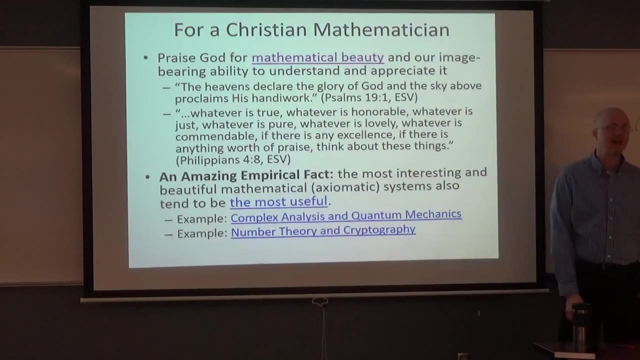 When complex analysis, complex numbers, were first being developed, thought about, people didn't imagine it would have any application, other than the reason they were developing, which was to factor polynomials. But in quantum mechanics, they find application, which is an advanced theory in physics. 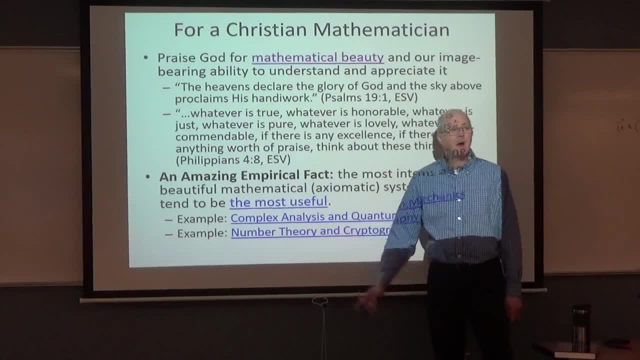 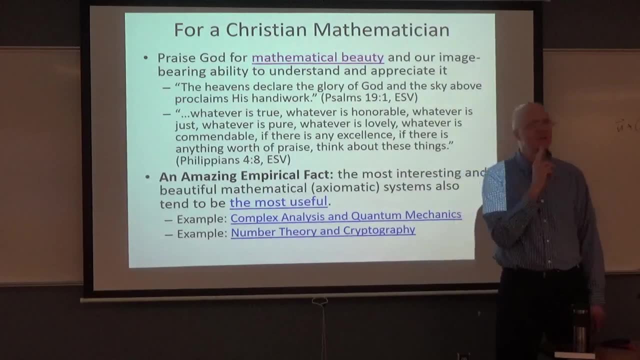 Number theory, long about, even just a hundred years ago, there was a mathematician named G.H. Hardy, I think it was Hardy who said this, maybe it's somebody else, who said, number theory is beautiful, okay, this is definitely a paraphrase, and I especially like it because it's unsullied by applications. Okay, there is a pure mathematician for you. 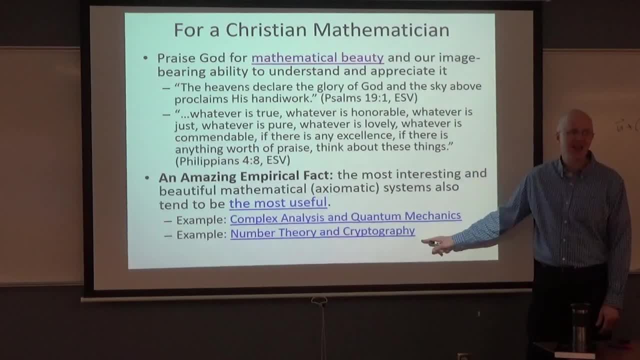 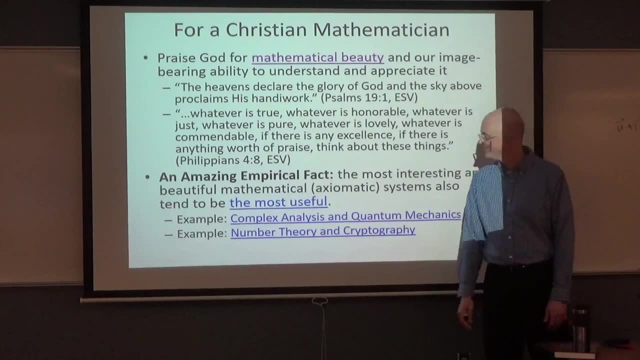 Well, there's plenty of applications now, okay? We wouldn't have our internet transactions going on without cryptography, which comes from number theory. And in particular, one important fact in number theory is that when you multiply two really huge prime numbers, you know, maybe, I don't know, 50 to 100 digits long, you get a really big composite number, and if somebody doesn't know what primes you multiply to get that new composite, they're not going to be able to factor it, even with today's computing technology. 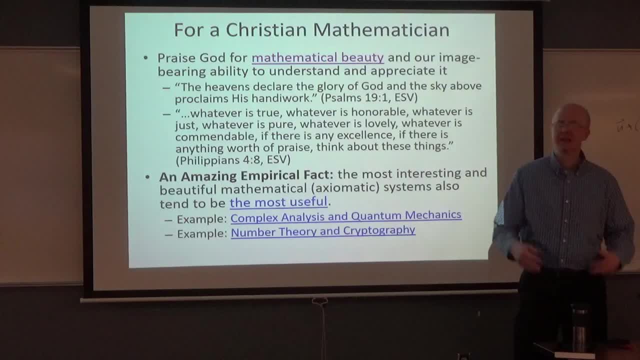 Now, there's some issues about whether quantum computing can lead to the ability to factor those really big numbers, but that's, at least for the moment, part of what makes cryptography work. They're really huge products, and two huge prime numbers can be really hard to factor if you don't already know what those two prime numbers are. 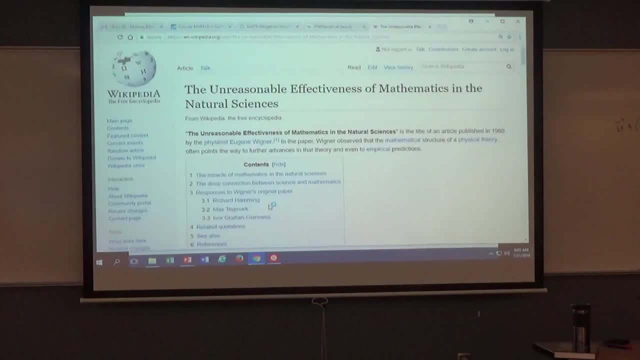 I'm going to go to this link here. Here's a very famous, the title of a very famous article in science. 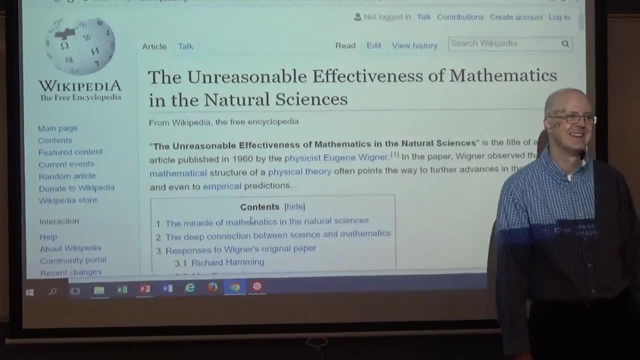 It's called The Unreasonable Effectiveness of Mathematics and the Natural Science. 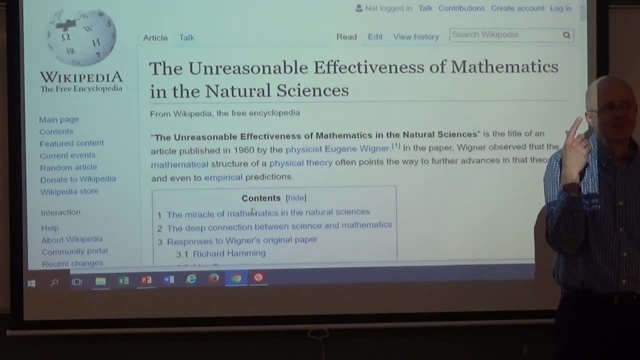 Philosophers wonder, why is math so useful? Why should our thoughts about math necessarily have any relevance beyond counting, say, and adding? 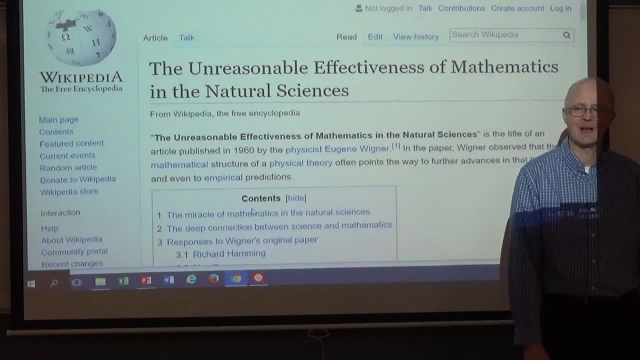 Now, why should complex numbers be useful in quantum mechanics? It's kind of a mystery, okay? But we can appreciate that. 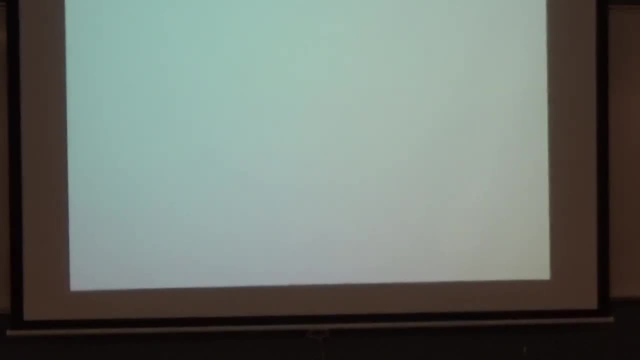 Here's a diagram you're going to appreciate if you go to grad school. 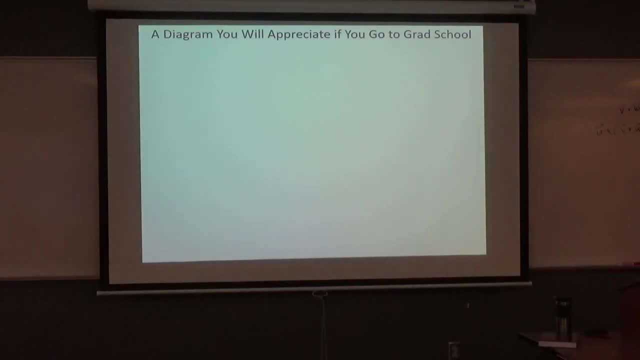 I found this on Wikipedia. I actually also found a mistake on it, so I'm going to highlight the mistake. It's hard to see. 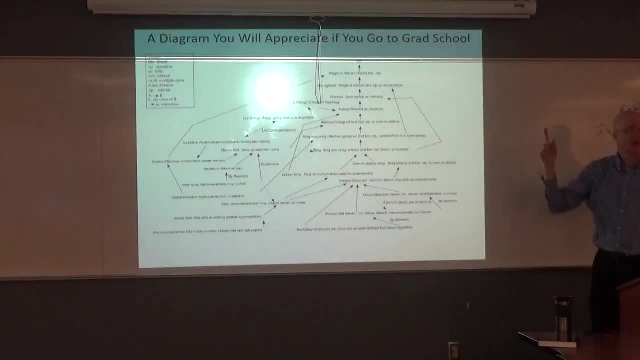 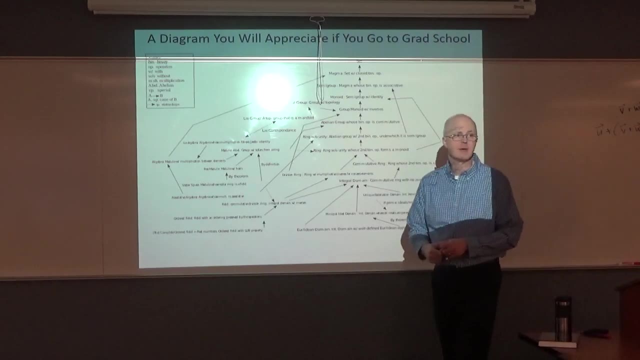 I will be putting these PowerPoints up on Google Drive and share them with you so you can look at them whenever you might need to. 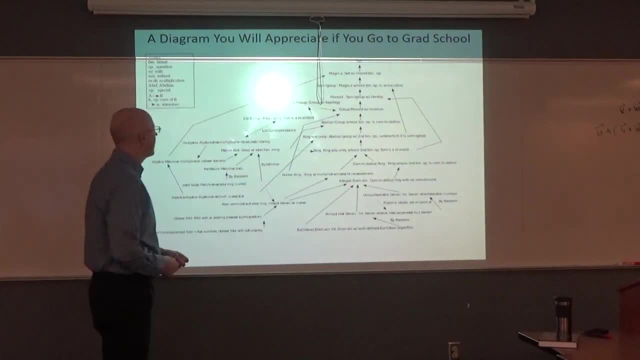 This is a diagram sort of showing a bunch of algebraic structures and the relationships between them. Maybe zoom in on that. 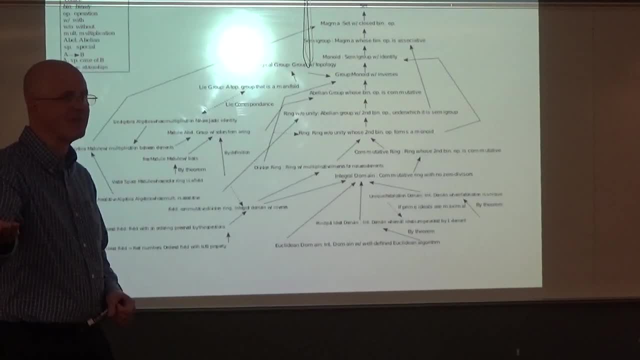 By the way, with videotaping the class, the quizzes, I should say, well, this first quiz I said could have a question or two, 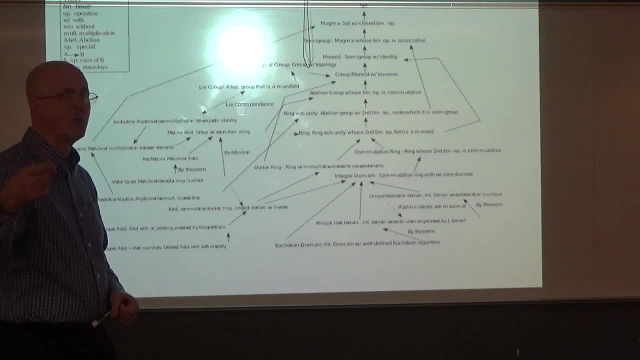 related to the syllabus. The quizzes are mostly supposed to focus on the preceding lectures, and not just the one preceding lecture. 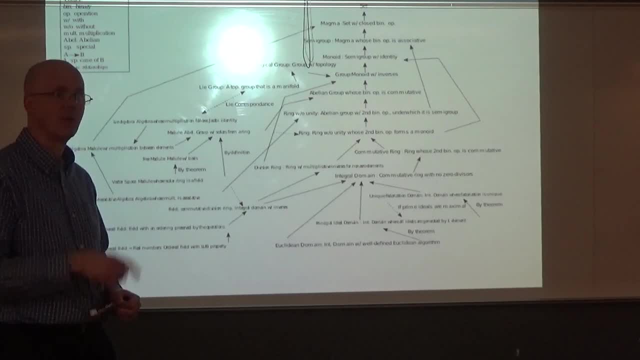 They're going to be cumulative, so you are going to want to take good notes in general once I start doing the math here. 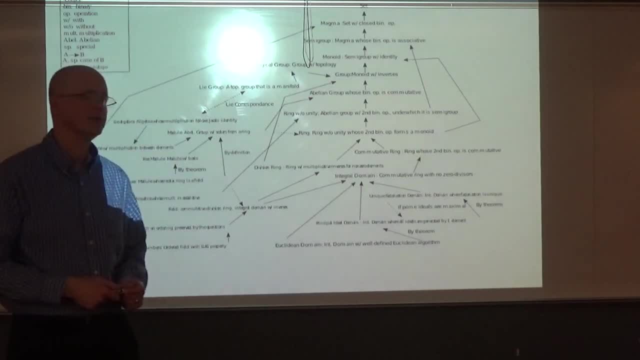 But you can re-watch something in these videos. I'll post them on YouTube if you think it might be helpful to look at them again. 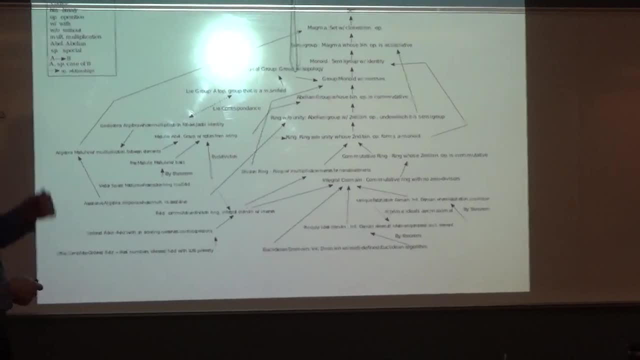 So zoom in. If it's hard for you to see them back, maybe you'll want to quickly watch this part of the video. 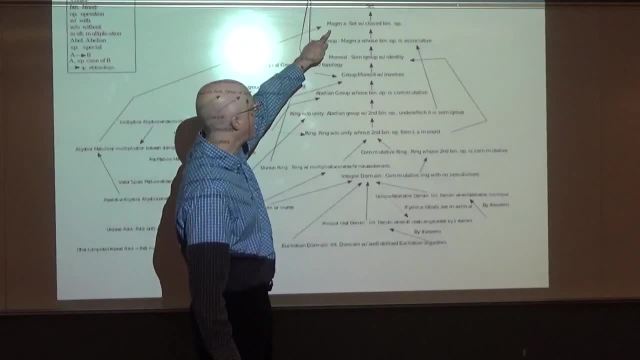 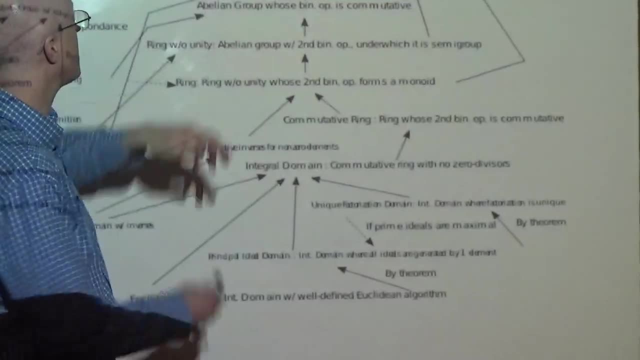 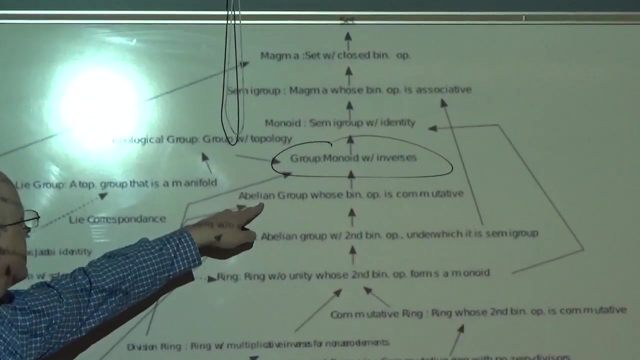 So there's a lot of different algebraic structures in here. A magma. Magma? Weird. Semi-group. Monoid group. I mentioned group. Abelian group. Don't say abelian group. 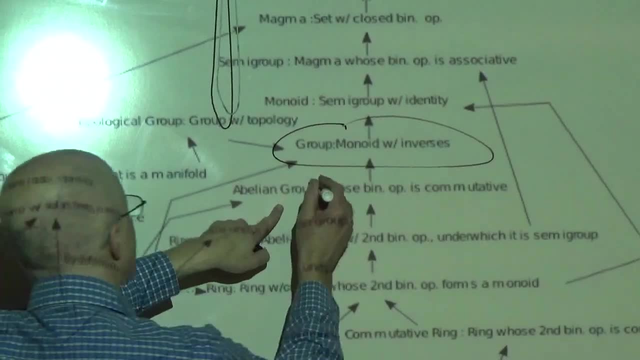 Abelian group is another thing we're going to be focusing on a lot. A ring without unity. Ring without unity. 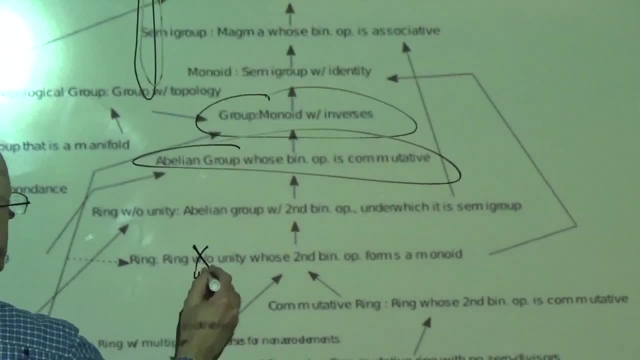 Here's the title. I think they meant ring with unity here, 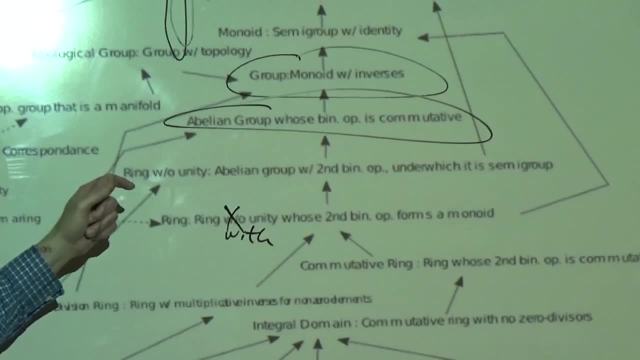 because they already mentioned ring without unity there. What's a unity? Well, it's like the number one, or the identity matrix. 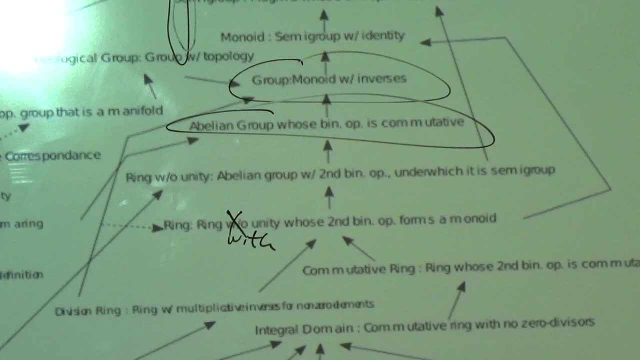 Those are examples of unities. So this will come up. 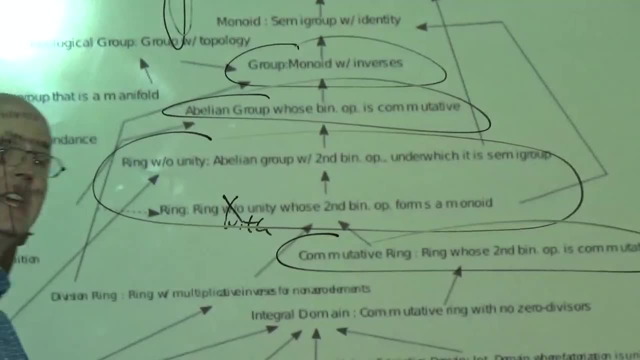 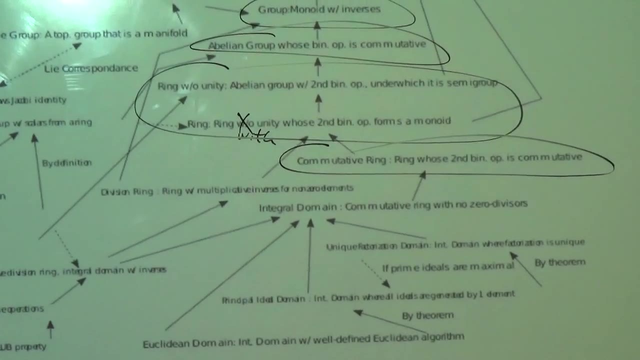 Commutative ring basically means multiplication is commutative. Matrices, matrix multiplication is not commutative. So a ring of matrices does not form a commutative ring. Let's see. I see the word field here. That says field. 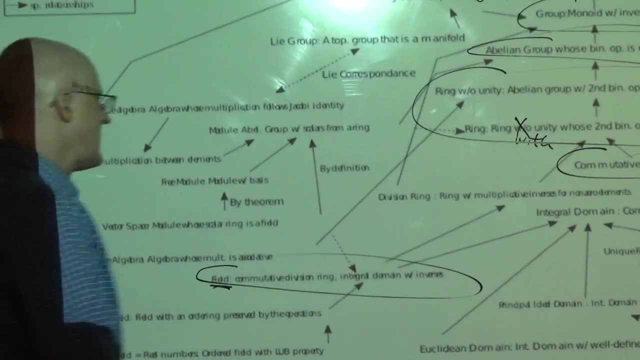 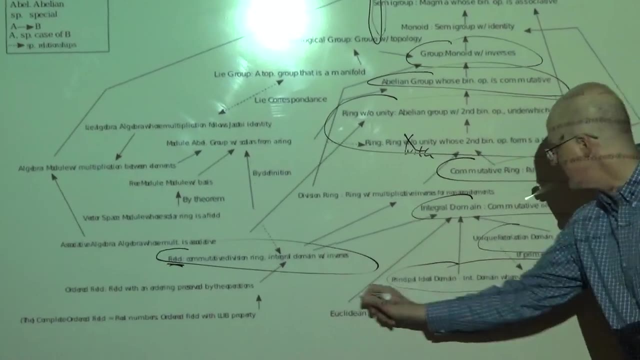 Kind of hard to see there. That's going to be important for us. And some of the stuff down here, integral domain, unique factorization domain, principal ideal domain, Euclidean domain, those are all going to come up as well in this class. We won't really talk about magmas. 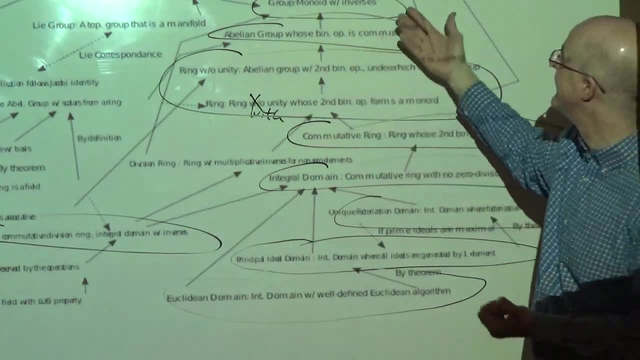 There's not actually much interesting to say about magmas. Semi-groups, monoids, I might mention those from time to time. Topological groups. This is stuff that's a little bit more advanced. 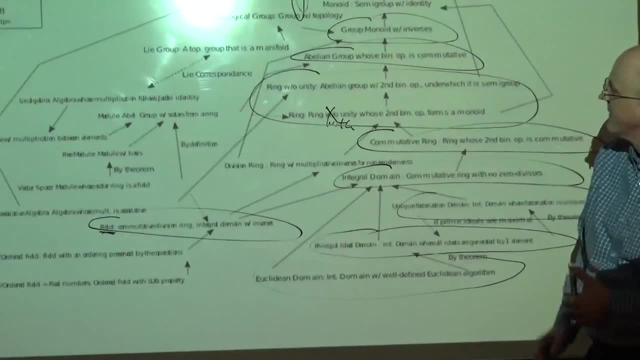 You need some other stuff besides this class. Over there. 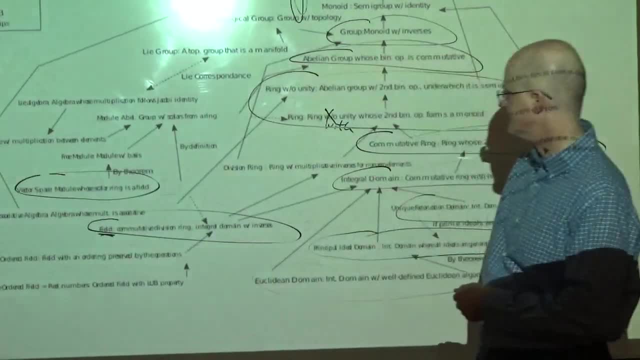 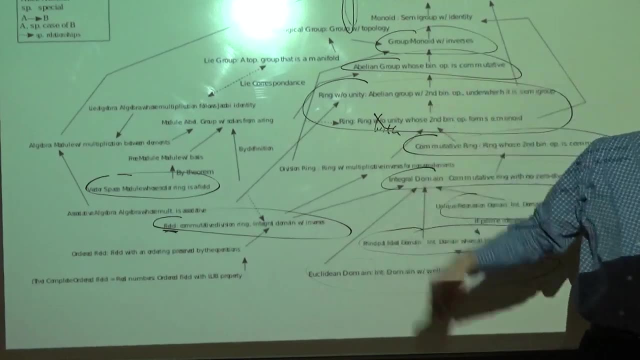 I do see vector space right there. So it doesn't make much sense to you now, but if you do go to grad school, you will appreciate this diagram more. Okay? 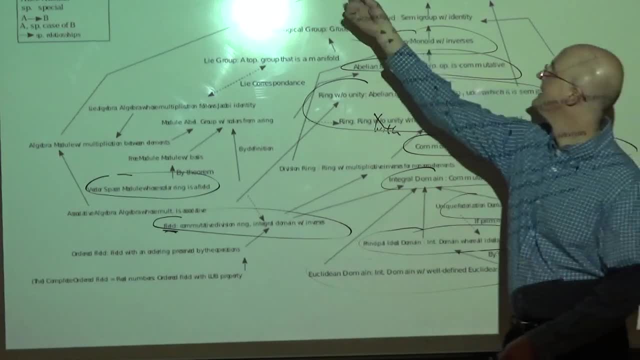 So you can try to see it from the future if you think you might go to grad school. 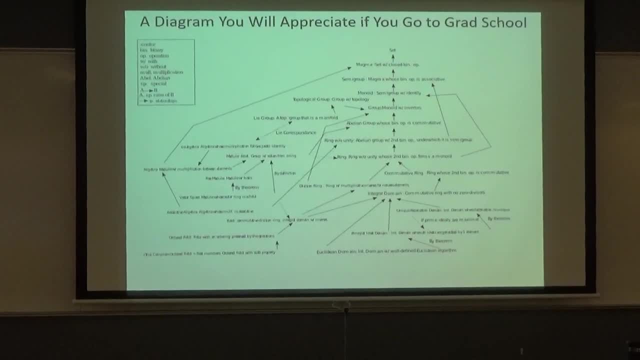 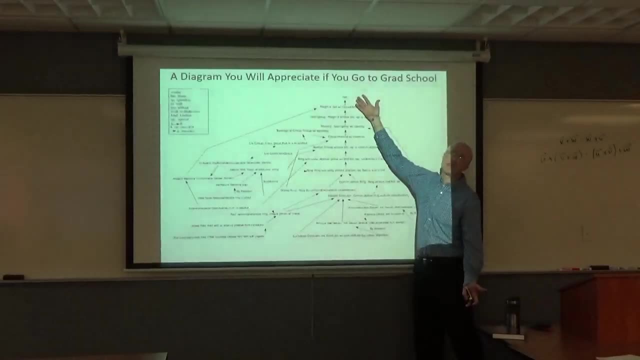 Showing the relationship between these different algebraic structures. Essentially going from bottom to top. This is sort of more general up here. Applies to more things. It's just set right there. 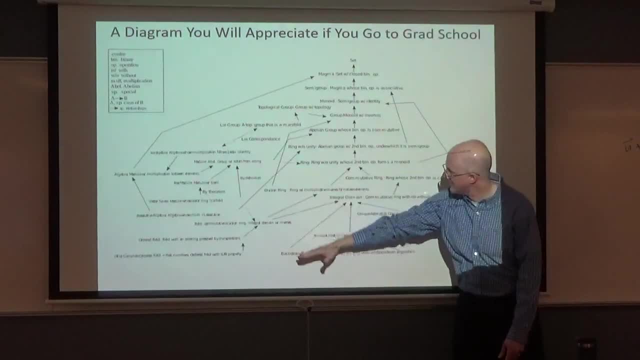 It's not really an algebraic structure. And these are, down here it's more specific you might say. 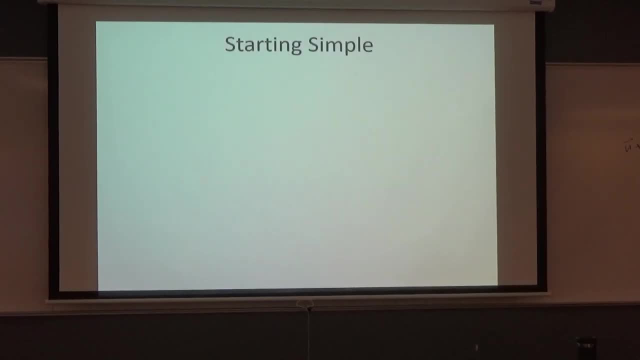 All right, we're about to do math now. Okay, so you may want to take some notes here. It's always good to start simple. 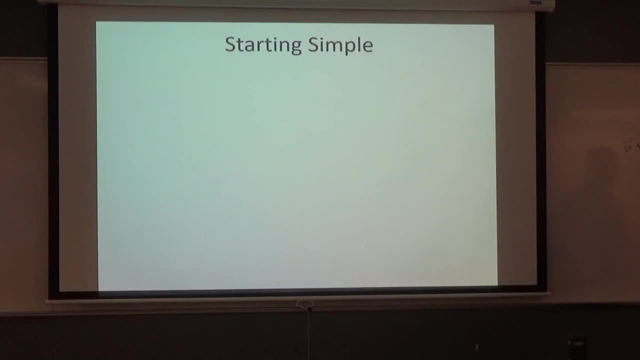 Start with things you know and then try to generalize. So by starting simple, what do I mean? I mean, well like for example, 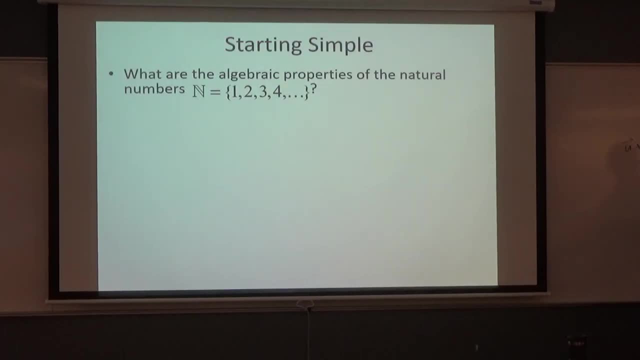 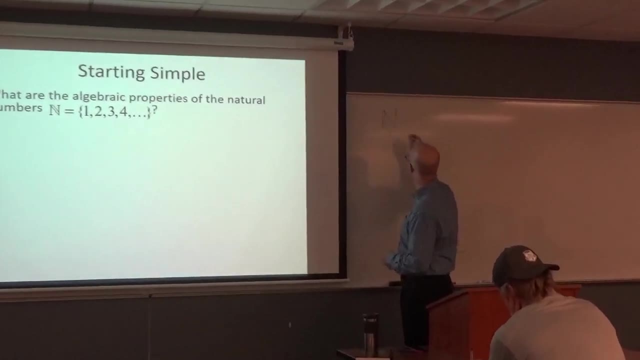 what are the algebraic properties of the natural numbers? This fancy n, which by hand I'll write like that, which is a little different than the typesetting. 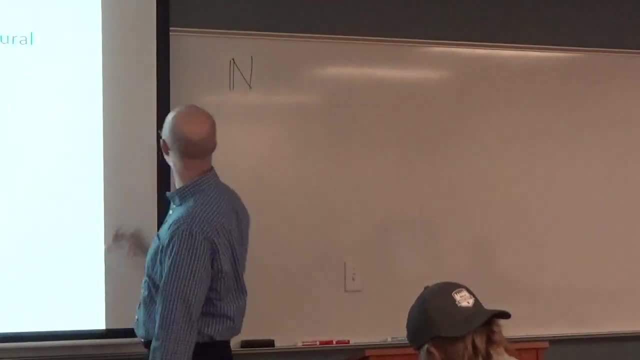 They put the double things through the middle, but I tend to write it like that by hand. 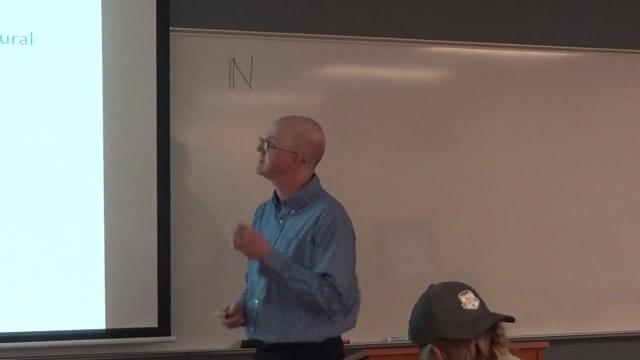 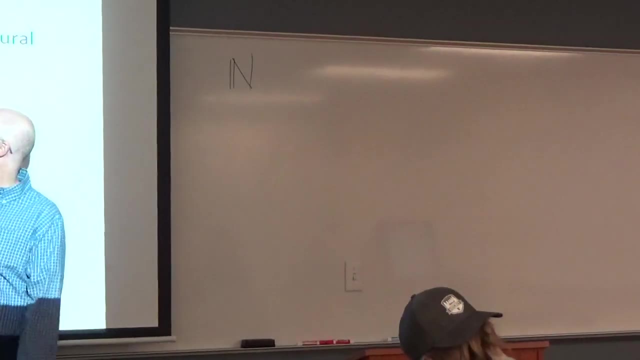 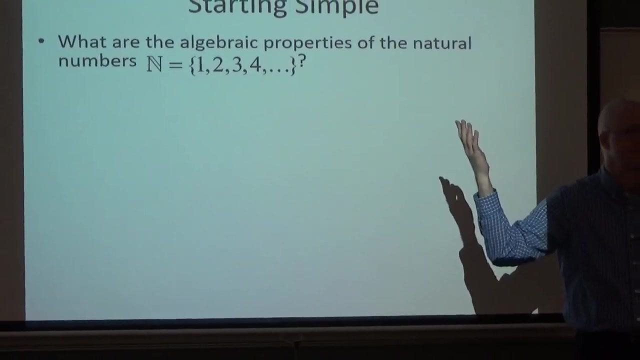 So this is a set. The set is typically called the set of natural numbers and that's why we're calling it n. It's the counting numbers. Not including zero. One, two, three, four, five, six, et cetera. So what are some basic properties of this? Well first of all, it's an infinite set. 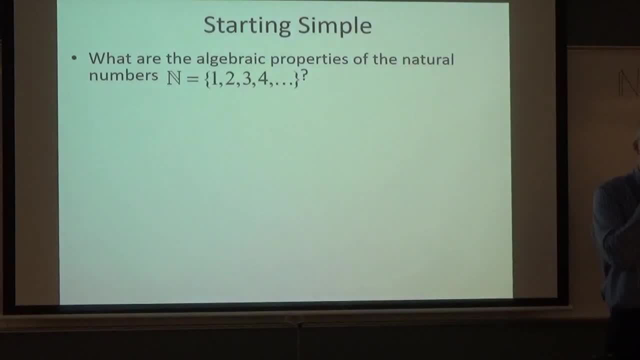 Secondly, you, if you think about it, would know there are operations you can do on this set. What properties does it have, for example, under the binary operation of addition? 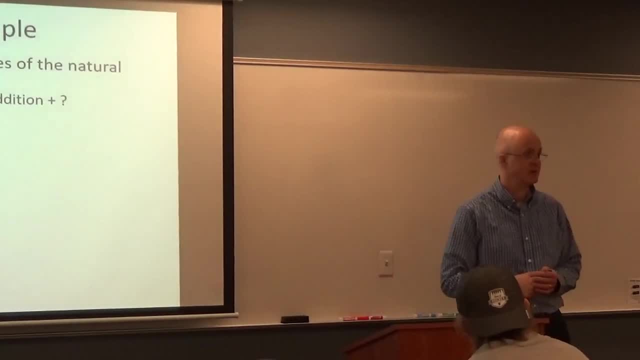 Well it does have properties similar to what vectors have when you have them. 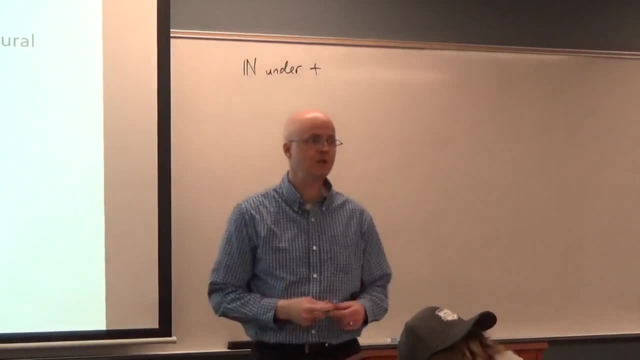 Binary operation, by the way, basically means you're taking two things and combining them to get a new thing. Okay, that's what binary operation means. 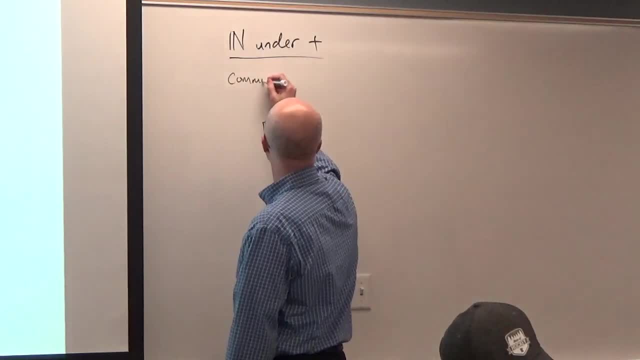 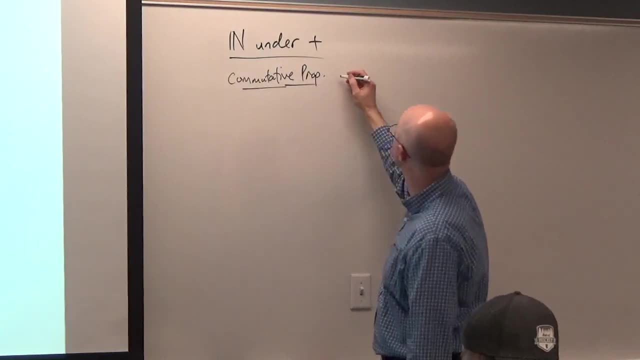 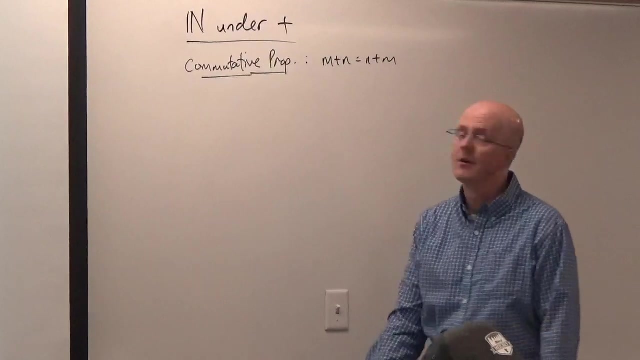 You've got the commutative property. You could write m plus n equals n plus m 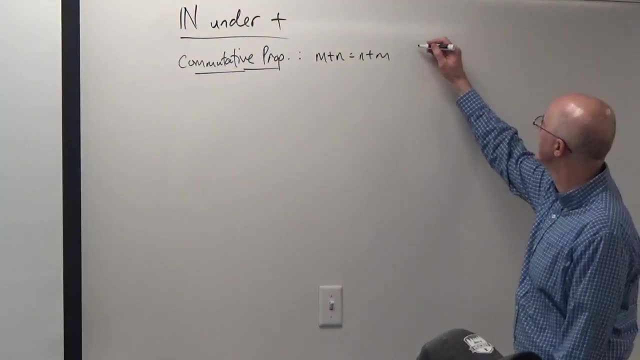 for all natural numbers, m and n. 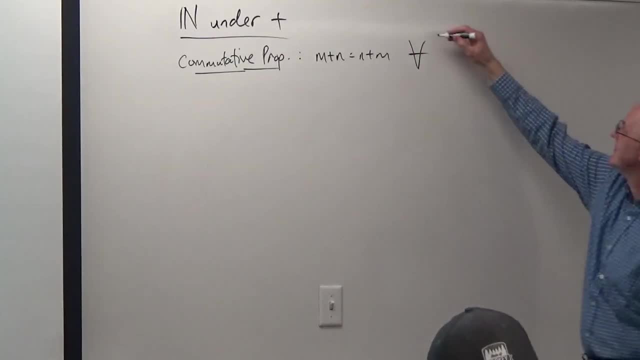 Upside down a means for all. We will use a lot of shorthand symbols in here. 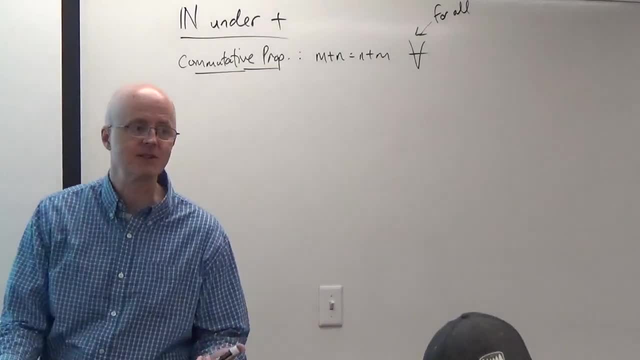 Partially because it just makes the writing faster. Partially because I just enjoy doing it. It's fun to make upside down a's. 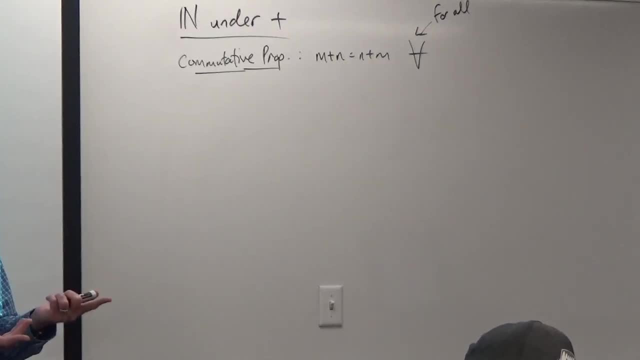 Especially if you're writing your paper and your friend who doesn't know much math comes by and says, what in the world is that? 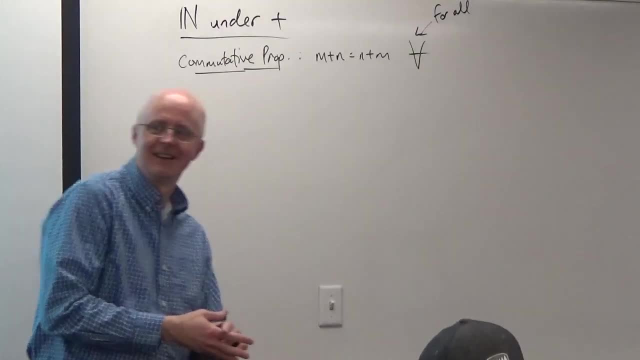 So that means for all, or you can show your parents. 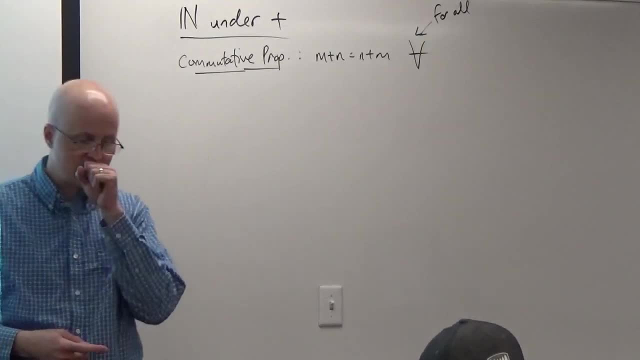 As far as, excuse me, as far as writing proofs goes, you should write your proofs in the set. 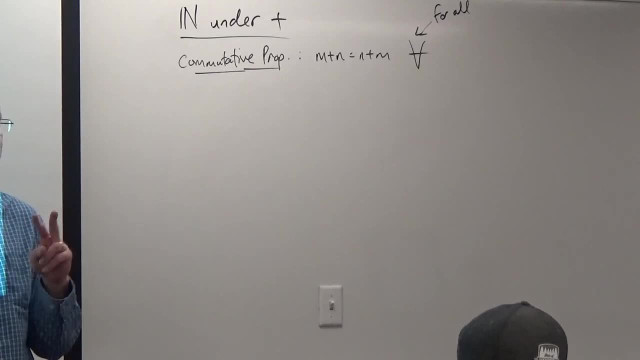 For proofs in the sentences, there are going to be two proofs due on Friday. 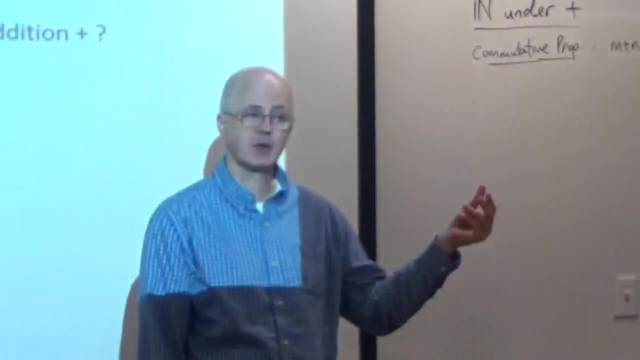 In addition, those are going to be the graded ones. In addition to completion problems, 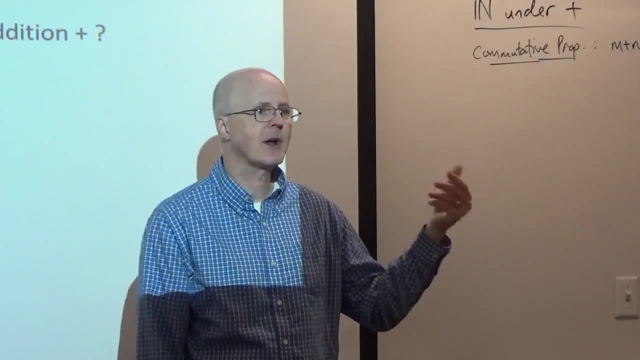 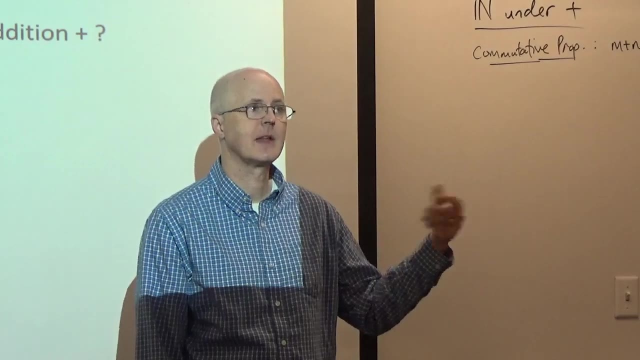 which you should also do, but typically are a little bit more calculation focused, maybe some proofs. I did put a solution key for the completion problems that includes more than just what's assigned on Friday up on Moodle. 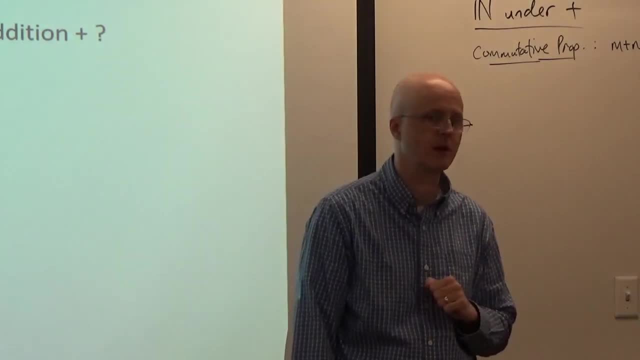 You'll see underneath the list of problems to work on for Friday. 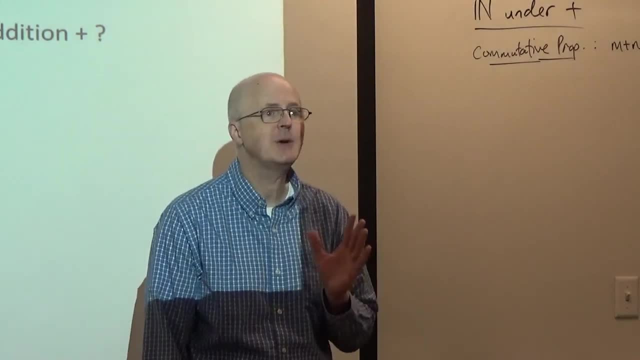 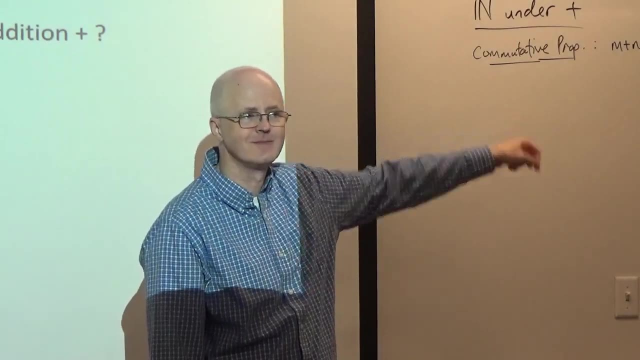 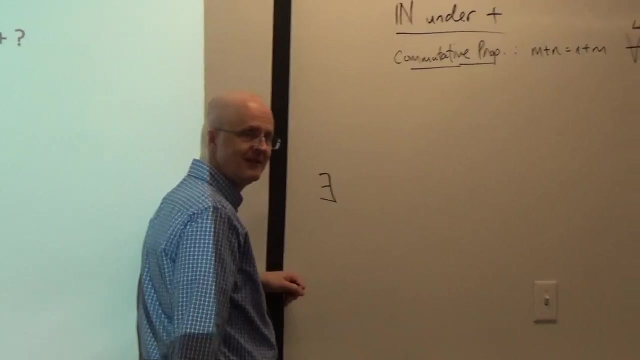 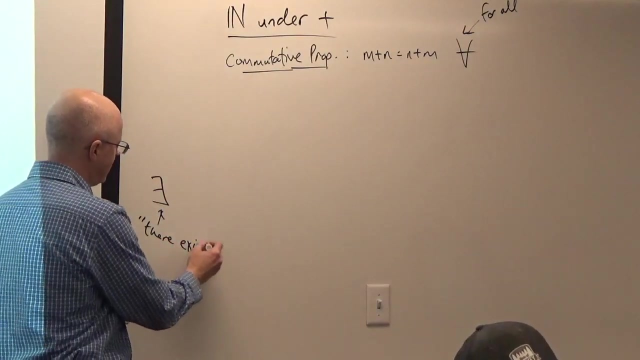 But in doing proofs, you should write in sentences, but you can abbreviate, okay? You can use that abbreviation, for example, for all. Another fun abbreviation is a backwards E for there exists. 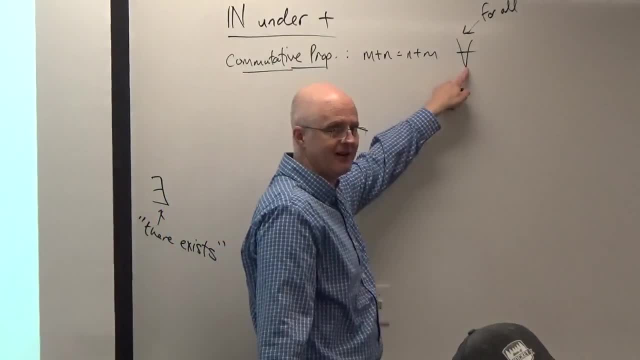 More officially, this is called the universal quantifier. 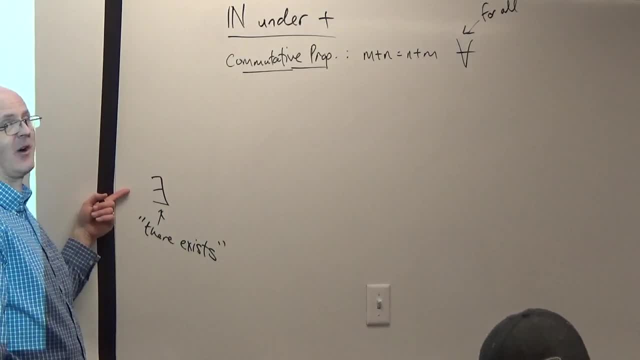 This is called the existential quantifier. Though I won't usually say those things. 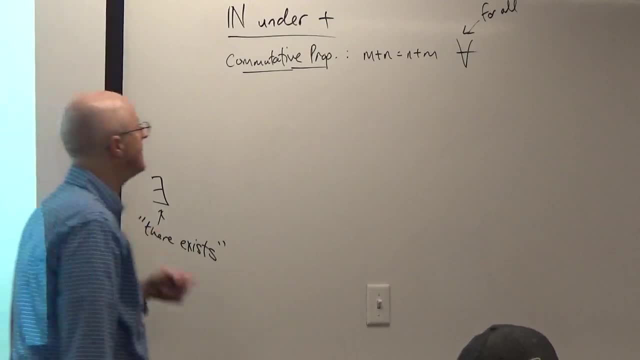 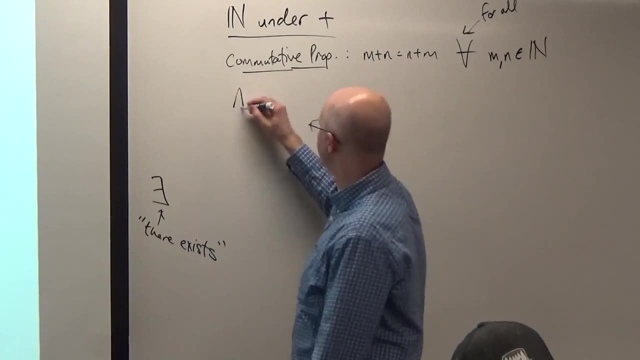 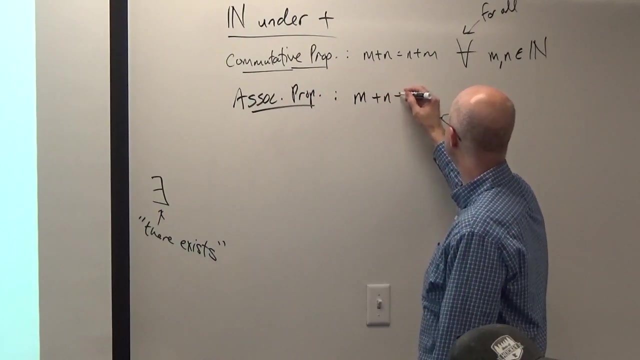 I usually say for all or there exists. So this is true for all numbers in the natural numbers. The associated property holds. Should I use an O? Probably I should avoid using an O. 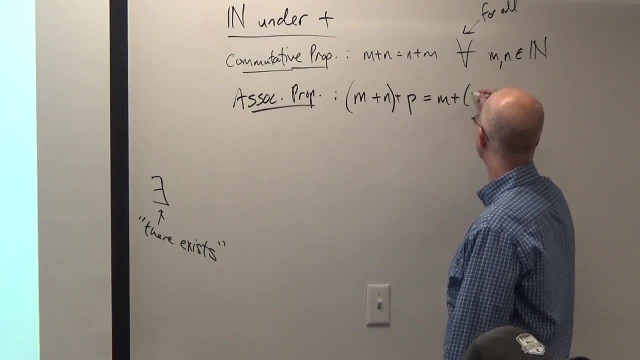 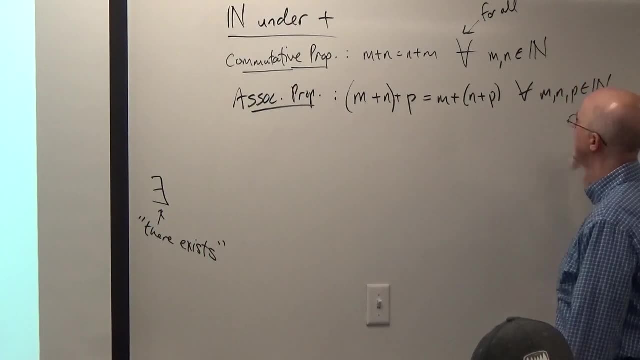 I'll use a P. Because you might think the O is a zero. 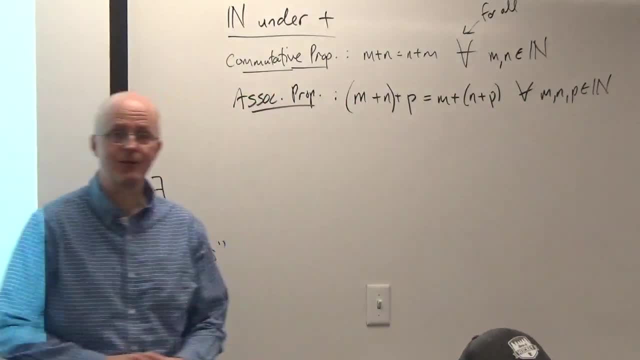 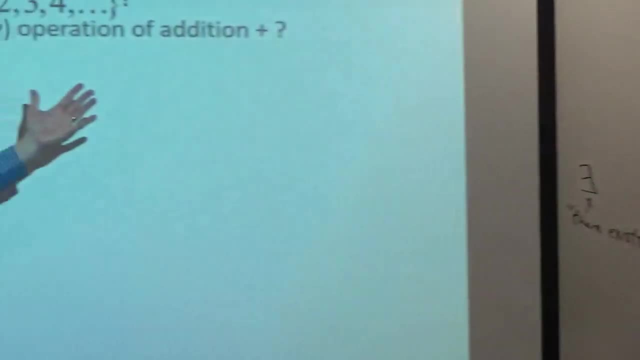 Should I write down M plus zero is equal to M for all M? No, because N doesn't have zero in it. 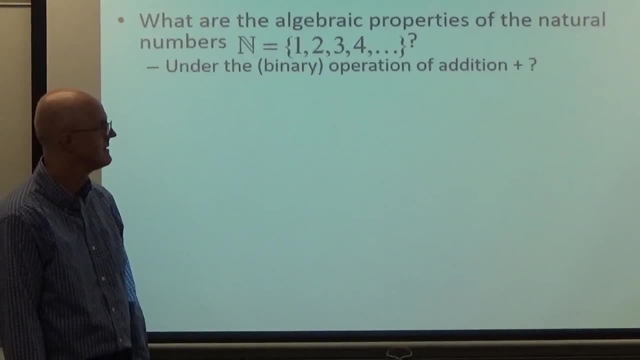 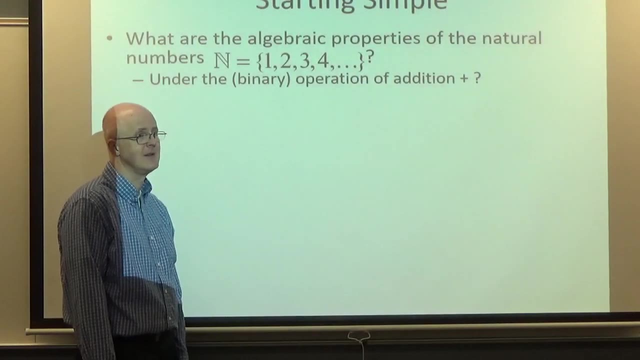 Satisfies the commutative property, the associative property. I'm not talking about multiplication here, so I don't want to think about the distributive property. Of course, zero does exist. 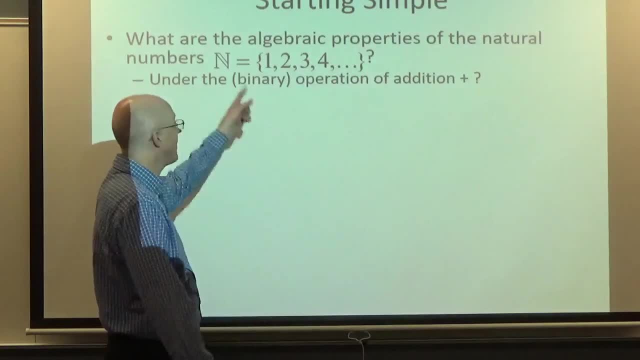 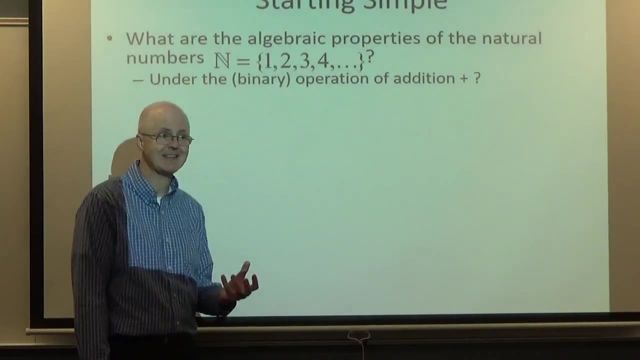 Zero is a number, the additive identity, but it's not part of N. So N, the set of natural numbers, as an algebraic structure, does not have an additive identity. It does not contain zero. 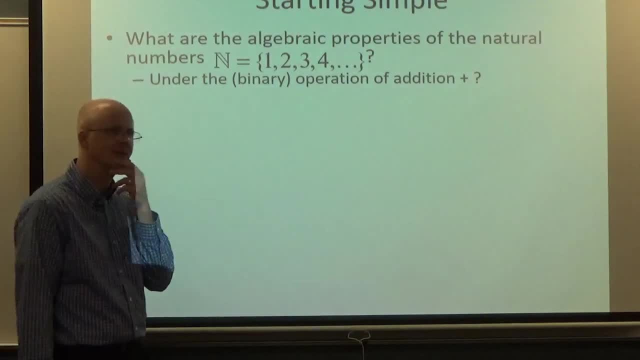 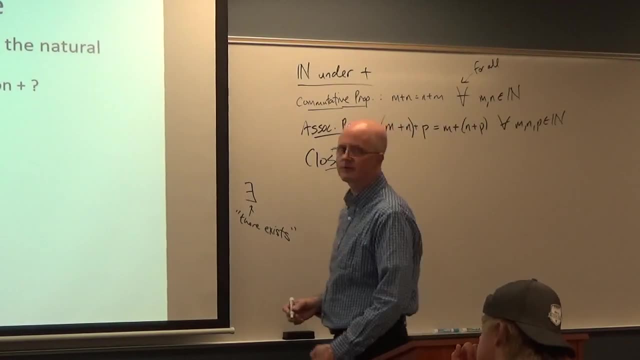 How about closure? What does the word closure mean? You should have talked about that in your algebra. 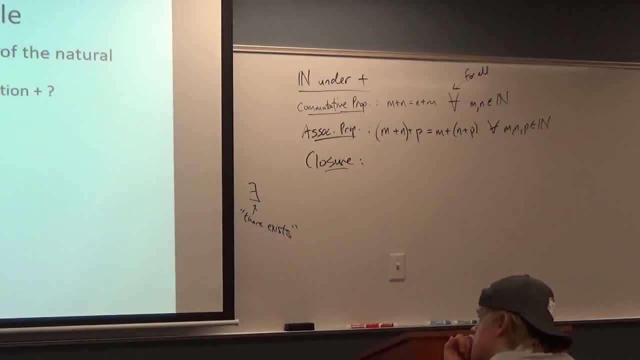 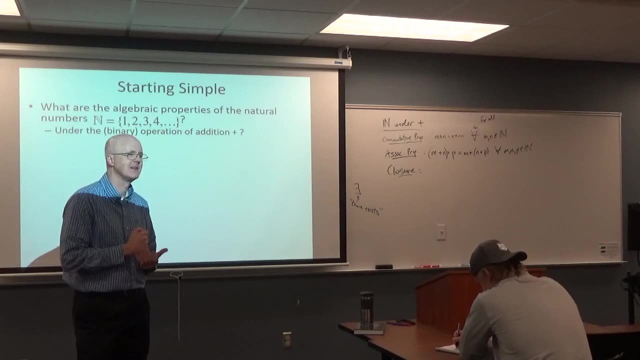 Remember what closure means? You say a vector space is closed under vector addition. 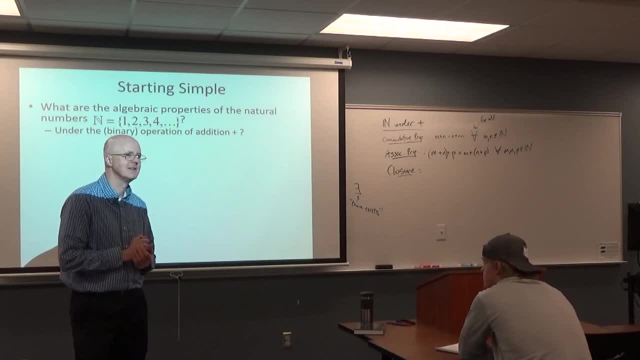 What does that mean? You add two vectors, what happens? You get another vector in that space. Yeah, you get another vector in that space. And that's especially important for subspaces. 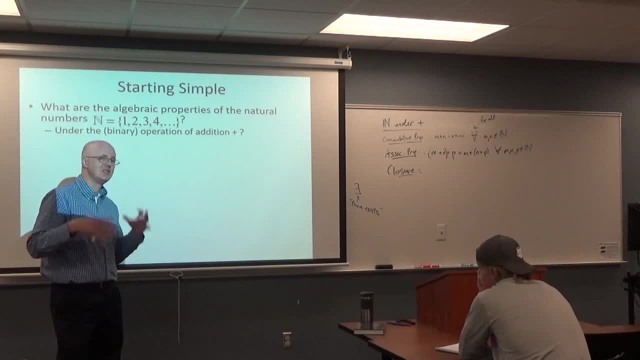 You remember subspaces? Geometrically, thinking of your vector space, for example, as being three-dimensional space. 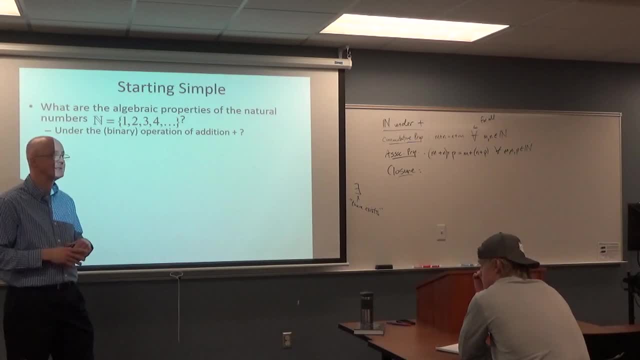 Two-dimensional subspaces of three-dimensional space are planes that go through the origin. And when you add two vectors in a plane, you get another vector in that same plane. 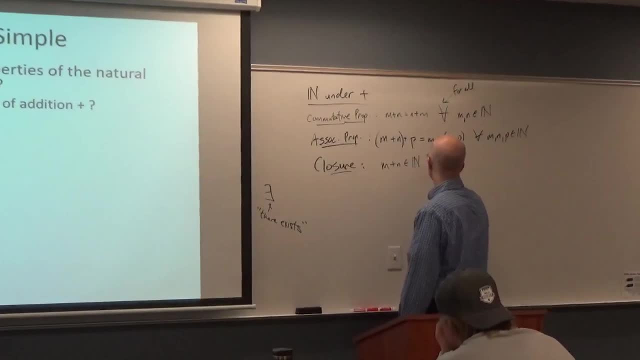 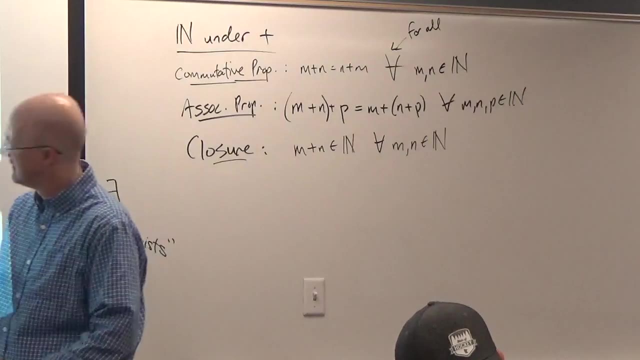 You could write M plus N is a natural number for all M and N that are natural numbers. 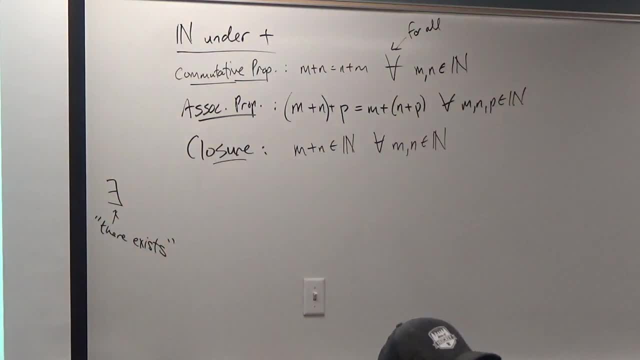 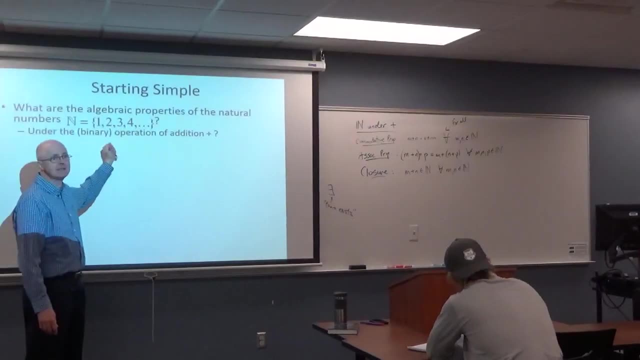 Actually, any time I use the word binary operation on the set, that actually automatically means it's closed for that operation. 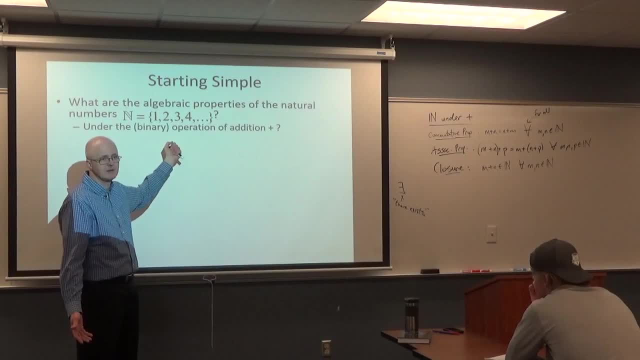 But sometimes it does take proof. To show that the operation is closed. 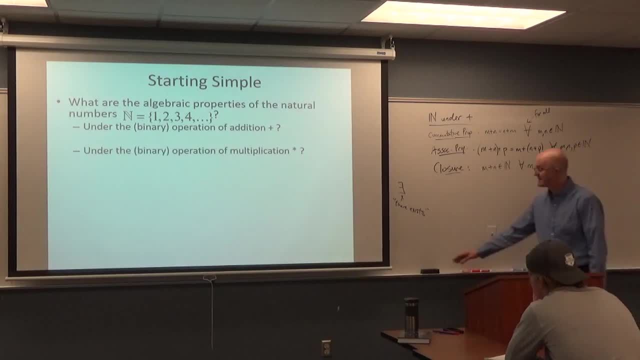 How about under multiplication? Can I write similar things? Except with a dot instead of a plus. Yep. 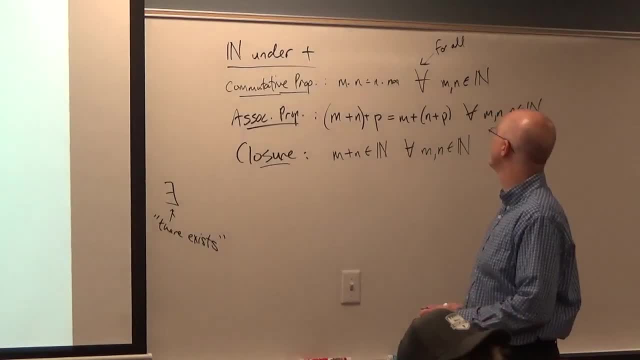 M times N equals N times M for all natural numbers. 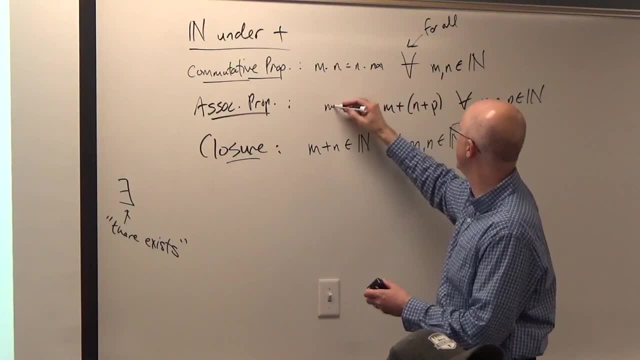 M times N times P with the M times N done first does equal... 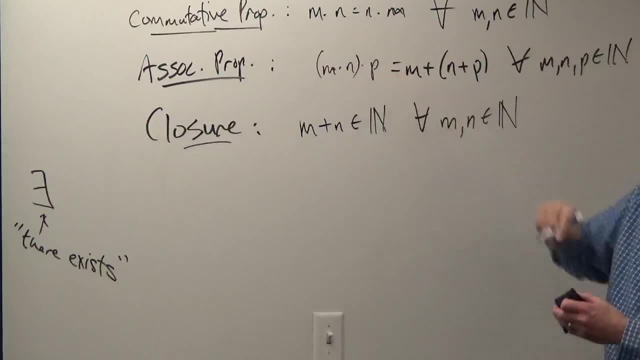 Did I forget my equal sign here before? Guess I just erased it. 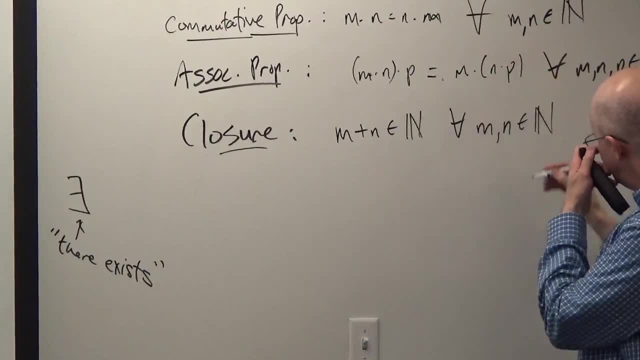 Equals M times N times P with the N times P in parentheses. So you do that first. 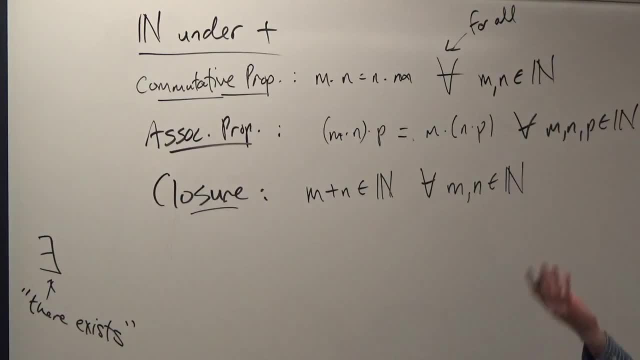 That's true as well. By the way, we aren't proving these things. We are taking them as known in this case. 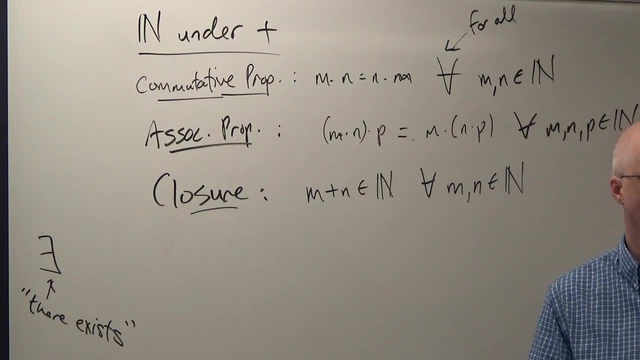 You can assume you know everything there is to know algebraically speaking about the natural numbers, about the integers, about the rationals, about the reals. 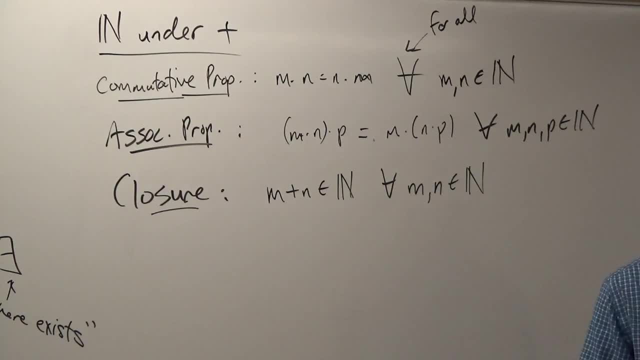 We are going to make that assumption. So we're not completely proving things from scratch in this class. 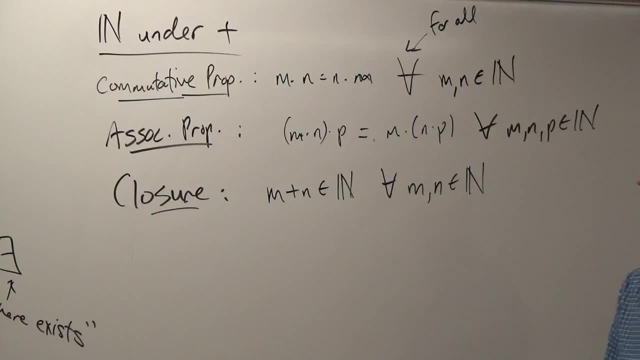 At least for examples like this. Okay? 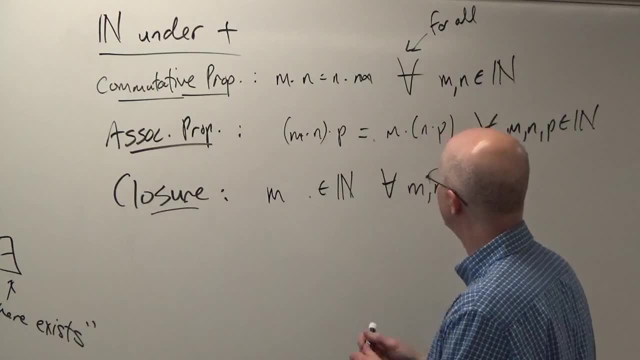 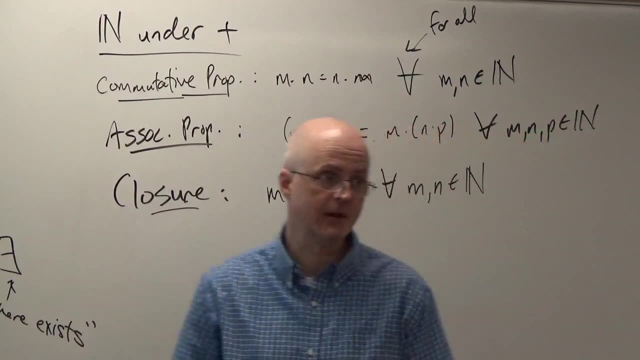 And there is closure. M times N is a natural number for any two given natural numbers. And in particular, you never get a product of zero, and you never get a negative product. 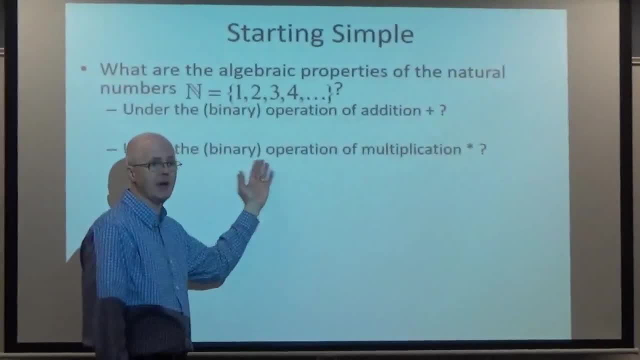 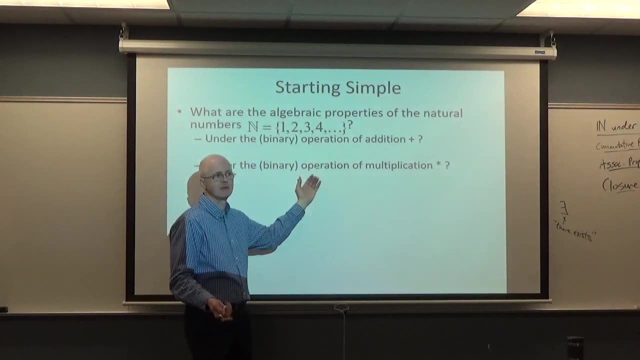 And again, for emphasis, when I say binary operation, when you use those words, you really automatically mean it's closed under the operation. 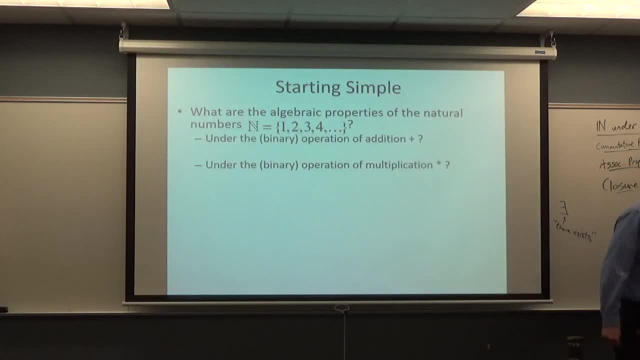 How are you doing? Paying attention? Having fun yet? Smile. 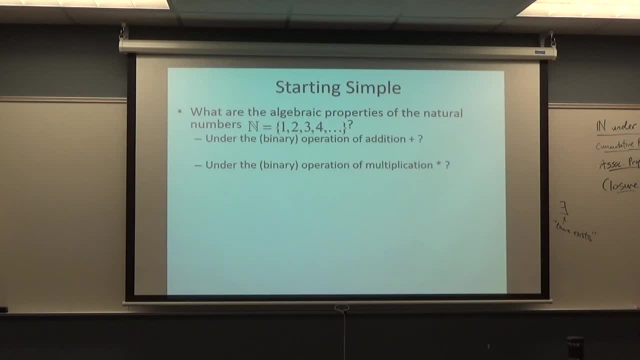 I know this part is not the most exciting stuff, but I think it does get better. Hmm. 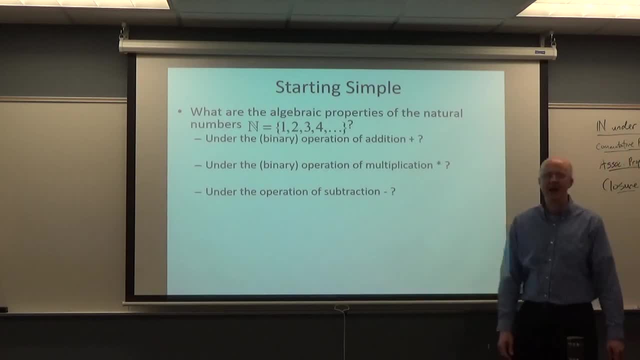 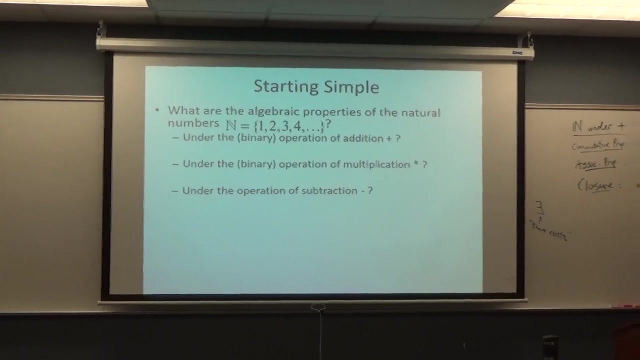 Operation of subtraction. Notice I did not put the word binary in there. If I just say operation, is it possible closure, for example, does not hold? Yes, that is possible. 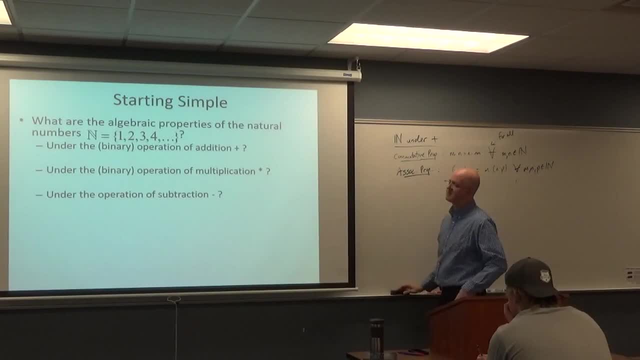 I mean, technically it's still a binary operation. You're still combining two things to get a new thing. 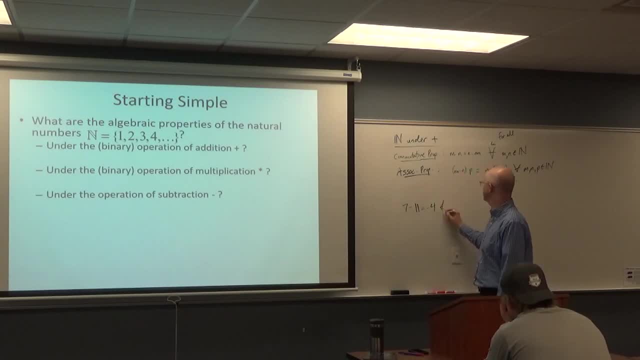 Of course, 7 minus 11 is negative 4, which is not a natural number. 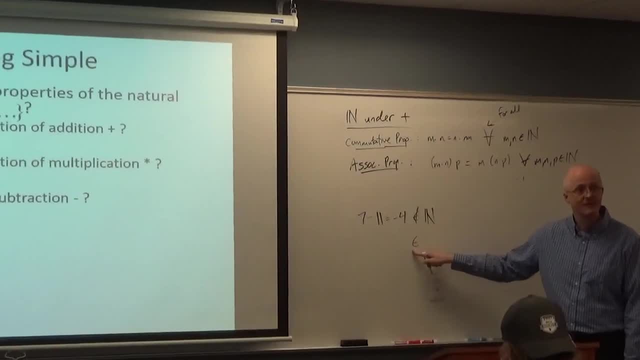 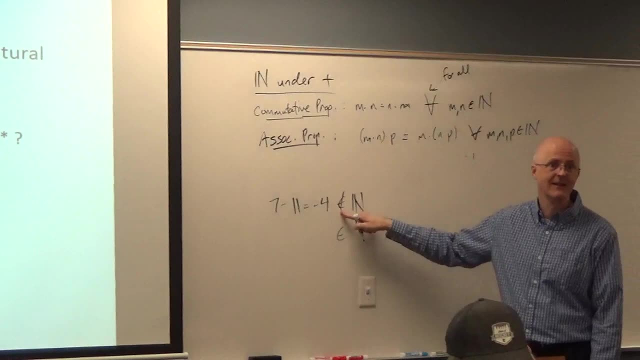 By the way, this funny looking E means it is an element of. If I put a slash through it, it means it's not an element of. 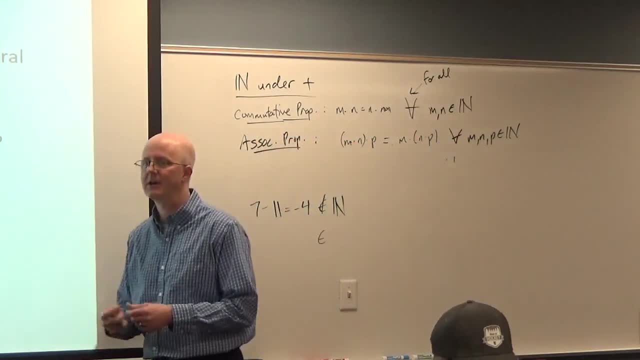 Technically, you might say binary operation is still included just combining two numbers to get a new number. 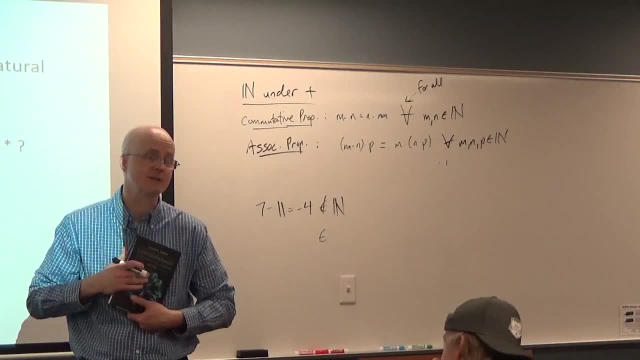 But again, in our textbook, I'm doing this because our textbook does this. 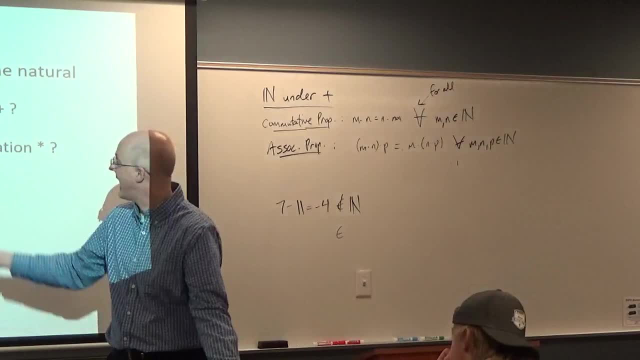 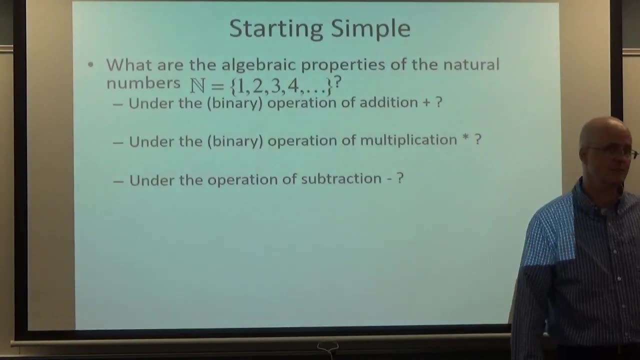 When you say binary operation, you automatically mean closure. So this operation, as an operation of natural numbers, is not closed for the set of natural numbers. 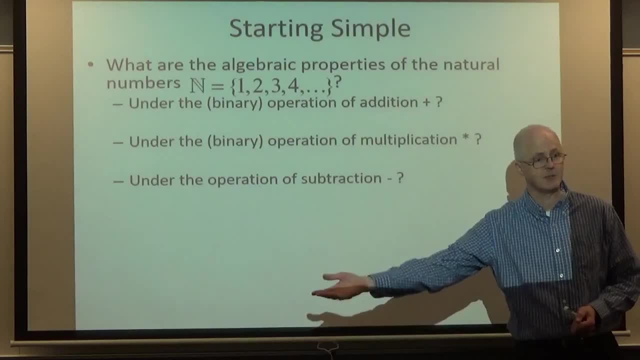 Though it is closed for the set of integers when you include 0 in negative numbers. 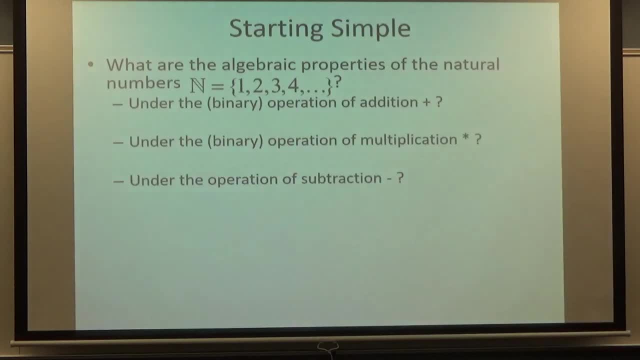 Negative whole numbers. And what if we do include 0? 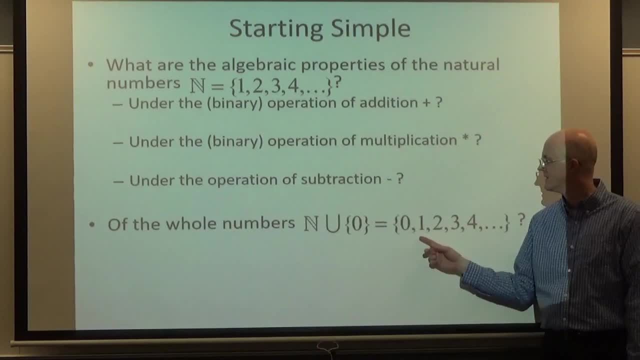 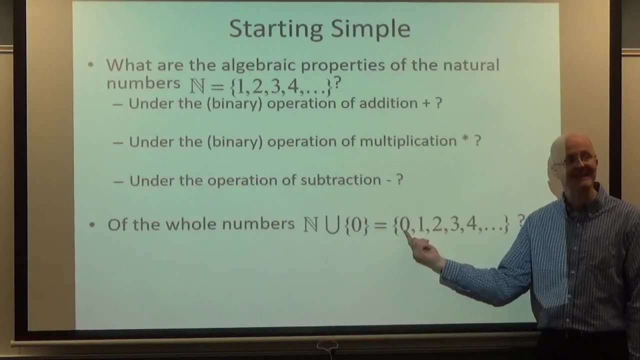 Take the union of the naturals with 0. Do we get any new properties? Well, yes, you get one new property. You get, under addition, you get a 0. You get an additive identity. 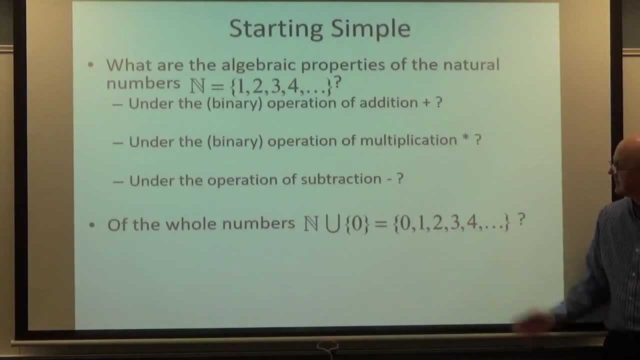 0 plus any number, any number in the set is that same number. 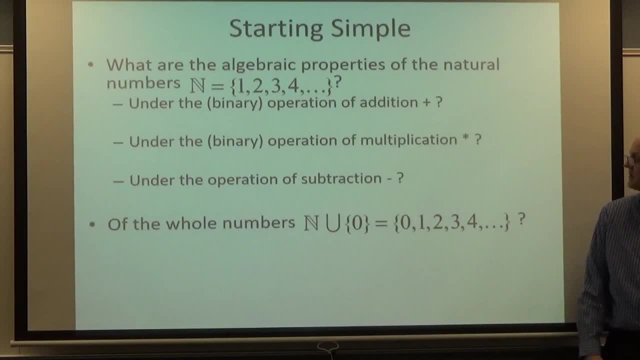 0 plus 5 is 5. 0 plus 27 is 27. 0 plus 0 is 0. 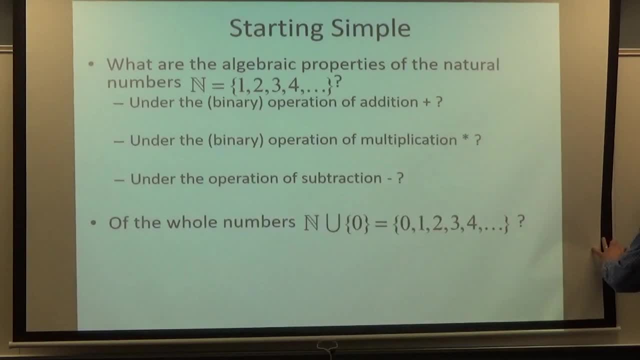 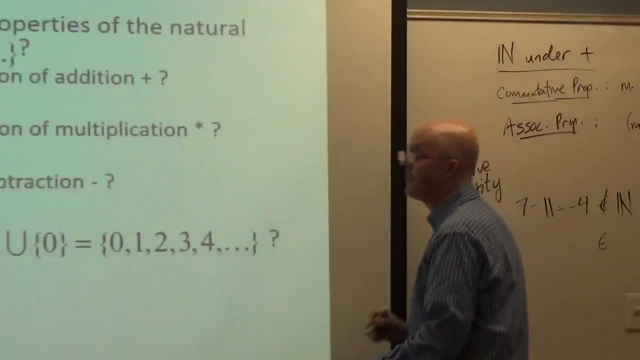 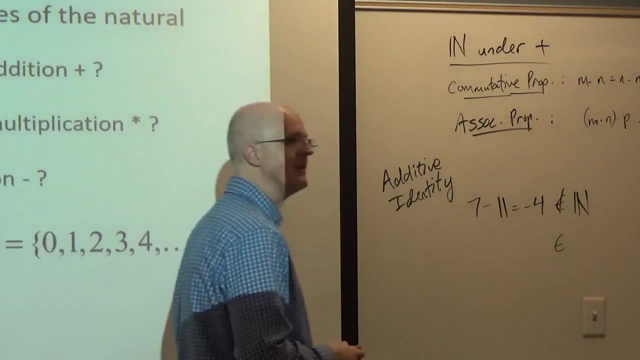 0 is the additive identity. Just like the 0 vector is the additive identity for vector spaces. 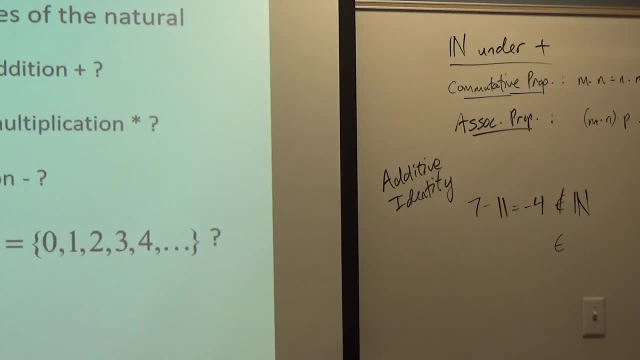 Add it to any vector, you get that same vector back. 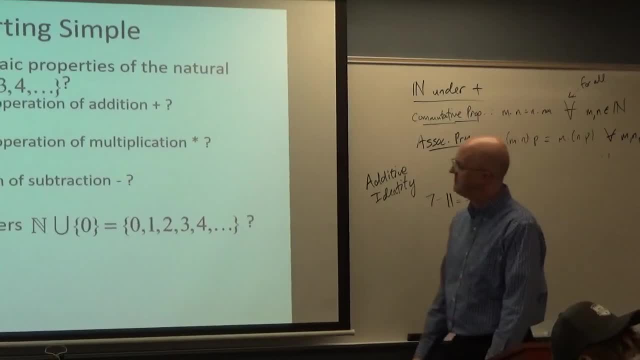 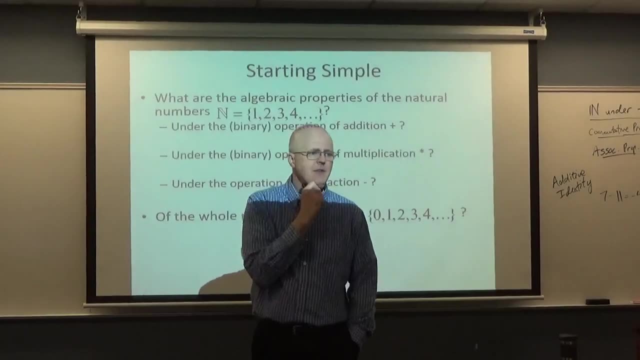 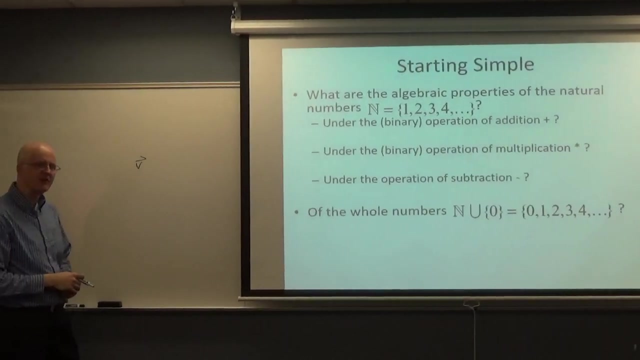 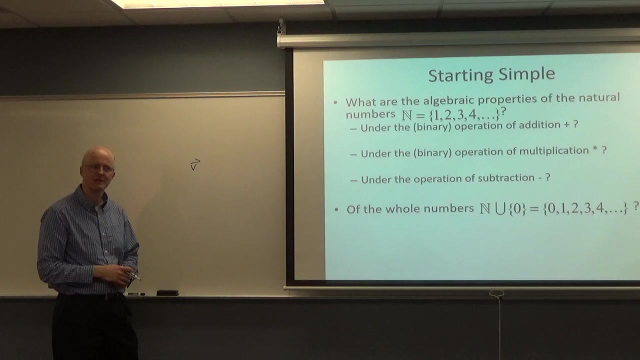 We are missing, though, even when we include 0, another property that might be nice to have, that we had for vector spaces. Given any vector, v, is there a vector such that when it's added to v, you get the additive identity? You get the 0 vector. 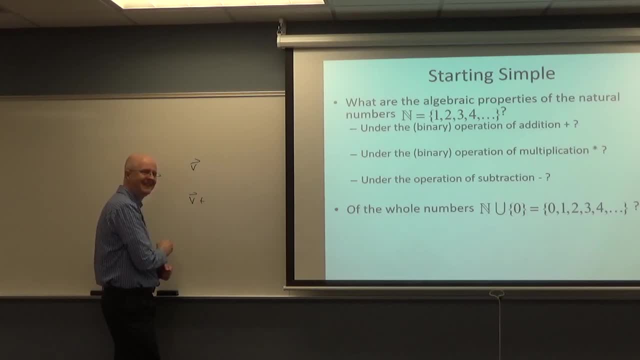 How would I write it? There is. 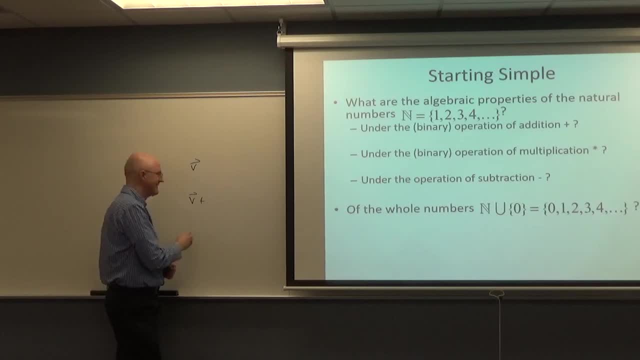 What's the typical notation for it? Negative v, yeah. 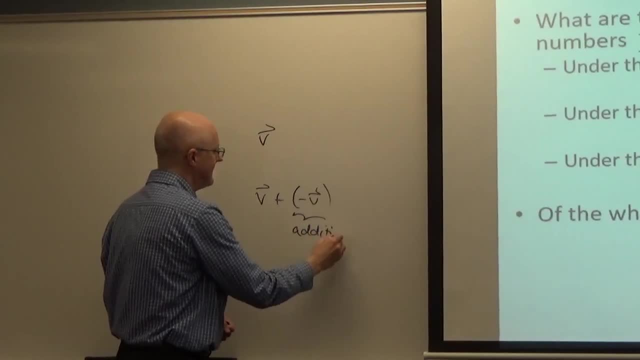 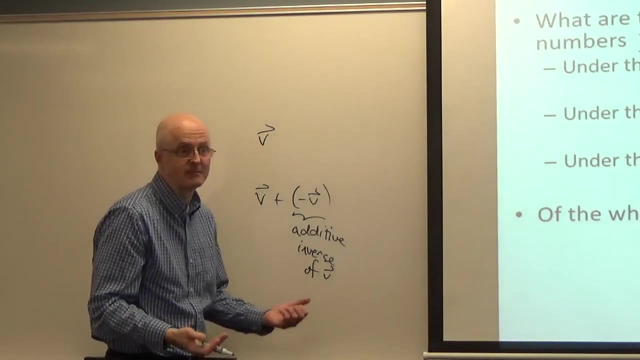 It's an additive inverse of v. And really, additive inverses are what help define subtraction. 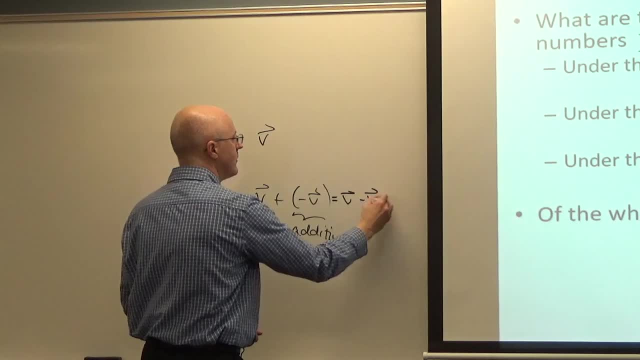 And yes, you can write this is v minus v, which is the 0 vector. 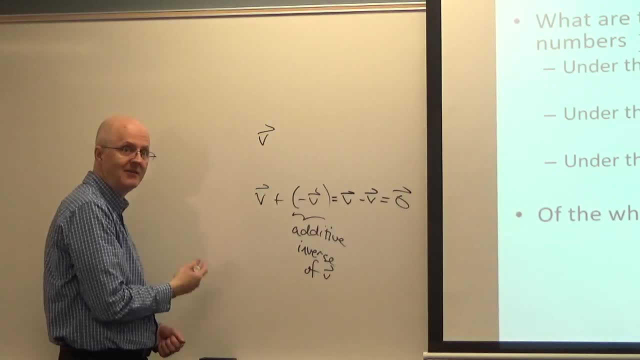 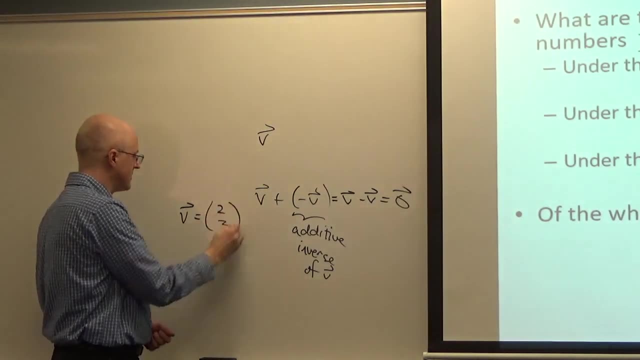 By the way, of course, for particular vector spaces, you might want to say what, if v is something, then what is negative v? If you're talking about, say, column vectors with two entries, if v is , then minus v, 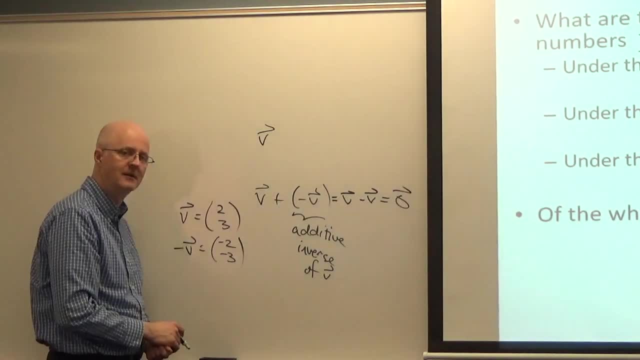 has entries negative 2, negative 3. 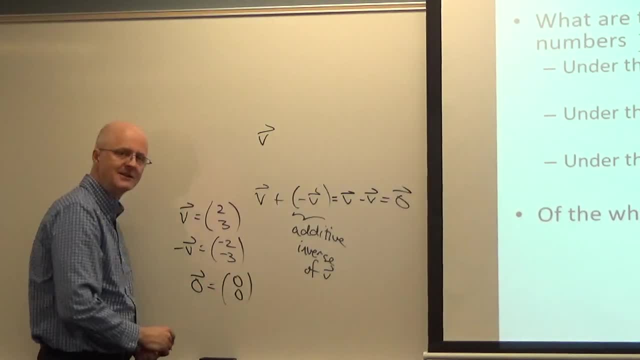 And the 0 vector has all entries in the 0 if you're talking about 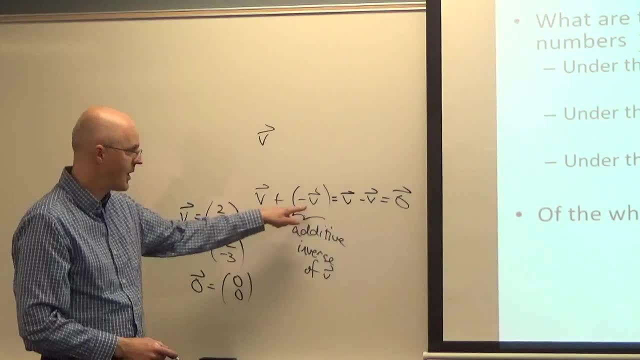 that particular vector space. But when you're talking abstractly, you just write negative v. 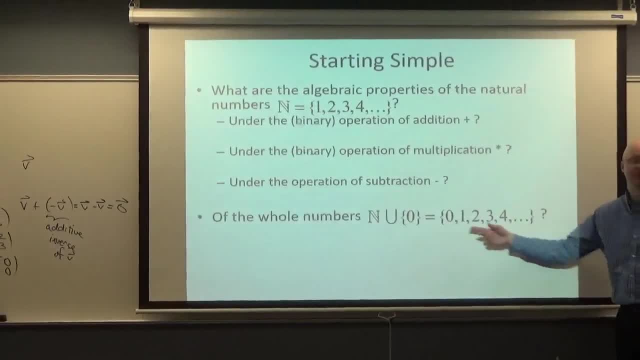 Even when we add 0, we don't have any additive inverses except for 0 itself. 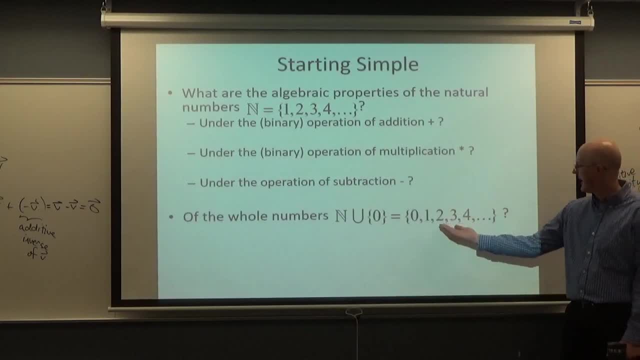 0 is its own additive inverse. But, you know, what's the additive inverse of 3? It would be negative 3. 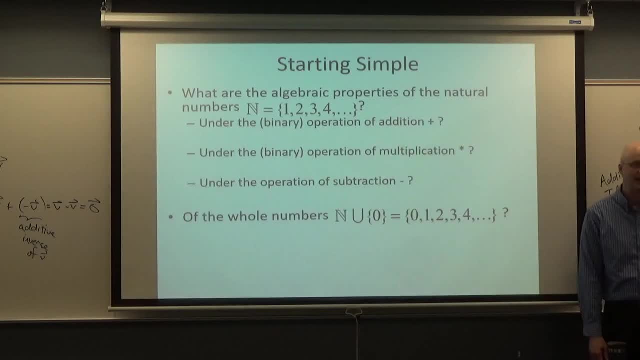 Negative 3 is not part of this set. So this set under addition does, it's got an identity, but not additive inverses. 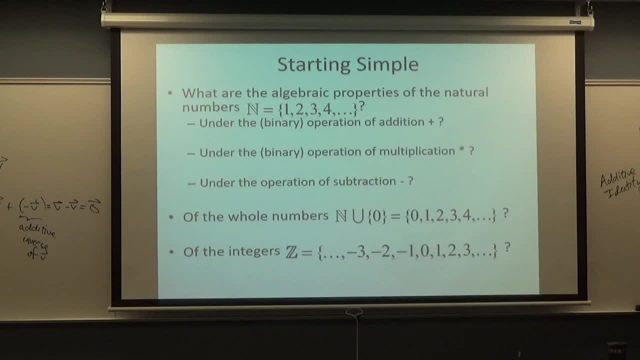 When we include negative numbers, though, then we have additive inverses. 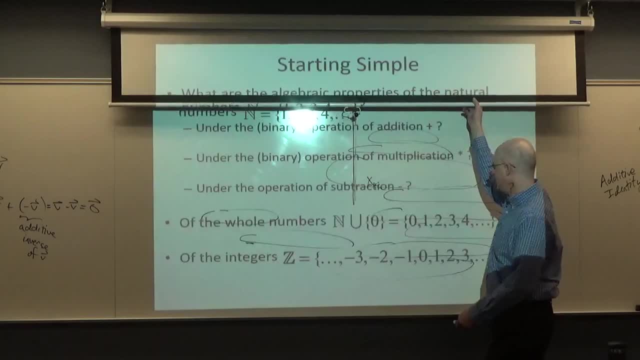 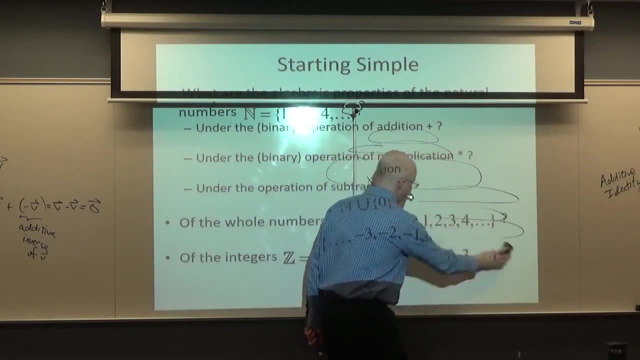 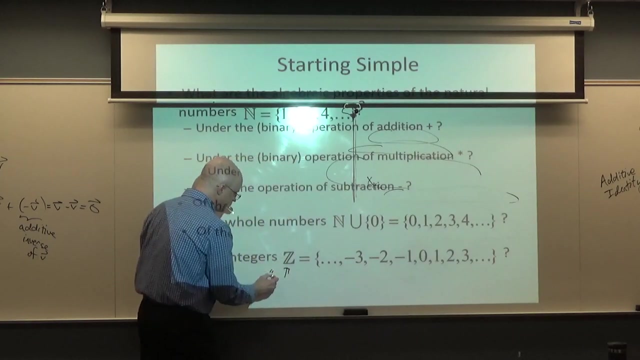 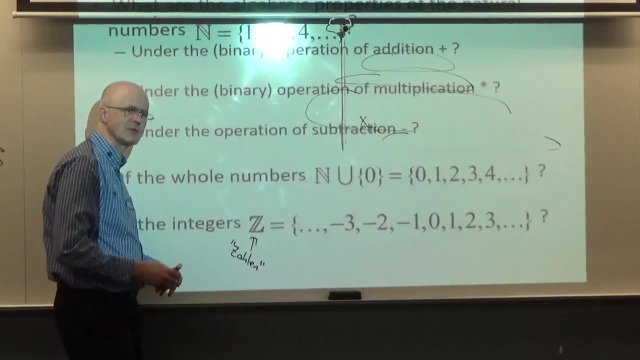 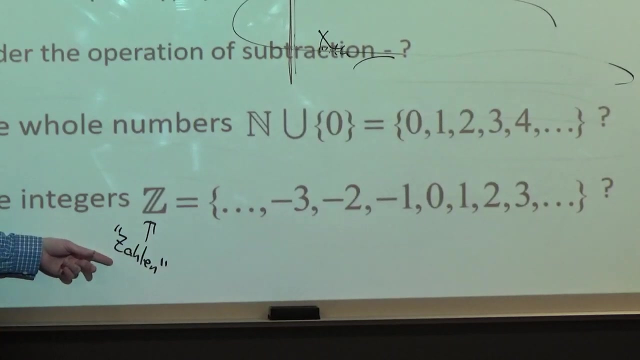 And z here, the integers, is our first example of a group. Z, by the way, this is the set of integers. It stands for, it's a German word, zahlen is how you say that. Don't say zahlen, say zahlen. It's basically a word that means number. 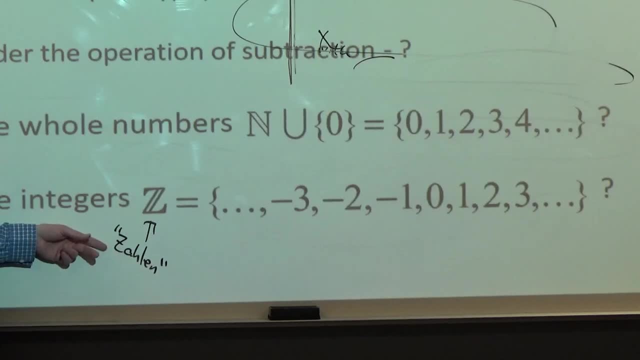 They also use the word numere, I think. But zahlen is also a word that means number. That is the standard symbol used for the integers, which includes the positive counting numbers, the naturals, it includes 0, and it includes the negative counting numbers, additive inverses of the originals. This is a group. 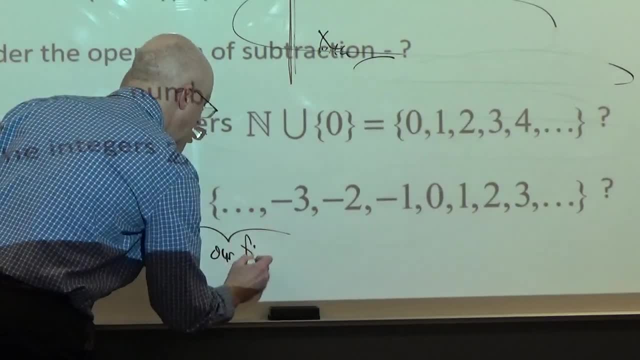 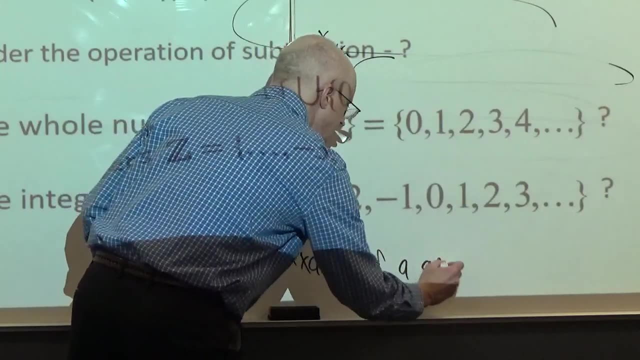 This is our first example of a group 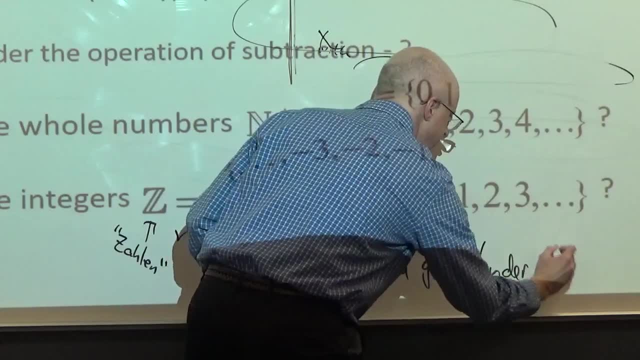 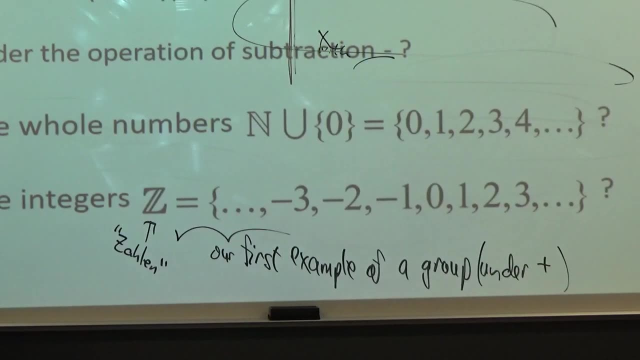 under addition in this case. The operation, the binary operation for this group is addition. Groups have, they're sets with a binary operation, so that automatically means, for our author at least, that it's closed under the operation. I'll try to reemphasize that every time. 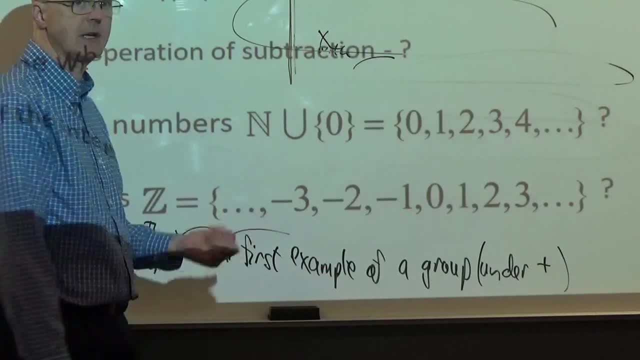 Binary operations mean it's closed. You add any two integers, you're going to get another integer. 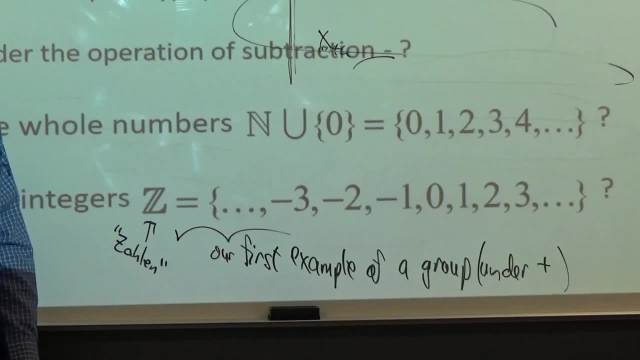 Satisfies the, so closure, associative property. 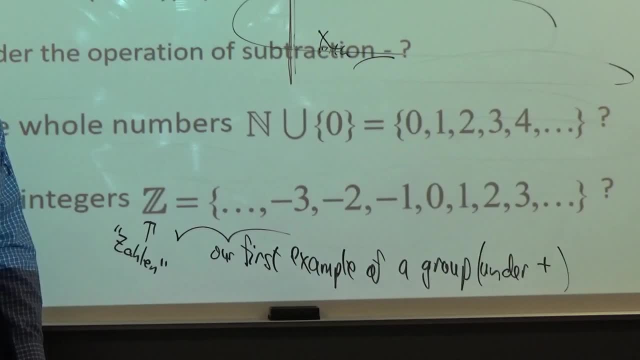 The existence of an additive inverse, in this case, is 0. 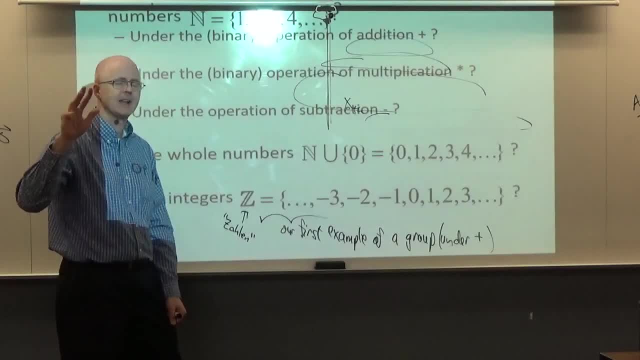 And every element has an additive, I meant to say additive identity, 0. 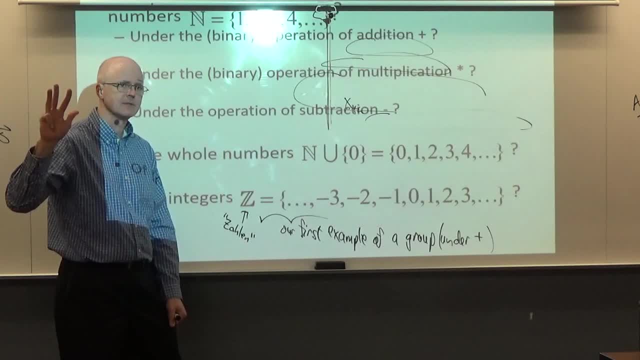 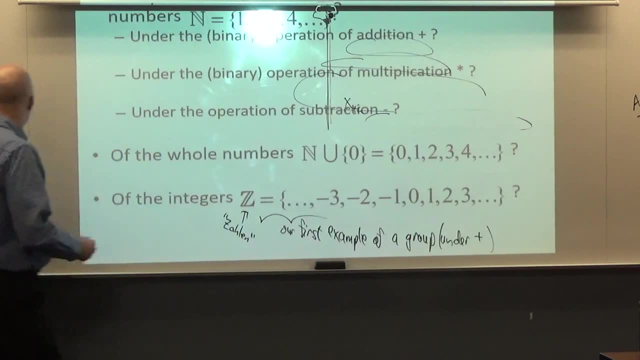 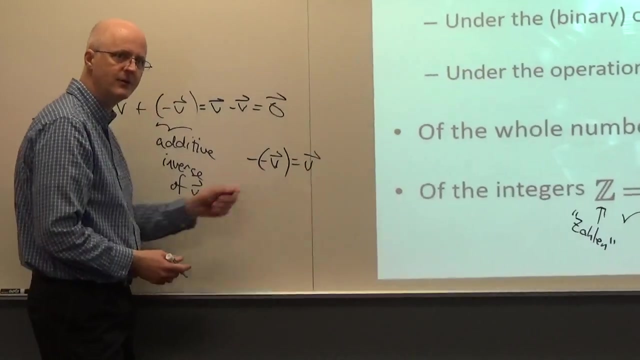 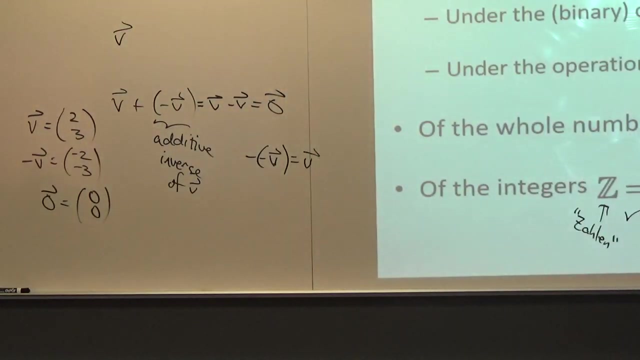 Every element has an additive inverse. The additive inverse of 7 is negative 7. The additive inverse of negative 25 is positive 25. The additive inverse of negative v is v. You can use that kind of notation. Okay? So that's our first example of a group. 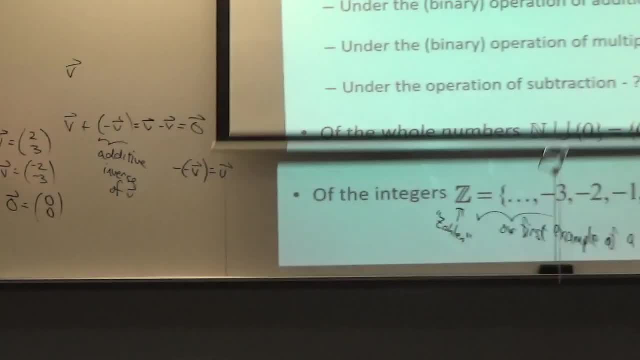 That's something familiar, right? I think I better go over the next slide quickly 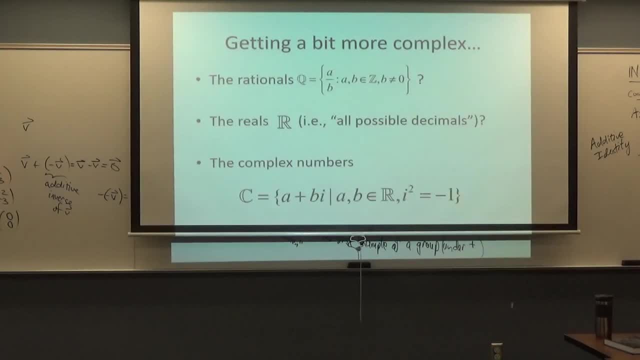 for the sake of time. We can get more complex. 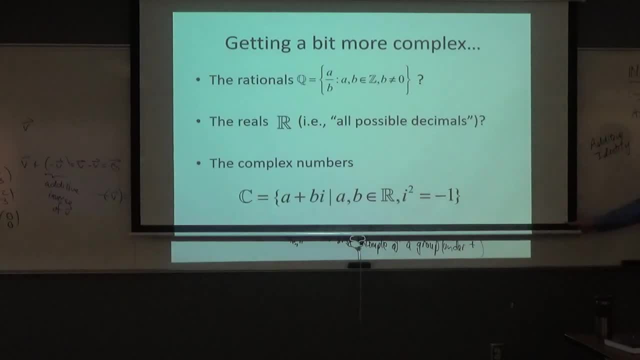 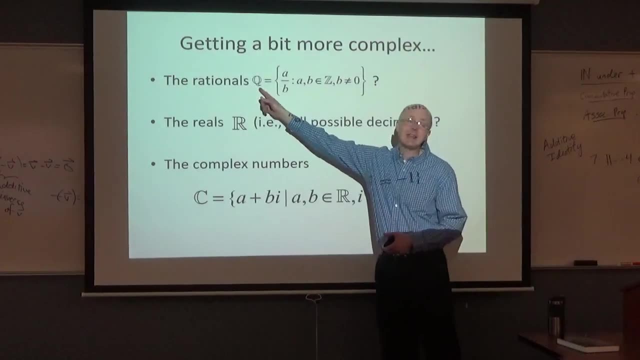 We can consider the rationals, q, standing for quotient, that's why we use a q for the rationals. 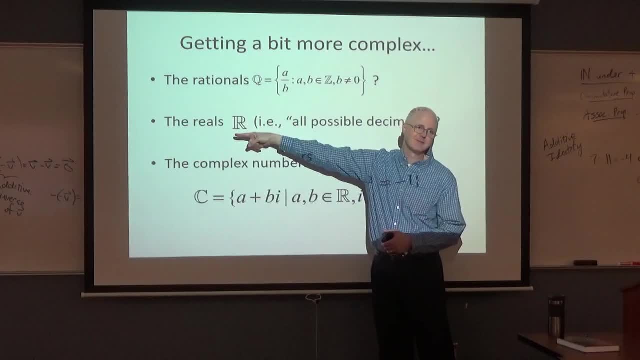 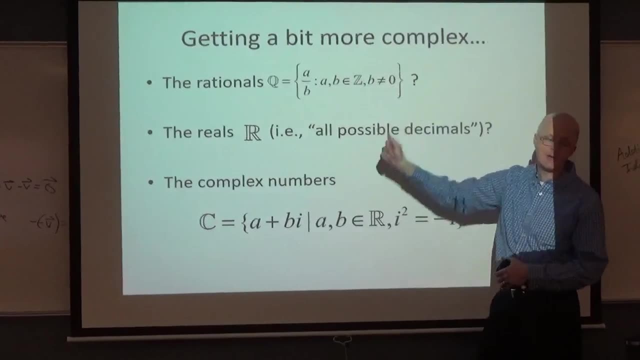 We're saving an r for the reals. Set of all fractions, a over b, where a and b are both integers, and b is not 0, don't divide by 0. 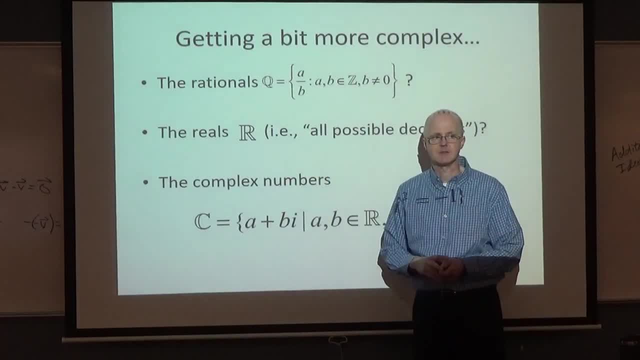 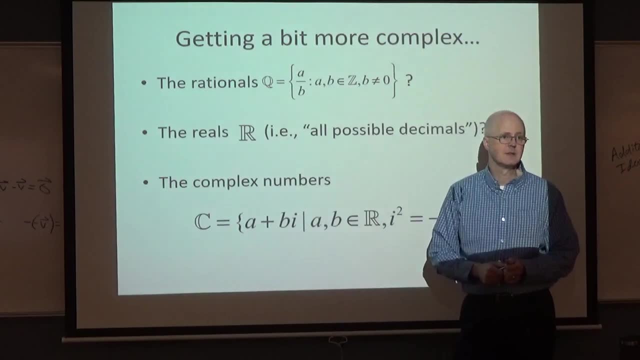 Actually, this is not the best description of the rationals, because it's sort of not taking into account the fact that you can reduce fractions so that, like, you know, 4 sixths is the same as 2 thirds. 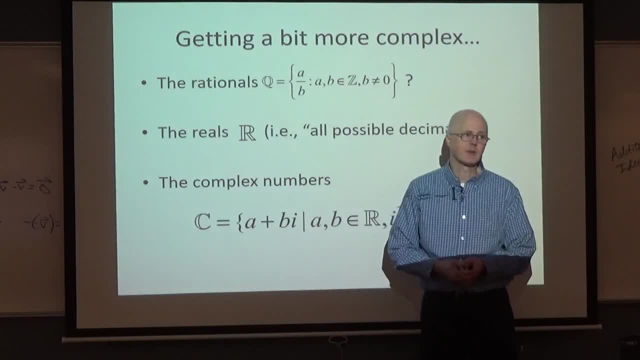 They are equivalent to each other and really represent the same rational number. So this is really not the best way to think about the rationals because of that fact. 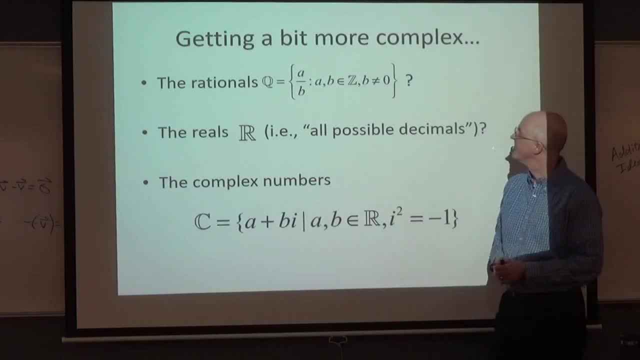 But I think it's, we're not going to worry about that. 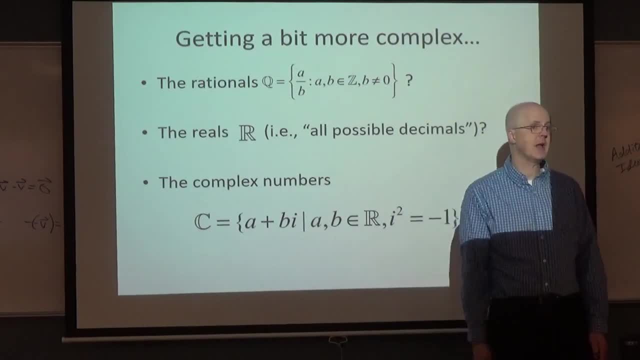 Under addition, you add two rational numbers, you get an irrational number. So it's closed. Right? 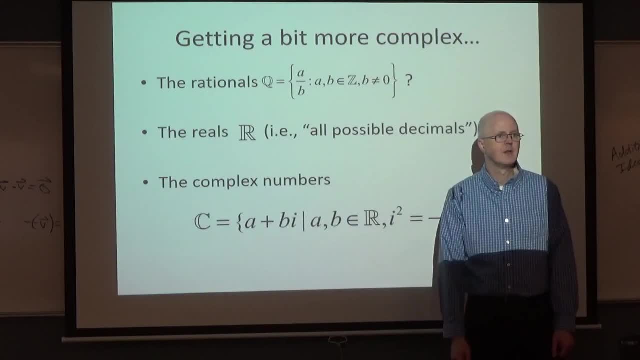 You get a common denominator when you add them. It does satisfy the associative problem. It does satisfy the associative property, still under addition. It still has an additive identity. 0 is a rational number. So that's three things so far. 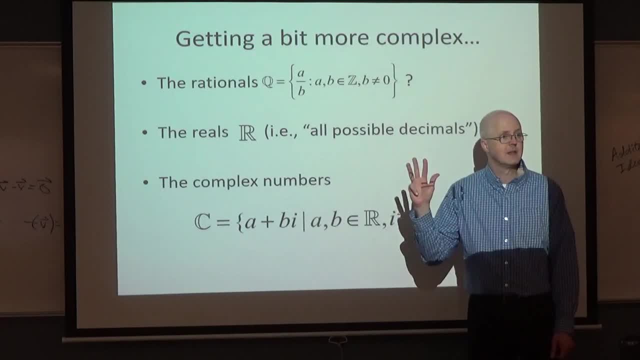 And every rational number has an additive inverse. Q, the rationals, is a group under addition. So is the set of reals under addition. 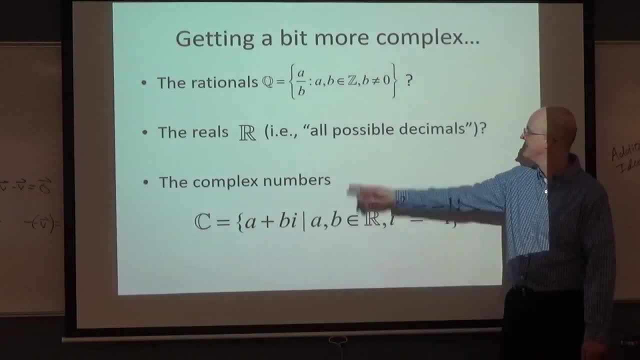 What are the real numbers? Well, they're all the numbers you're used to. You might say all possible decimals. That's not a precise definition. Including decimals that go on forever, either with a repeating pattern or not. 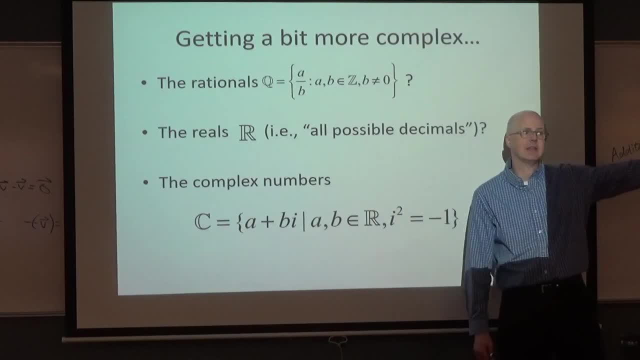 So it includes irrational numbers when we do not have a repeating pattern. You can define addition on the real number system in such a way that it's a group. 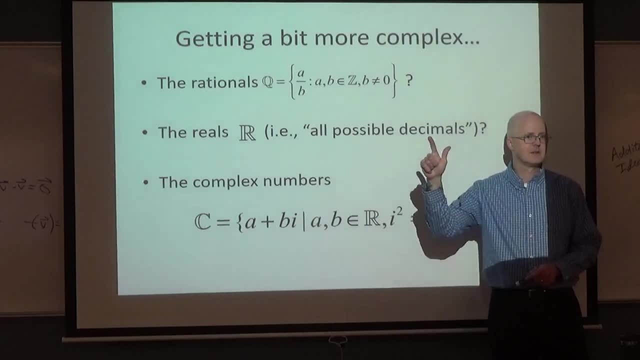 Closure, associativity, additive identity is 0 still. Additive inverses. The additive inverse of pi is negative pi. 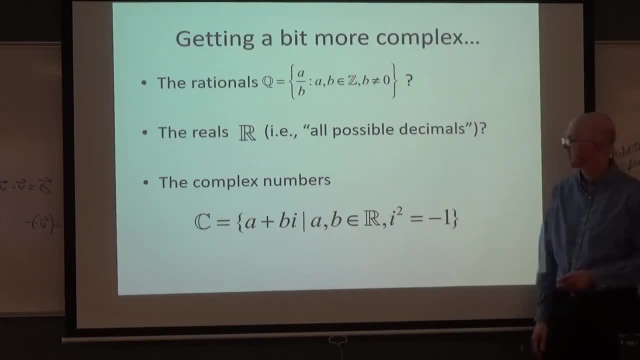 The complex numbers, c, does form a group as well under addition. 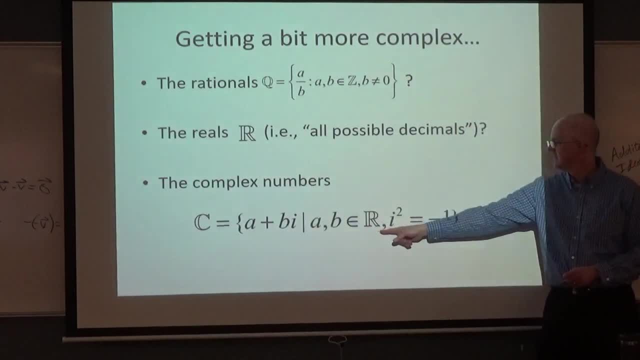 Set of all numbers of this form where a and b are real and i squared is negative 1, right? 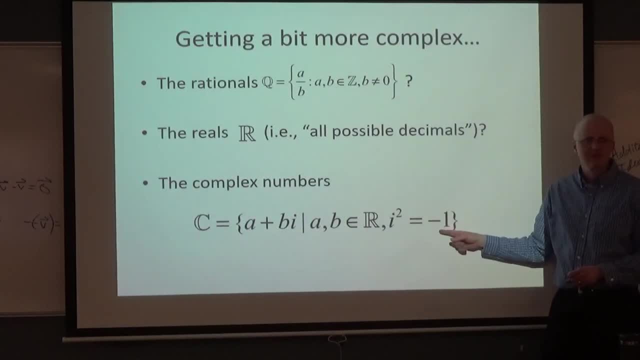 That complex unit. If you took differential equations with me, you know complex numbers are useful in differential equations. That's one example. 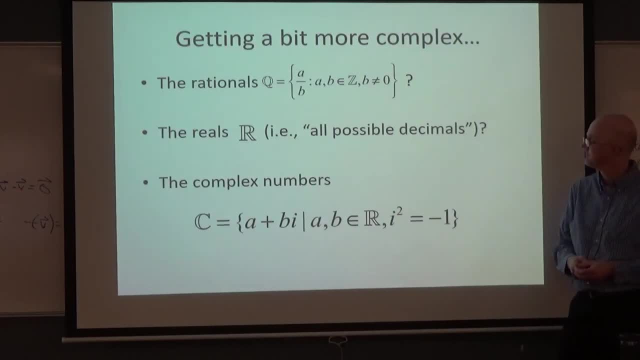 They are useful in quantum mechanics, as I mentioned. 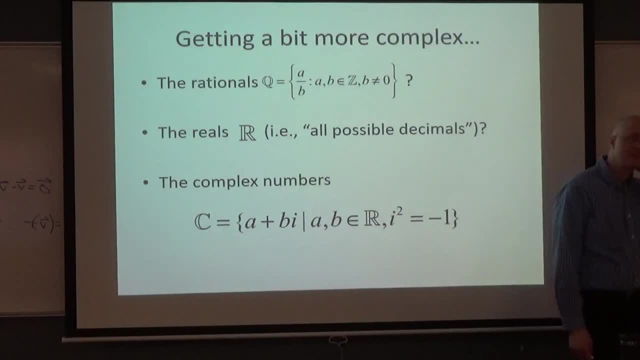 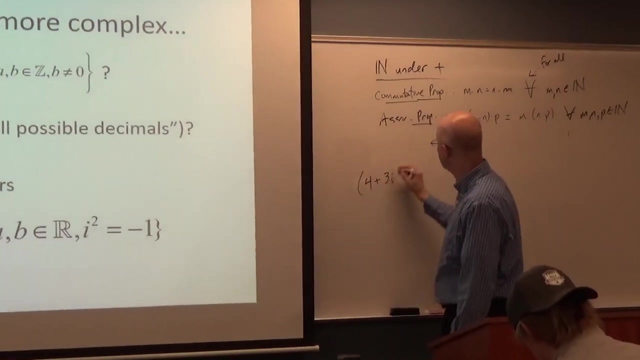 They do form a group under addition. Once again, closure. Associativity. Additive identity, which would be 0. 0 plus 0i is 0. And additive inverses. Of course, you add complex numbers. I hope you've learned this before. It's like 4 plus 3i added to negative 7 plus 2i. 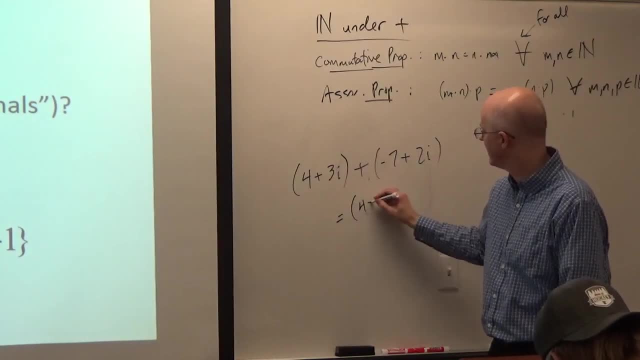 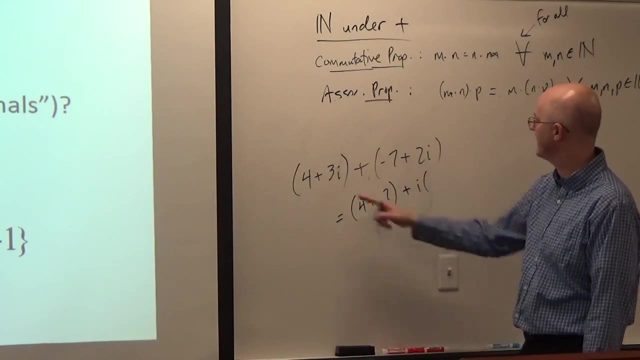 You add two complex numbers by adding their real parts that are not next to the i and then putting plus i times the sum of their imaginary parts, the numbers that are right next to you. 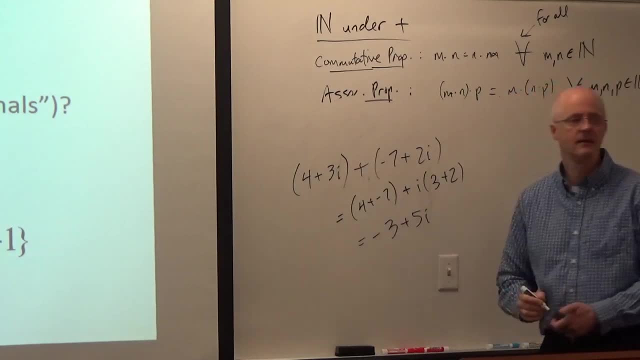 So the sum of these is negative 3 plus 5i. Forms a group. 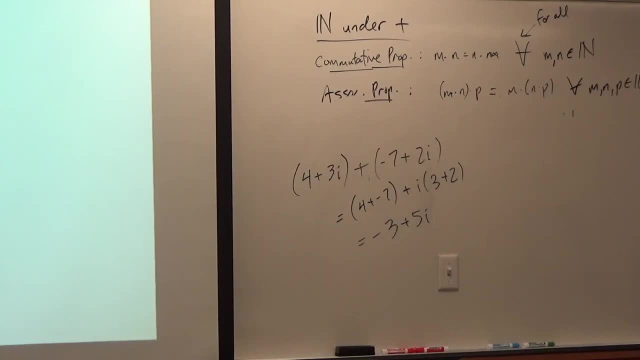 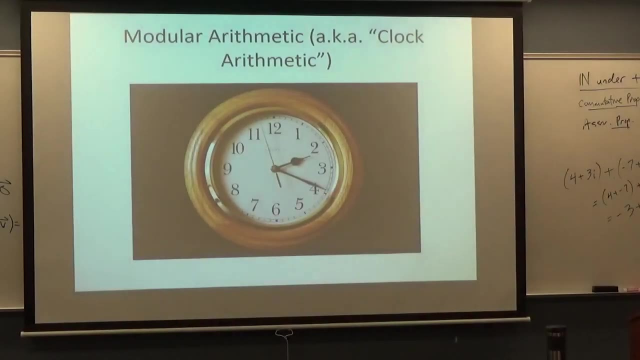 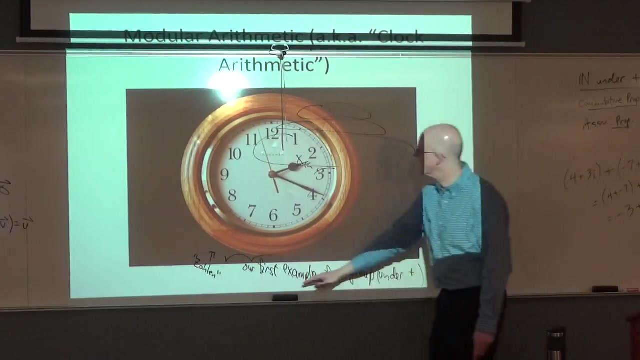 A new kind of group perhaps for you is to consider what's called modular arithmetic, also known as clock arithmetic. 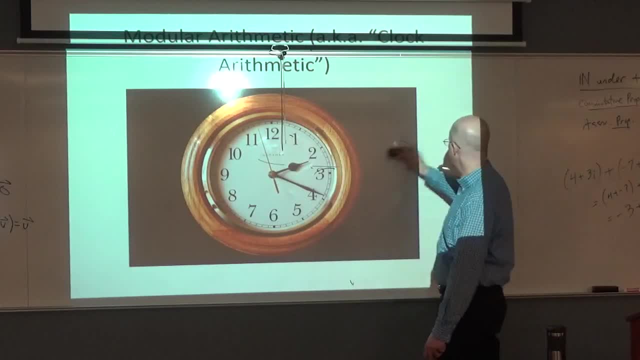 Thinking about your everyday experience, thinking about time. 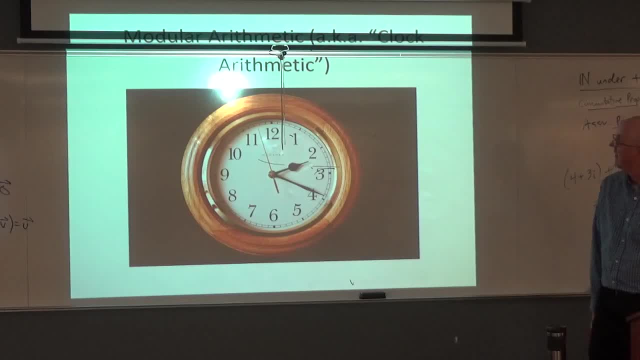 I don't know what time is it here shortly, well, it's about 8.30 right now. 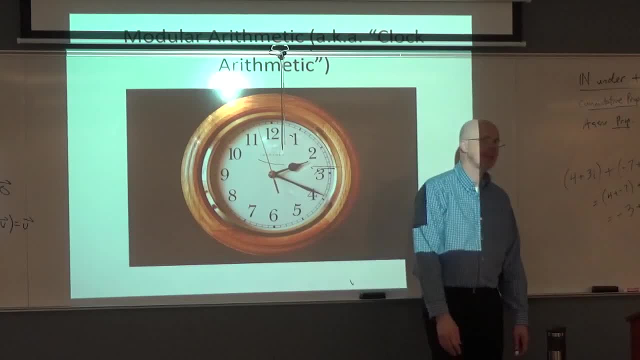 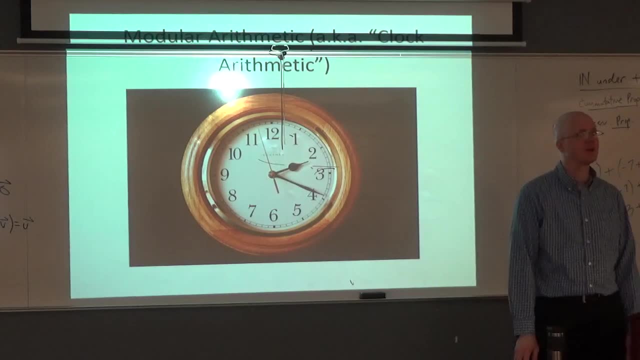 If it were, say, 9 o'clock, and you say, what time is it 5 hours from now? You don't know. It's 2 o'clock 5 hours from 9 o'clock. 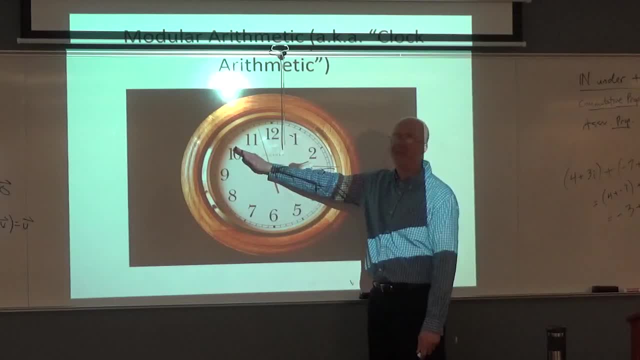 What did you do there? You took 9 and added 5 hours. 1, 2, 3, 4, 5 to bring you to 2. So 9 plus 5 equals 2. Huh? Yeah. 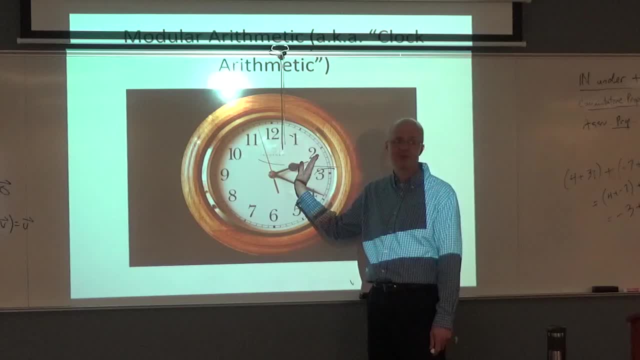 In clock arithmetic. 9 plus 5 equals 2. 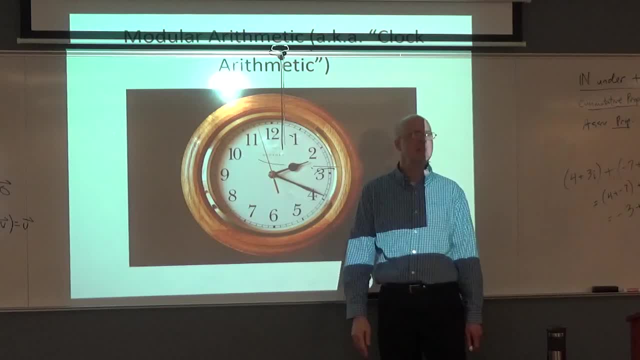 8 plus 17 equals what? Well, there's a trick you can do. 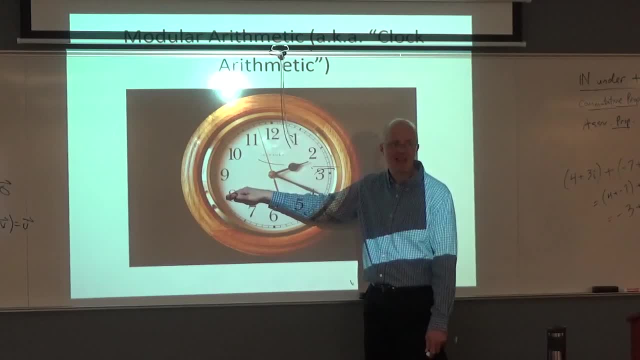 Do 8 plus 12 first to get you back to 8, and then add on 5 more to get you to 1. 8 plus 12 would equal 1. 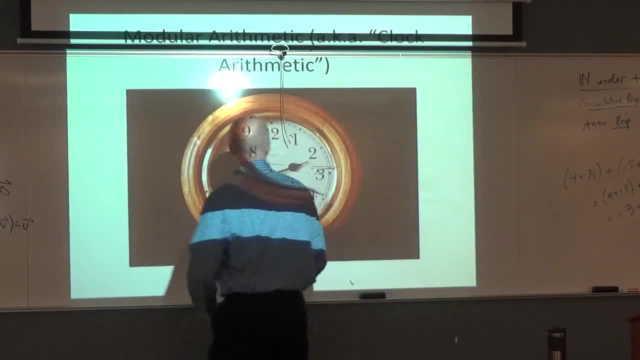 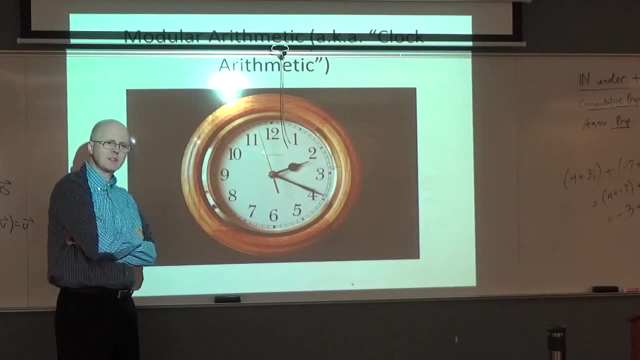 In fact, anything plus 12 brings you back to where you started. 12 is the identity. But wait a minute. 12 is not 0. Well, effectively, in this system, you can think of 12 as being 0, because if you add 0 to any number you're at, you also stay where you're at. 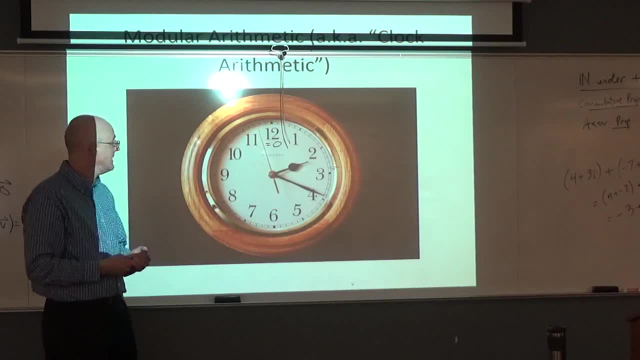 Every number has an additive inverse, too. What's the additive inverse of 8? What added to 8 will bring you to the identity? Negative 8. Negative 8 does. Also, 4. 1, 2, 3, 4 brings you to 12, which is the same as 0. 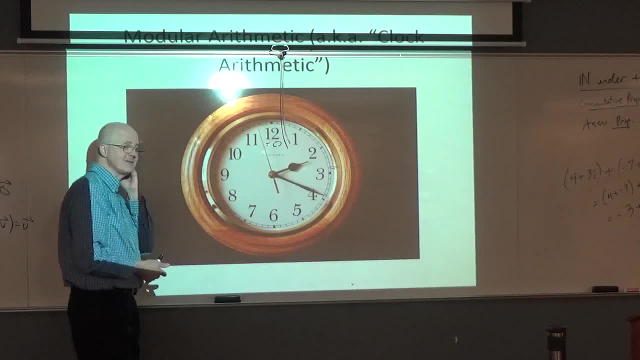 Additive inverse of 4, or let's do 5, is negative 5. You could go backwards, yes. Or 7. 1, 2, 3, 4, 5, 6, 7. 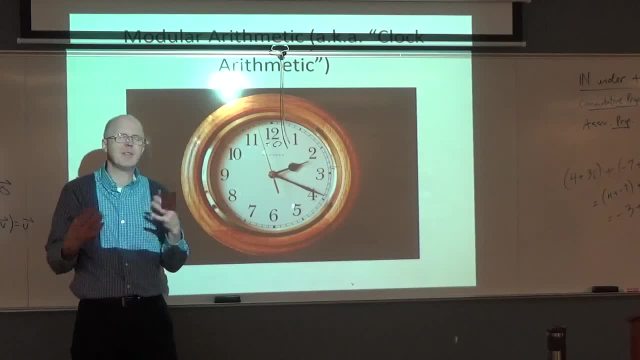 But wait a minute. How can the additive inverse of 5 be both negative 5 and 7, and I suppose maybe 19 and 31? How can you have more than one additive inverse? Is that a problem? Well, yes, technically it is a problem. 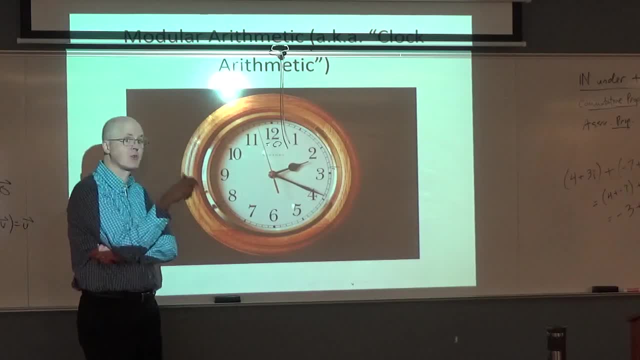 We want to think of those different numbers like 0, 12, 24, 1, 13, 25, 2, 14, 26. We want to think of those as being equivalent. 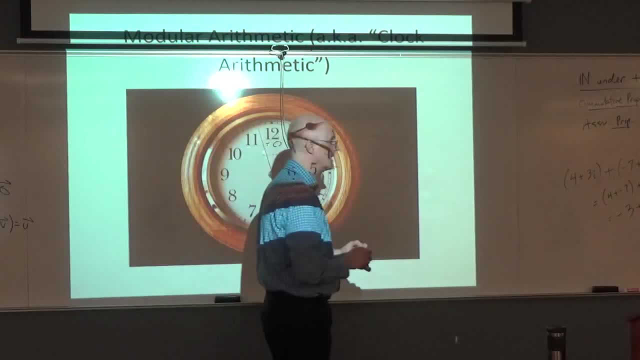 And so we have to bring in the idea of something called an equivalence relationship. But I'm not going to talk about that yet. That's mod 12 arithmetic. 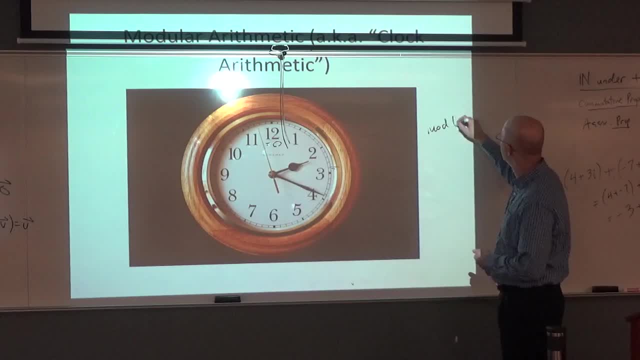 This is called mod 12 arithmetic. Because you've got to think about 12 as the important distinguishing number between these. 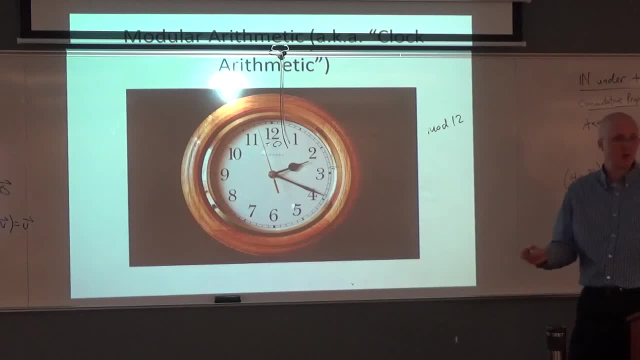 Things are equivalent. 1 is equivalent to 13 because they are 12 units apart. 2 is equivalent to 14 and 26 because those are each 12 units apart. That's why it's called mod 12 arithmetic. There are other kinds of mods you can do, other kinds of clocks. This would be a mod 10 clock. 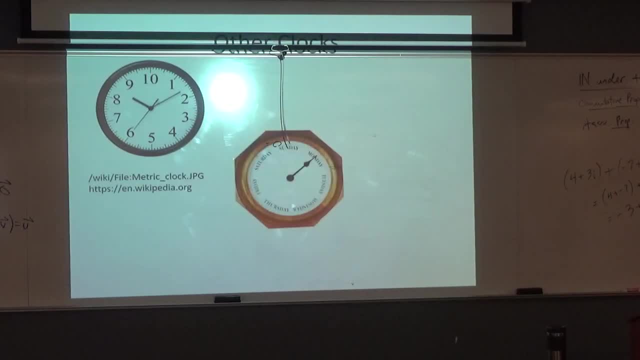 This would be a mod 7 clock. 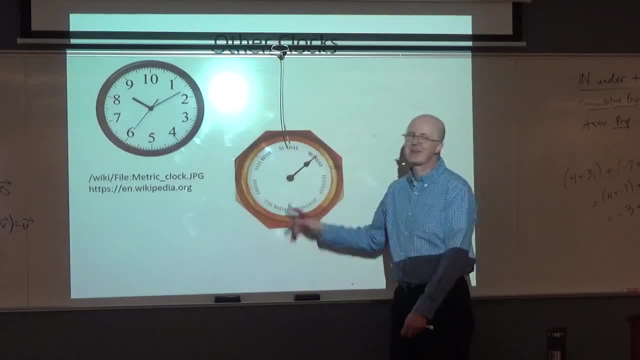 It's not really best to use names of the days of the week. Because what does it mean to add Tuesday to Thursday? Well, what you really mean is if you're at Thursday, you go two more. 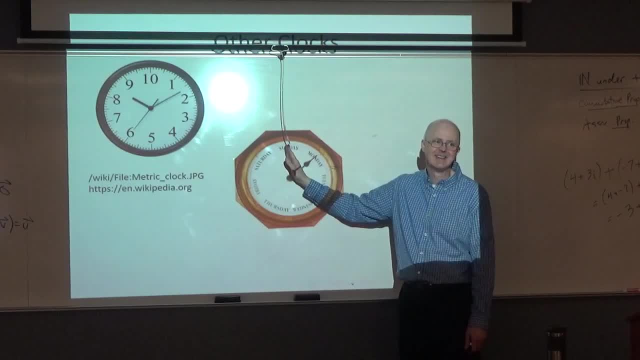 You treat Sunday, since it's at the top, as the additive identity. 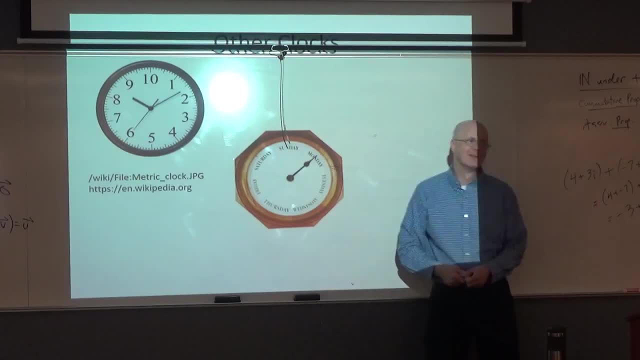 So it would be better to use numbers here. But you get the idea. 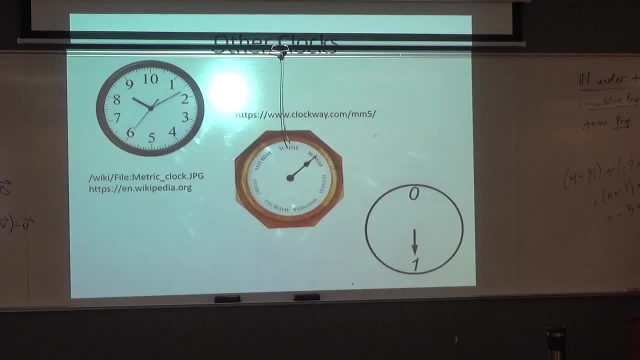 And I made my own little clock here, too. There's a mod 2 clock. 0 and 1. 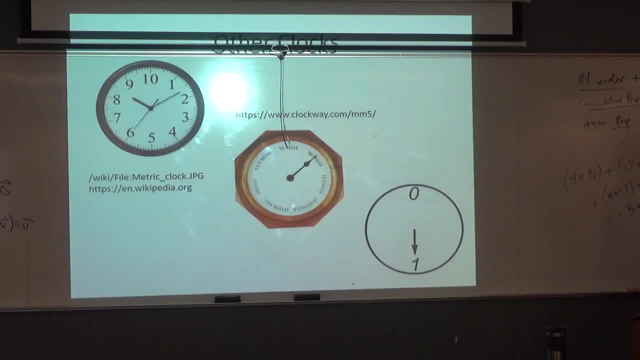 0 is equivalent to all even numbers. 1 is equivalent to all odd numbers. 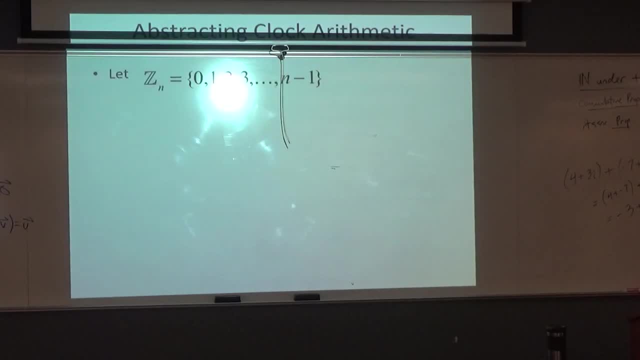 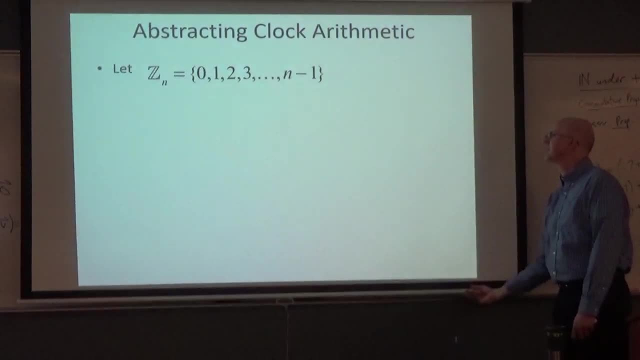 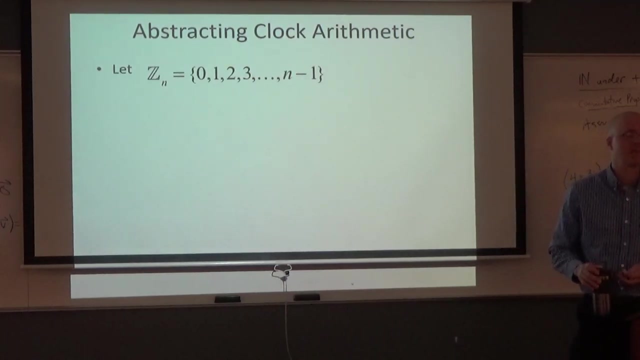 All right, let's get a little bit more official with it. Abstracting this idea of clock arithmetic, we will, in the rest of this course, let z sub n represent the finite set of numbers 0, 1, 2, 3, 4, et cetera, through n minus 1. 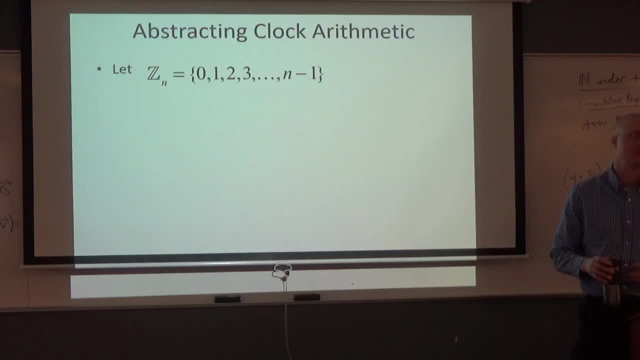 Notice it's got n elements in it. z 10, for example, would be then 0, 1, 2, 3, through 9. 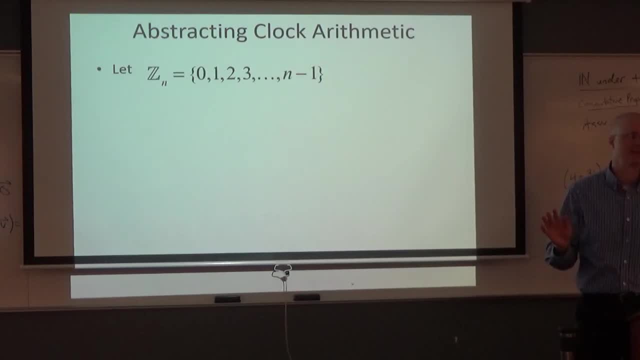 We will use this notation for the rest of this class. That's what z n always represents. 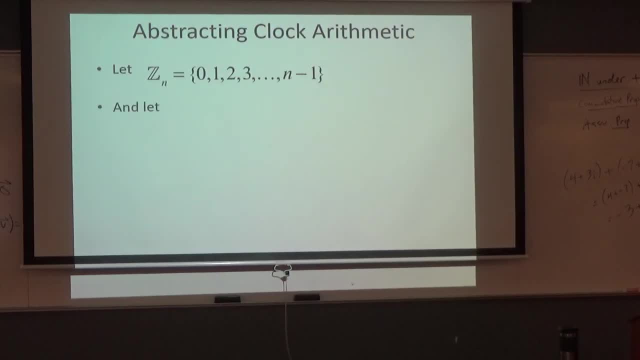 It's going to be one of our favorite groups, ultimately, here. 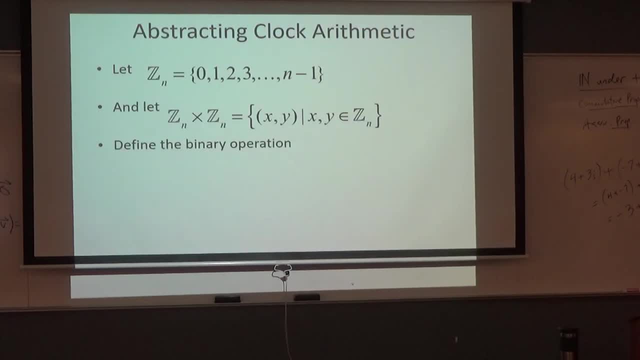 We can define a binary operation on z n after first defining what's called the Cartesian product of z n with itself. 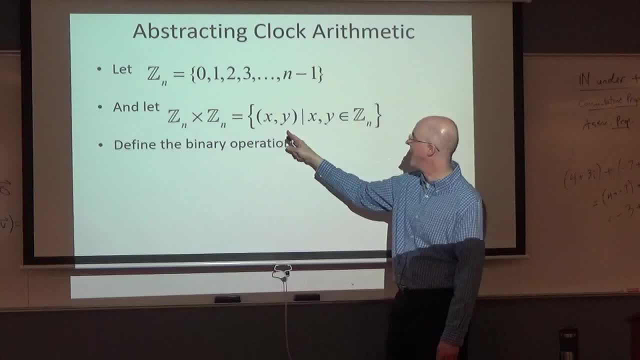 z n cross z n is the set of all ordered pairs, x comma y, where x and y are both elements of z n. By the way, I haven't said this yet. 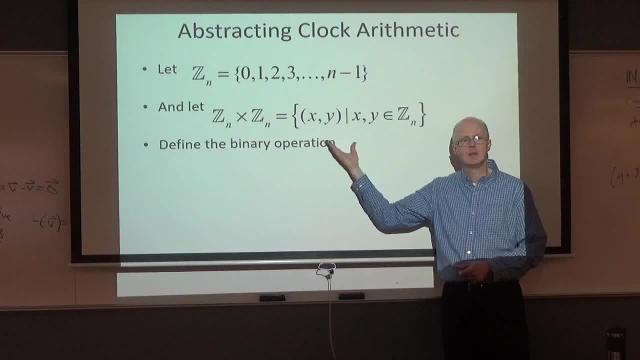 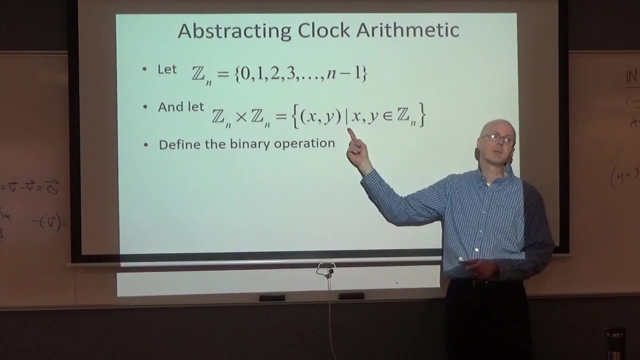 This is called set-builder notation. You want to get used to this. You read this as the set of all ordered pairs, in this case, x comma y, with the property that or such that. Think of this vertical line as representing with the property that or such that, for short. 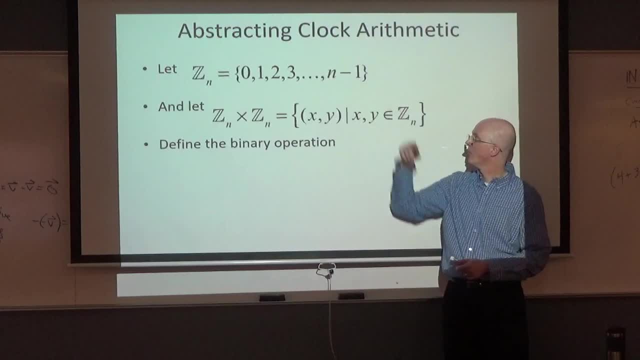 x and y are both elements of z n, so they are one of those numbers. 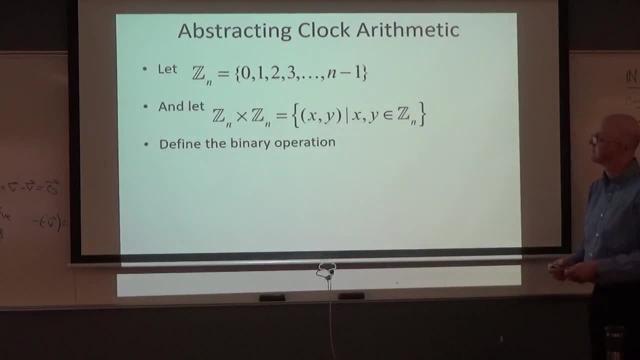 It's called the Cartesian product of z n with itself. Officially, binary operations are functions from the Cartesian product to the original set. 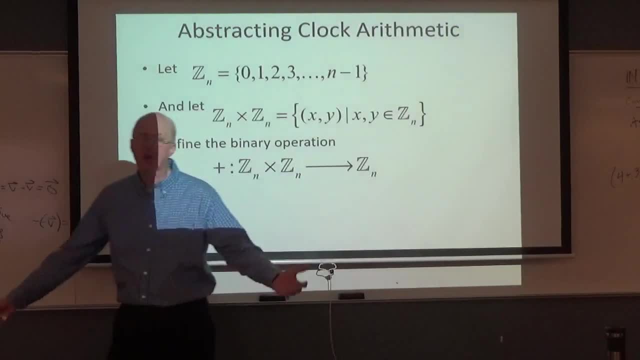 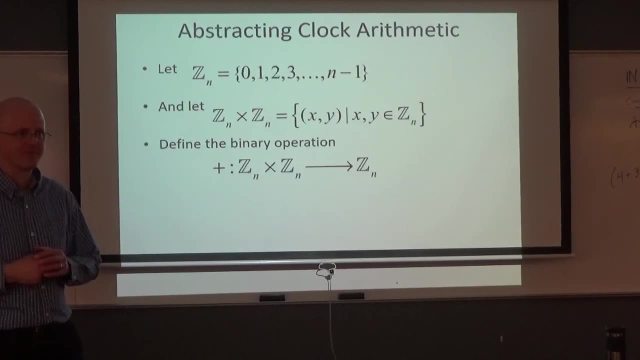 So I'm using this plus here as the function name for this binary operation, which is not something you're used to. 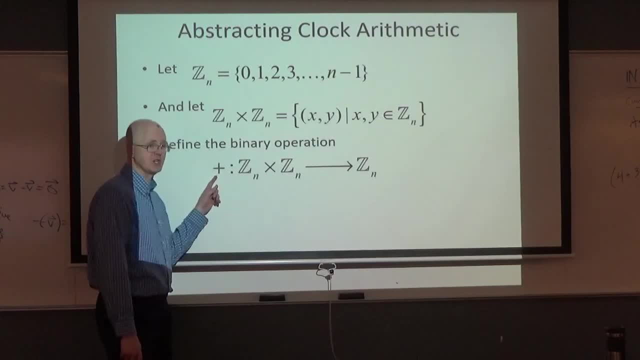 This notation means this is the function. 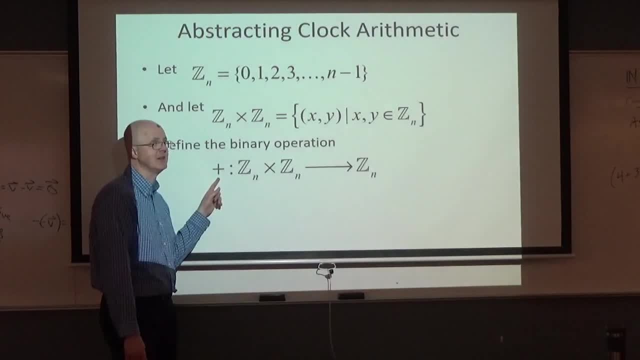 Plus is the symbol for the function here. That's going to represent addition, mod n ultimately. 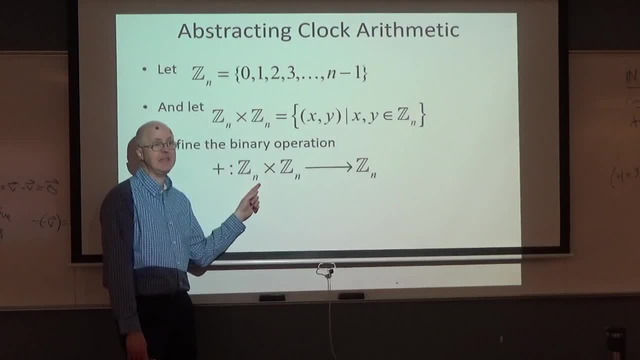 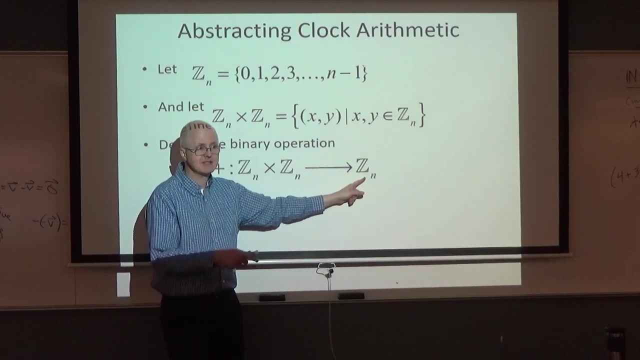 This is its domain. Inputs for this function are ordered pairs of elements from the set. I'm going to call this a codomain, which is consistent with your linear algebra book, but not consistent with this book, although actually in earlier editions it was. 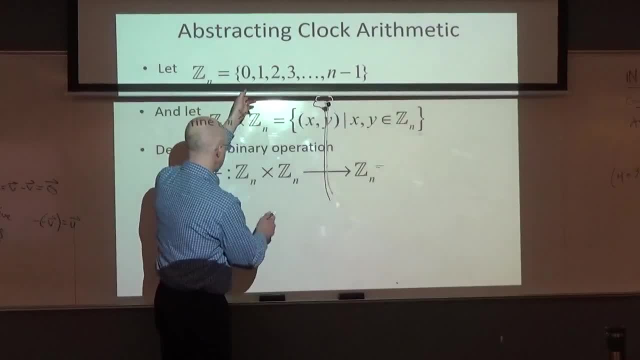 I'm going to call this the codomain. This is a function here 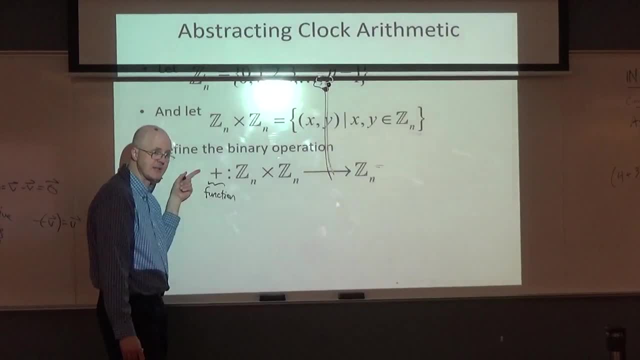 that I'm labeling with the symbol plus because it's going to represent addition. 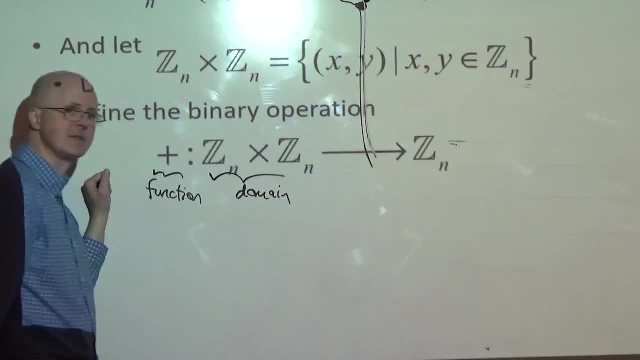 This is the domain of the function, the set of all the inputs. 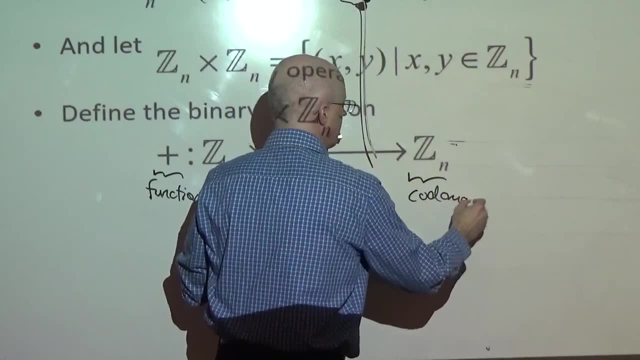 This I will call the codomain. Some people call it range instead, but I'm going to leave the word range for something else. 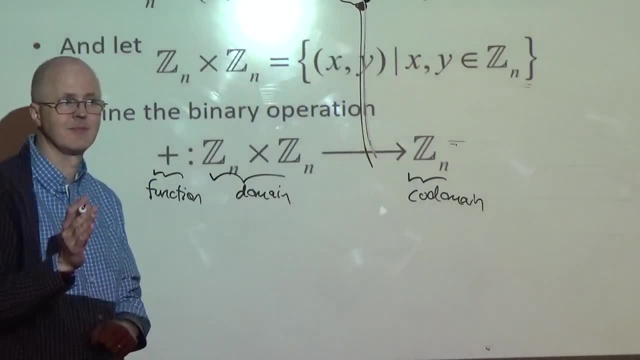 Actually, I'm going to mostly avoid the word range. I'll use the word image. 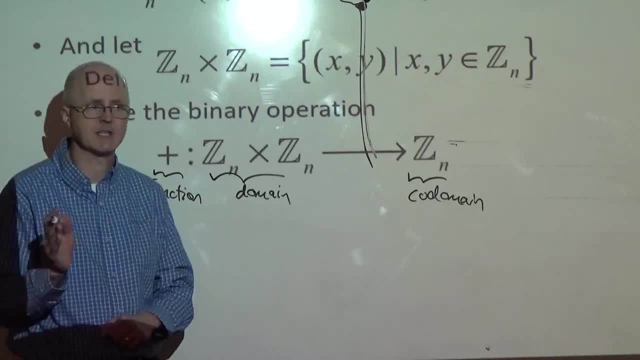 I like avoiding the word image, except to say in pre-calculus courses. 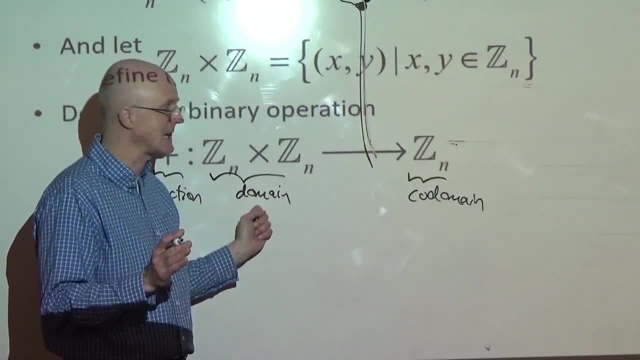 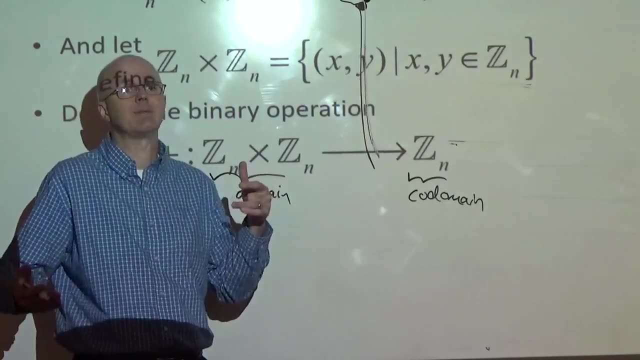 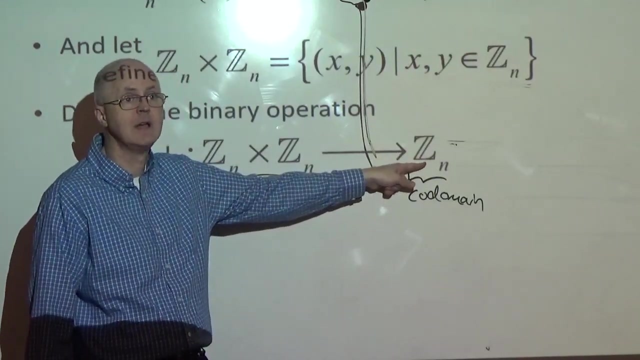 That's the set of all inputs. This is not necessarily the set of all possible outputs in general. It's just the target space. It's the set where the outputs live, so to speak. The outputs are elements of the set, though you don't necessarily in general have all those elements as possible outputs. 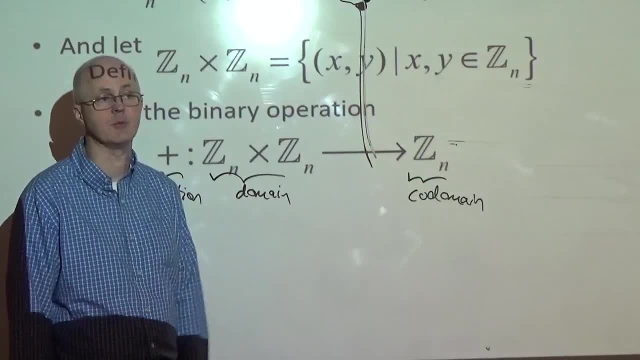 The function is not necessarily onto, but this one is. 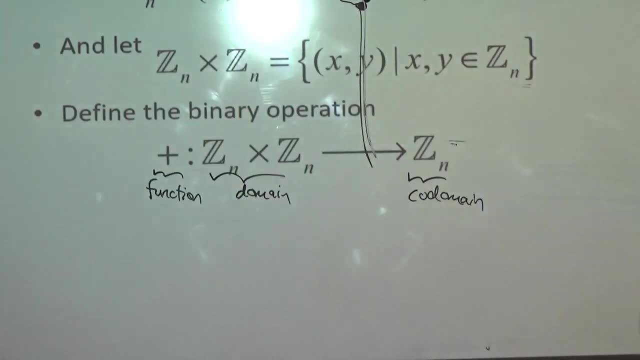 And what does plus do? Well, it adds numbers in Zm. Mod n. 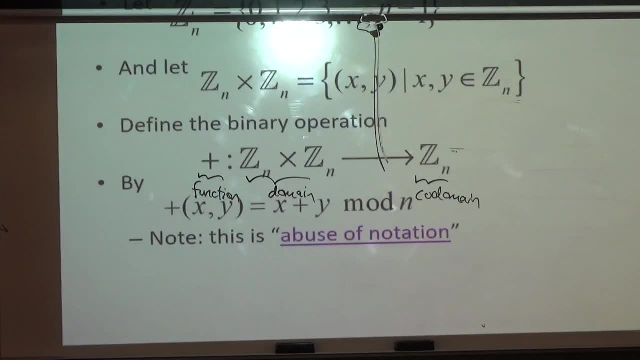 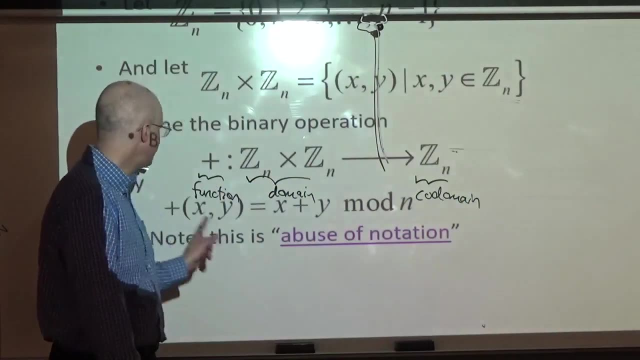 Technically speaking, I am abusing notation here. I'm using this plus symbol in two different ways, both as a function name and in the ordinary way. Abusing notation. 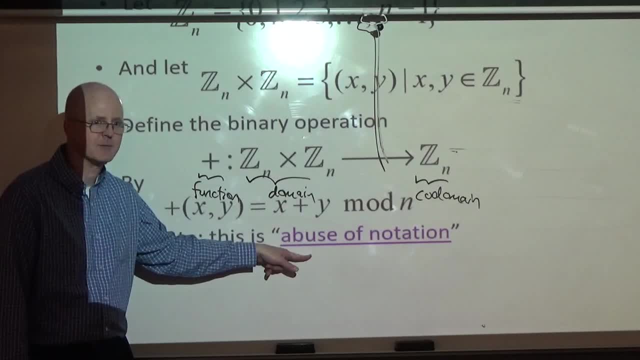 The main thing with abusive notation is just not to let it bother you. Just get used to it. It's okay. 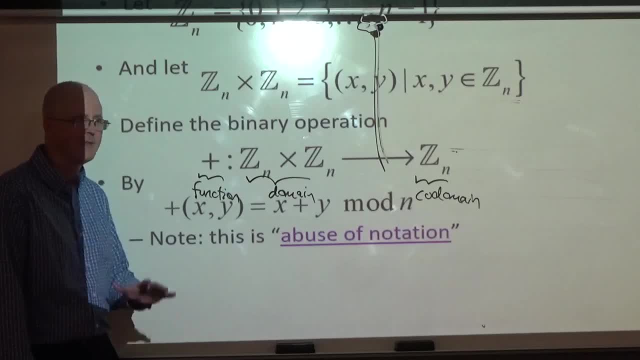 Don't worry about it too much. Probably, if I was going to try to avoid abusing notation, I'd use a different symbol here for the function name. Maybe I'd call it F sub plus or something like that. 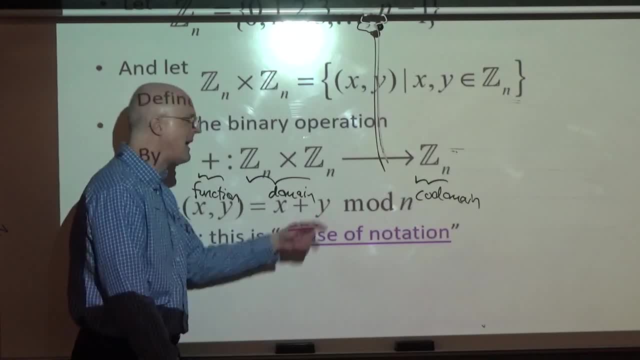 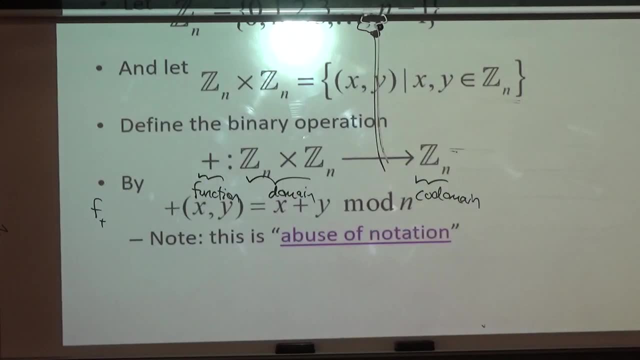 What does mod n mean? It means find out what x plus y is equivalent to mod n, meaning find the remainder when x plus y is divided by m. 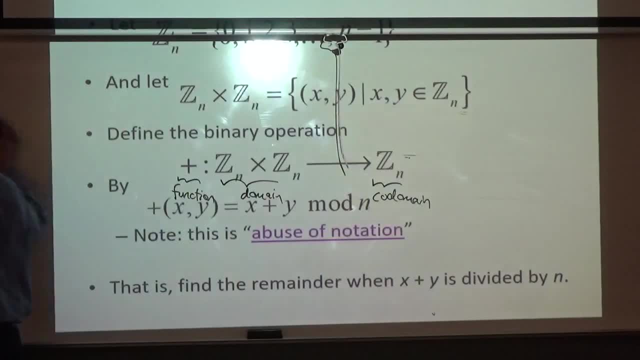 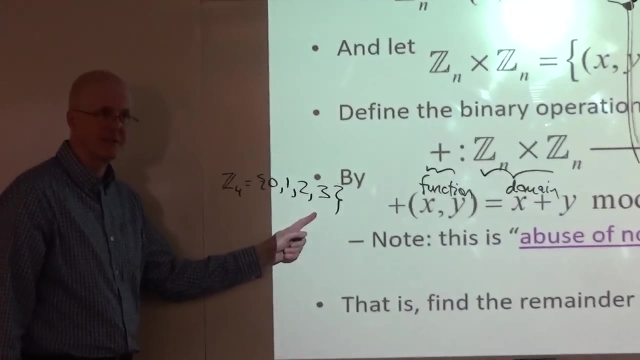 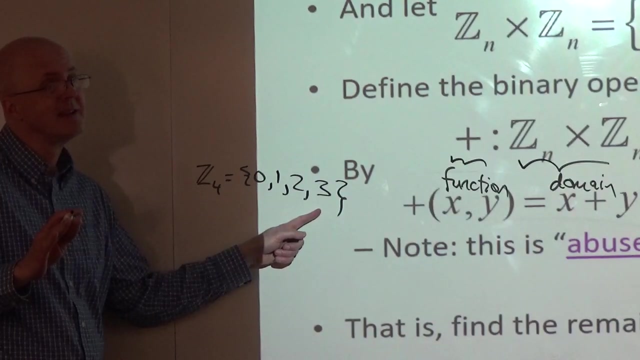 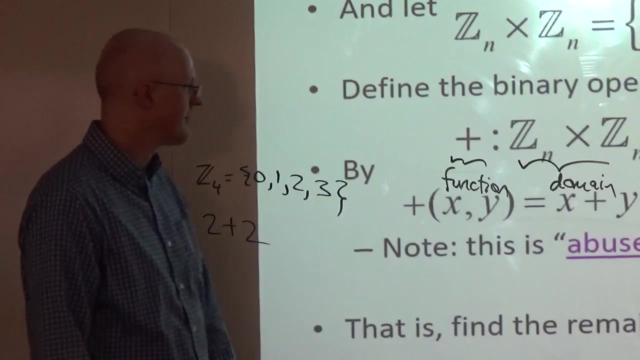 That's what mod n ultimately really means. So, for example, if I'm talking about Z4, which consists of those four elements, those four numbers, 0, 1, 2, and 3, not 4, though 4 is equivalent to 0 in a sense. And I want to, for example, do 2 plus 2. Mod 4. The answer is, what is the remainder when 2 plus 2 is divided by 4? The remainder is 0. 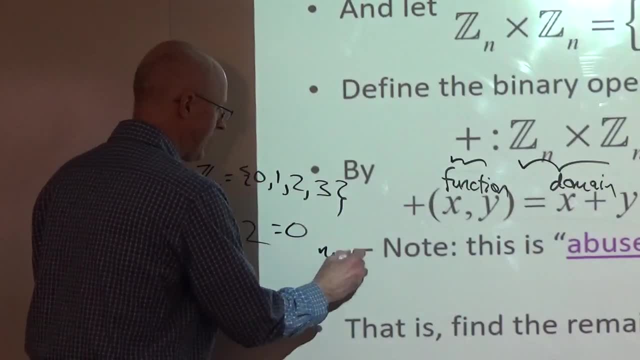 2 plus 2 equals 0. Mod 4. 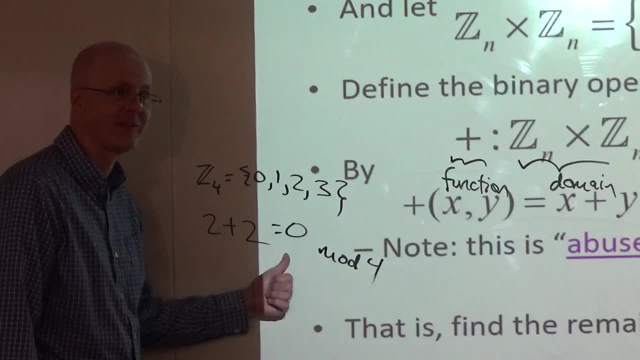 And you can go home and tell your parents, guess what I learned in math today? 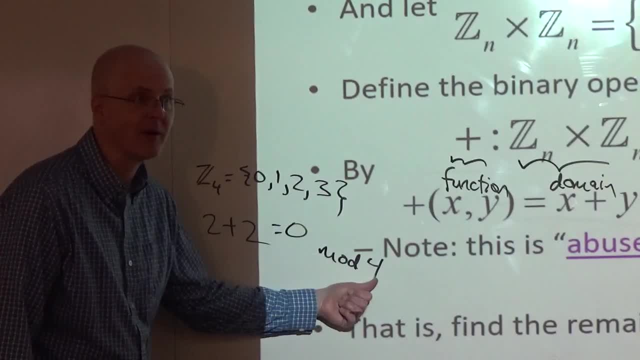 2 plus 2 equals 0. Well, you should add the caveat, mod 4. 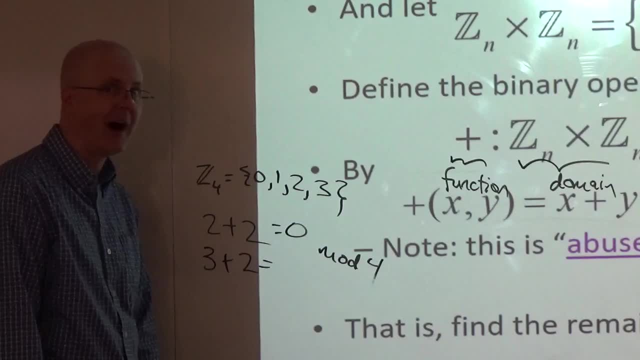 3 plus 2 is 5. But what is 5 mod 4? What's the remainder when you divide 5 by 4? 1 mod 4. 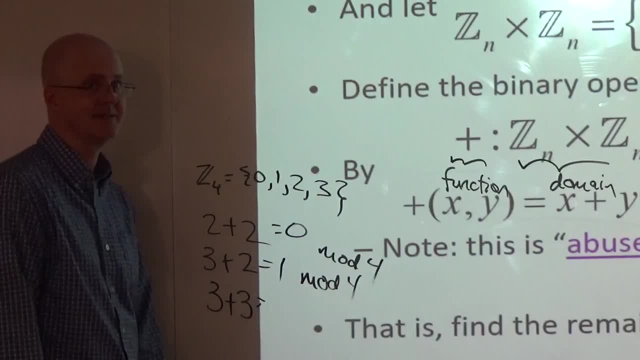 3 plus 3? 6. 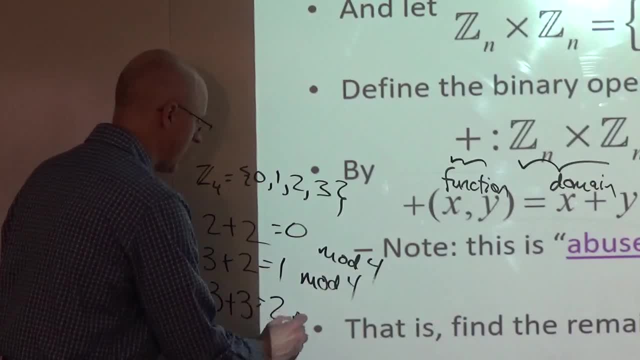 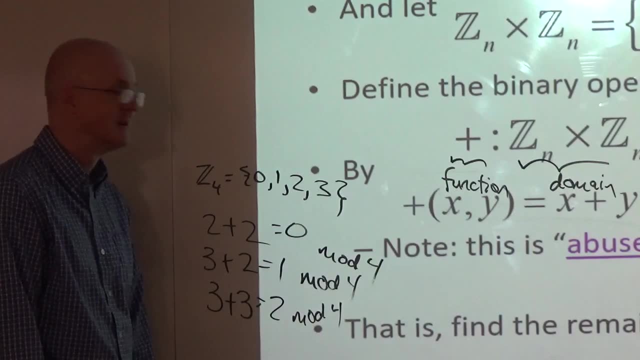 Divide 6 by 4, you get a remainder of 2. This is 2 mod 4. 0 is the additive identity. The additive inverse of 2 is itself, because 2 plus 2 is the additive identity. 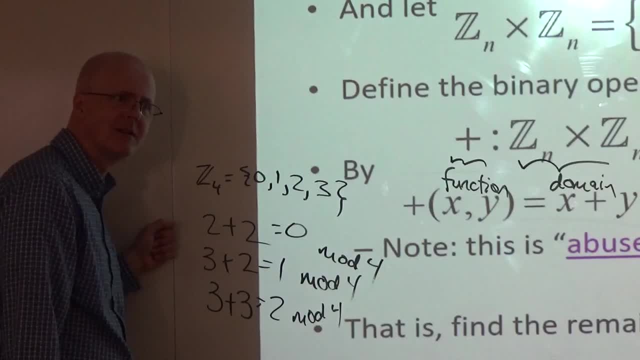 What's the additive inverse of 1? Which of these can you add to 1 to get 0? 3. 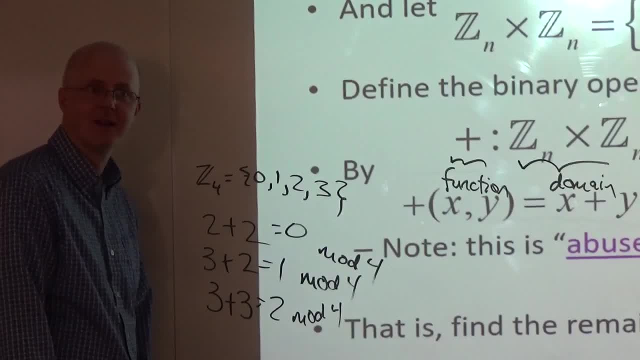 3. 1 plus 3 is 0. Mod 4. 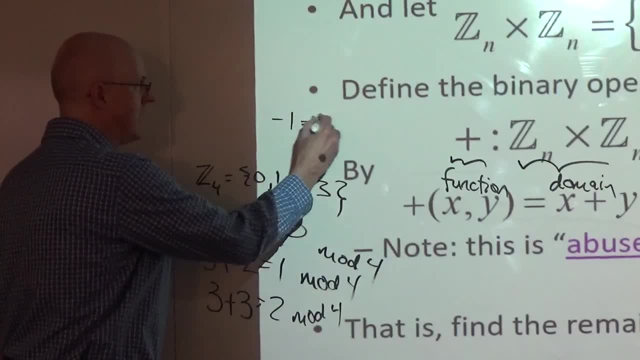 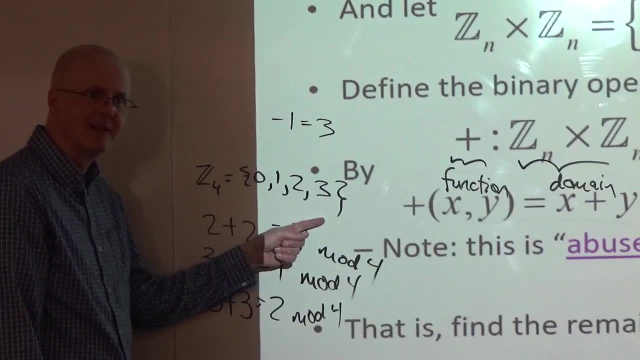 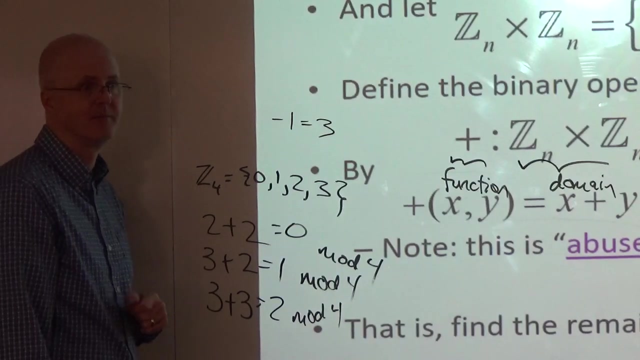 The additive inverse of 1 is 3. You can maybe write negative 1 equals 3 mod 4. Maybe that makes sense, although negative negative 1 is not part of the set, though it is a notation you could use for the additive inverse of 1. Please stop me if you've got questions, okay? Feel free to stop me. 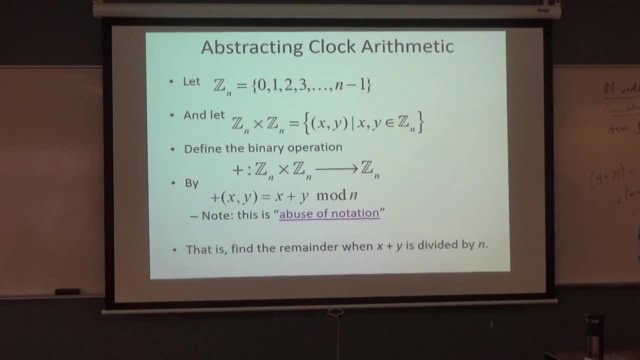 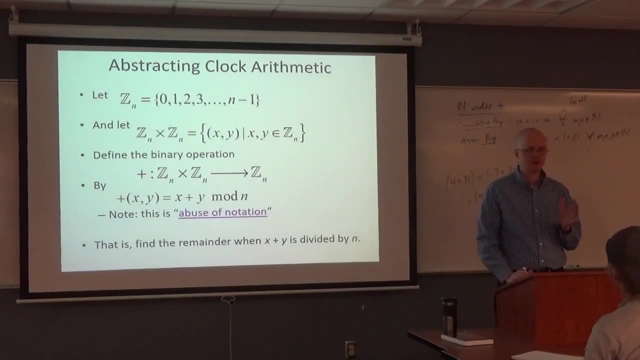 I've got about 10 minutes left here. You know, I have goals as far as how far we want to get, but I don't want those goals to override your understanding. So, you know, we can flex as far as how fast we go to a certain degree. So if you feel confused, I do want you to stop me and ask me to re-explain something, okay? Probably I will generally have more slides than I can get to. 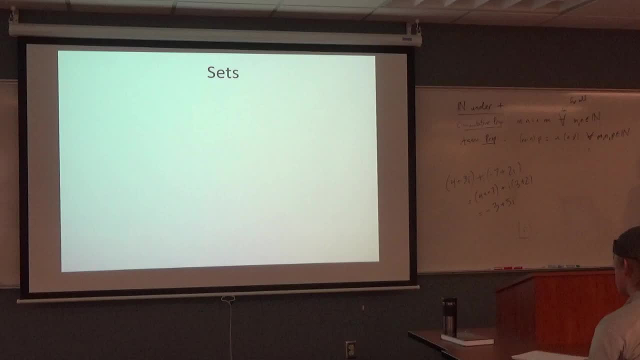 I think that's the case here. I think we're going to finish up talking about sets and functions fairly quickly. 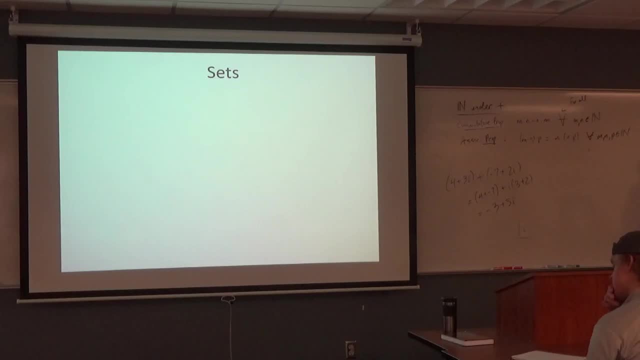 There's an idea of equivalence relations at the end of this set of slides. I'm going to go fairly fast through this so we can get through the idea of sets and functions. 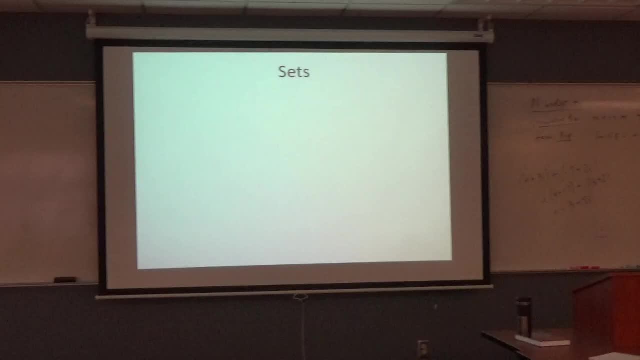 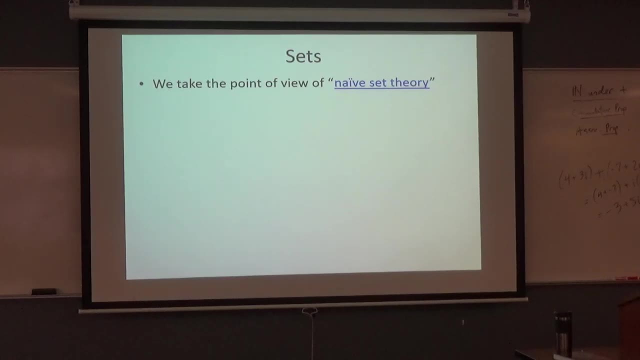 Technically speaking, this is stuff you probably have seen before. We're going to take the point of view of what's called naive set theory, and that's got its own Wikipedia page, as that link indicates. What in the world is naive set theory? Well, basically it's not a very good set theory. 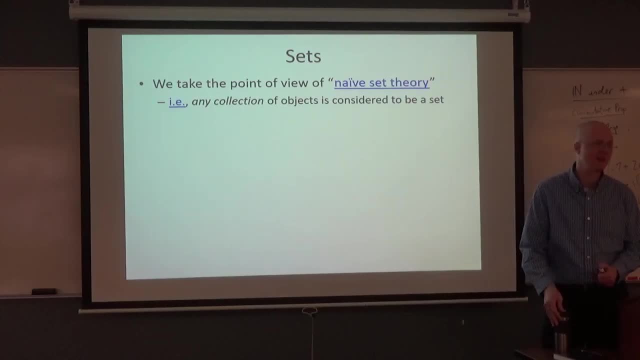 It's where we take the idea that a set is just any collection of objects. It could be a collection of numbers. It could be a collection of words. It could be a collection of people. It could be a union of those things. It's just any collection, okay? That actually leads to trouble. Naive set theory leads to paradoxes. And so it's not the best kind of set theory. 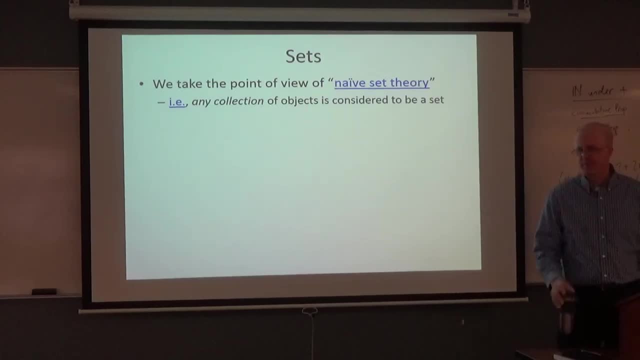 There's an axiomatic set theory that's better. But it only leads to trouble. 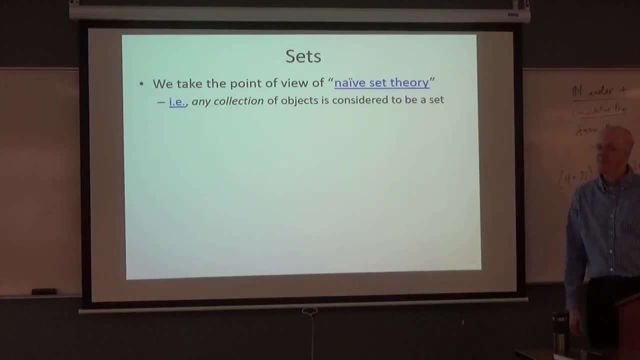 It only leads to trouble when you start thinking really, really high level about stuff. 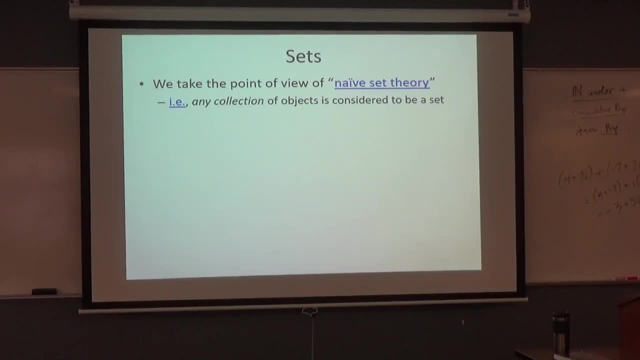 Well, okay, you can say it's basic, but it's not going to bother us. Let's just put it that way. 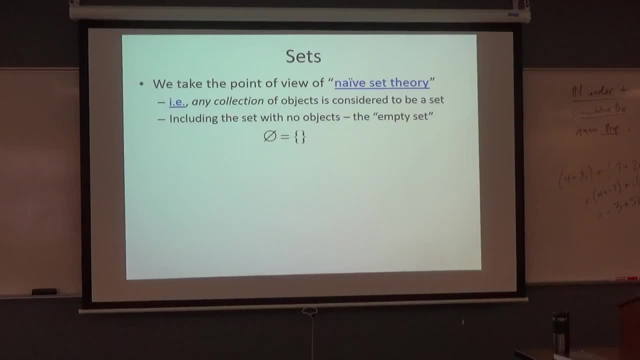 That includes the set with no objects called the empty set, which you can use either of these notations for. An O with a slash through it. It's not the number zero there. 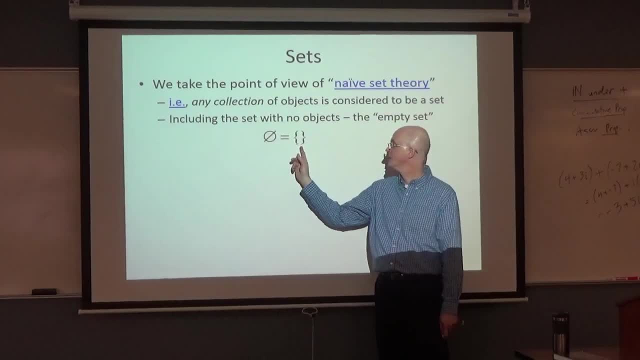 It's an R with a slash through it. It represents the empty set. It embraces with nothing inside. That can represent the empty set as well. Both are standard notations. You don't have to use both notations. You can just use one or the other. 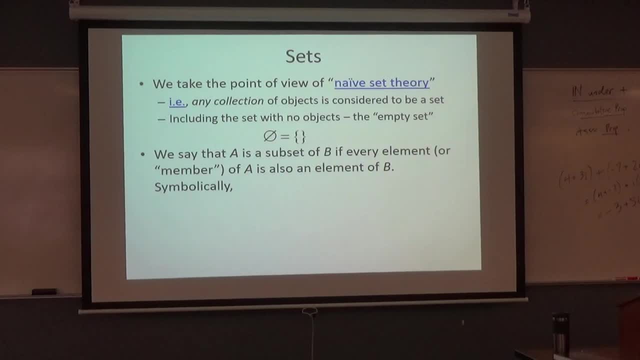 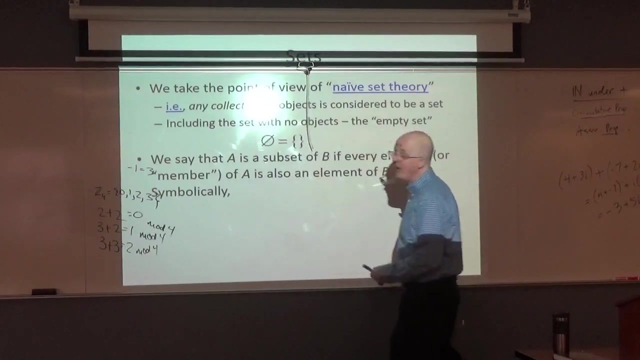 We say A is a subset of B if every element of A is an element of B. Symbolically, well, okay, before we look at the symbols for this, let's just draw a picture of Venn diagram. 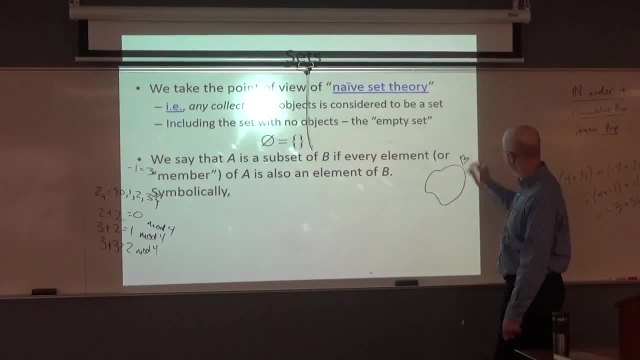 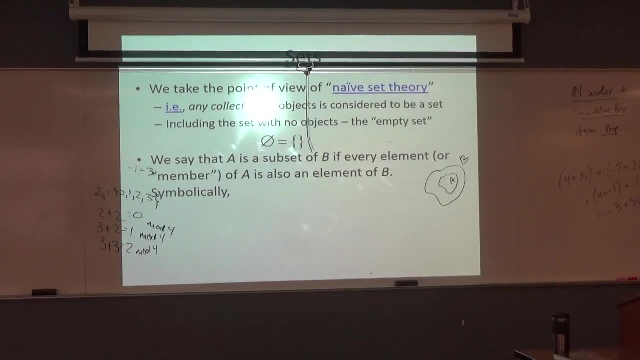 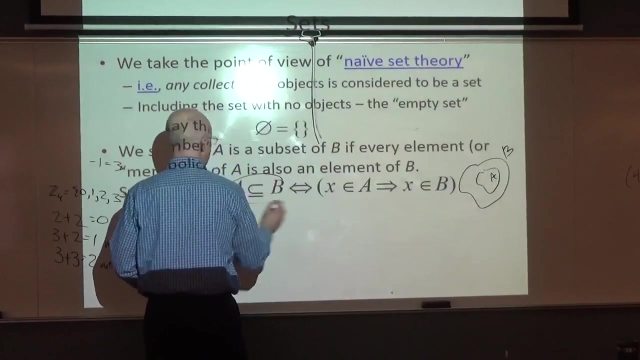 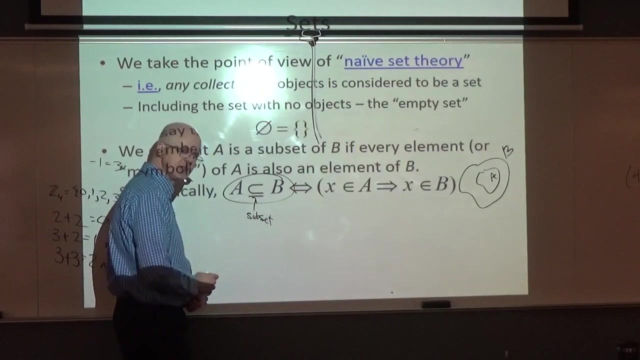 In Venn diagram, you might say if this is B, then A has to be inside B to be a subset. Symbolically, though, we've got to be a bit more official about it. A is a subset of B. This is subset notation. Actually, more officially, you should say subset or equal to perhaps, though. Subset means it could be equal. You will see some people just putting this instead for short. This is technically better because it allows for the equality. 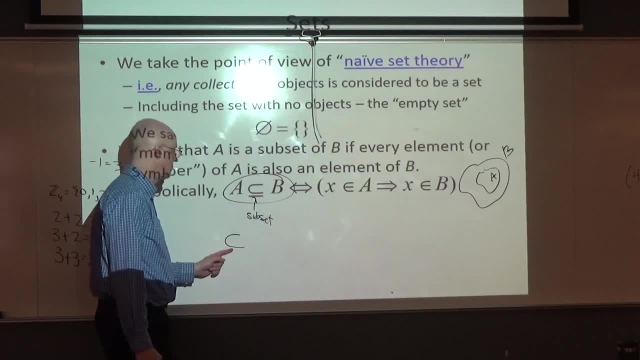 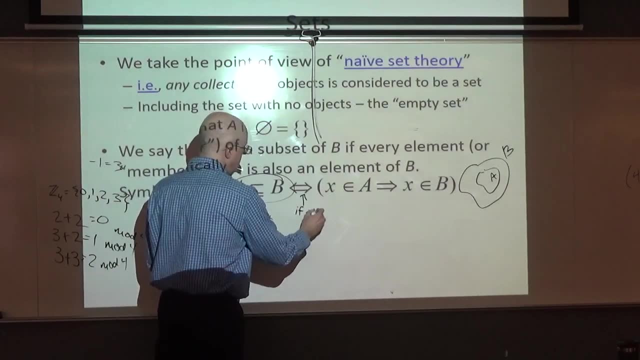 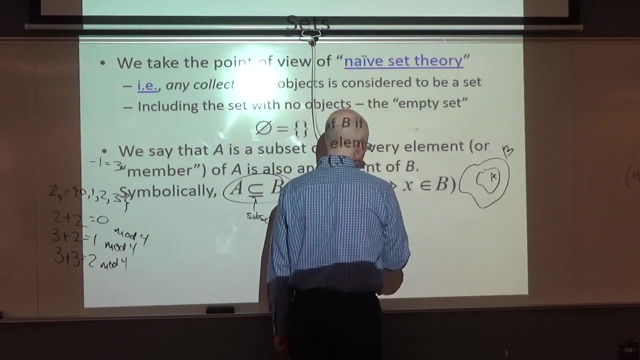 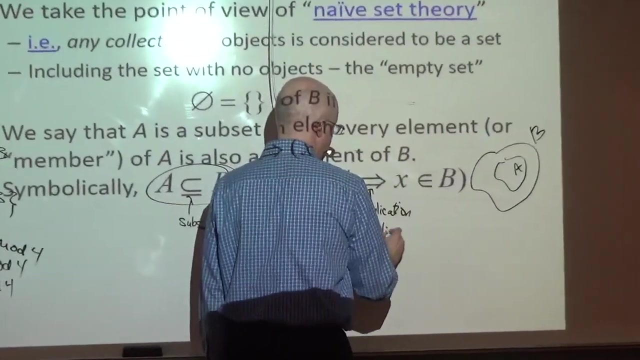 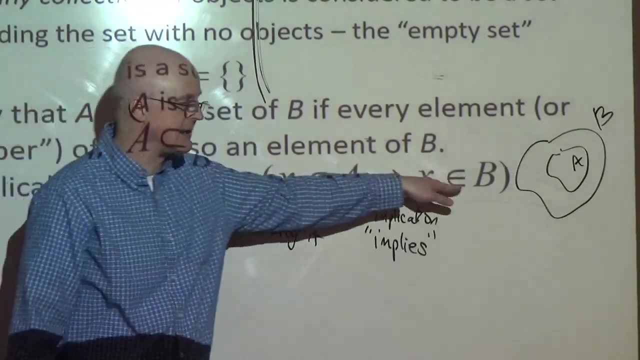 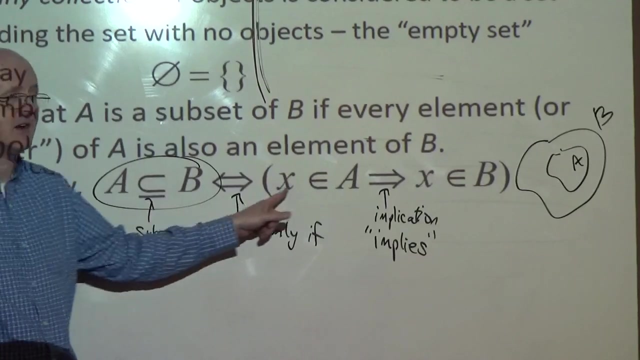 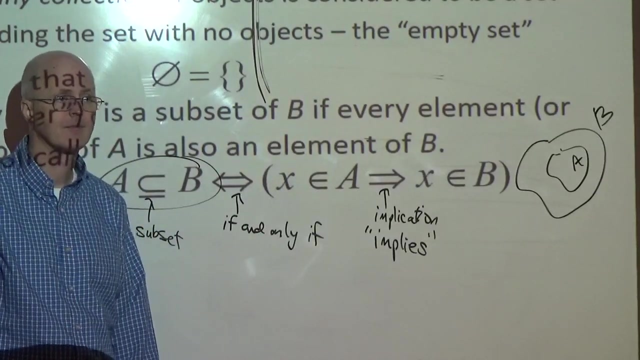 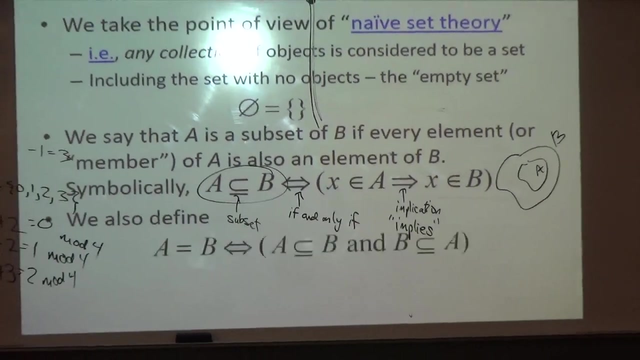 But when people use this, they sometimes still mean it could allow for equality. Arrow pointing both ways essentially means if and only if. In arrow pointing one way like this, this is called an implication. You can think of it as the word implies for short. If you're given X in A, that automatically implies X is in B. That's what it means for A to be a subset of B. That means to prove that A is a subset of B, you have to say, give me an arbitrary element of A, and you would need to show it's in B. Two sets are equal if they're both subsets of each other. 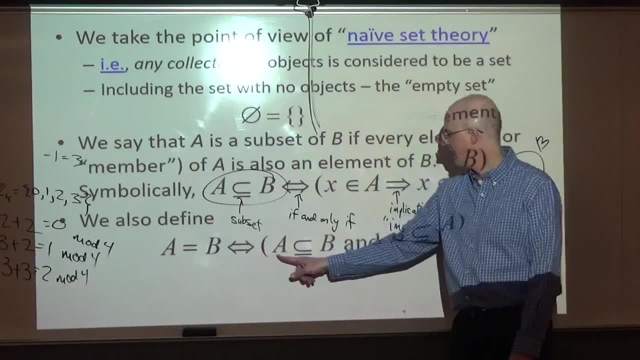 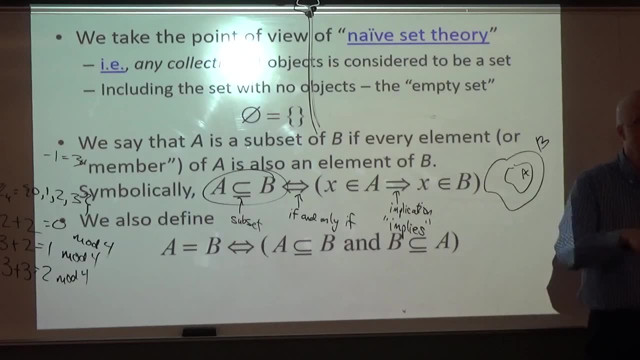 A equals B if and only if A is a subset of B and B is a subset of A. To show two sets are equal, you need to show A is a subset of B and B is a subset of A. 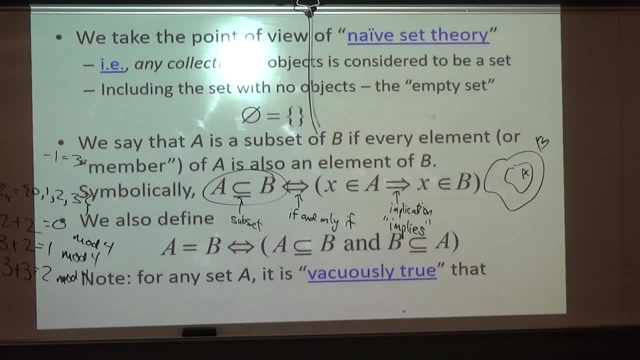 Here's something important to note. For any set A, it is vacuously true that the empty set is a subset of that given set. The empty set is a subset of everything. Of every set, I should say, including itself. Essentially, it satisfies this implication because if A is the empty set, this part of the implication is false. 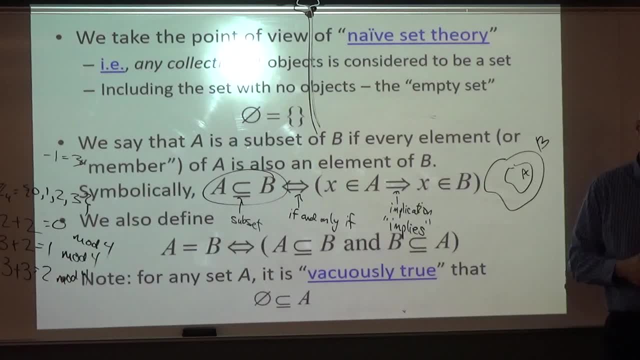 Making the implication true, you might have learned about truth tables in discrete math. P implies Q. 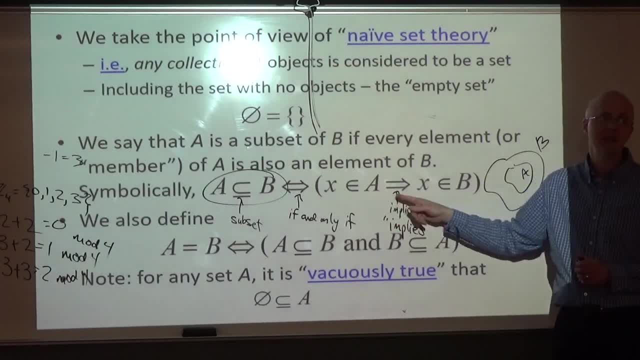 When P is false, the implication P implies Q is true no matter whether Q is true or false. 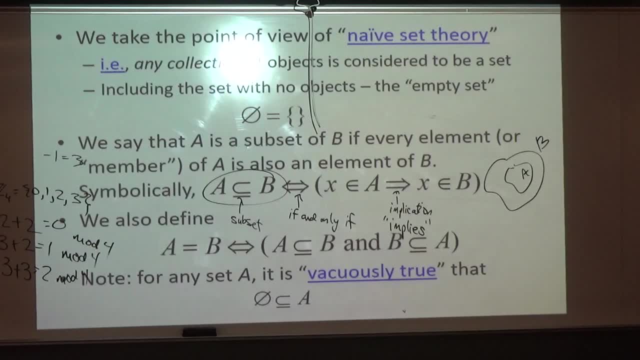 Kind of a weird thing, but just know the empty set is a subset of every set. 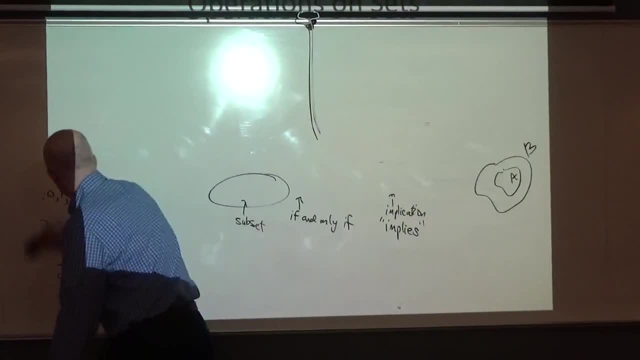 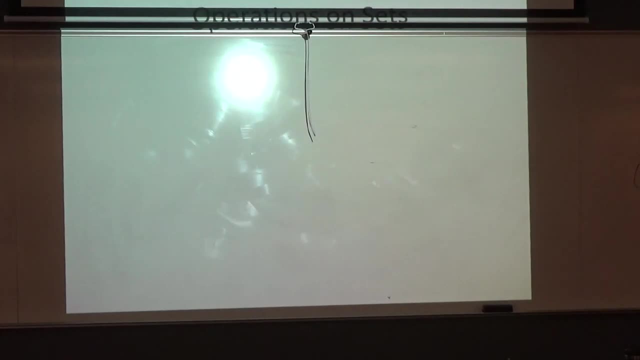 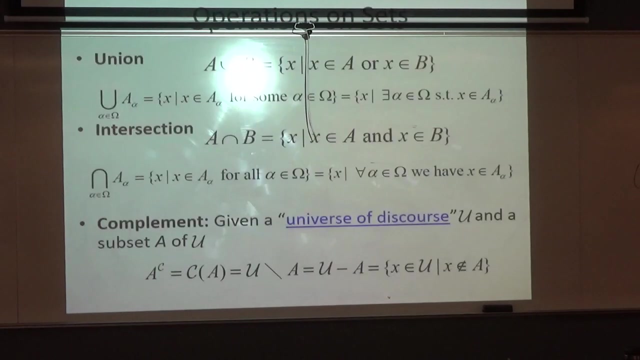 We can do operations on set outsets. I want to go over this really quickly. I do want to get to briefly talking about functions. Operations, what I mean is union, intersection, and complement. Let me just show you the whole page here. 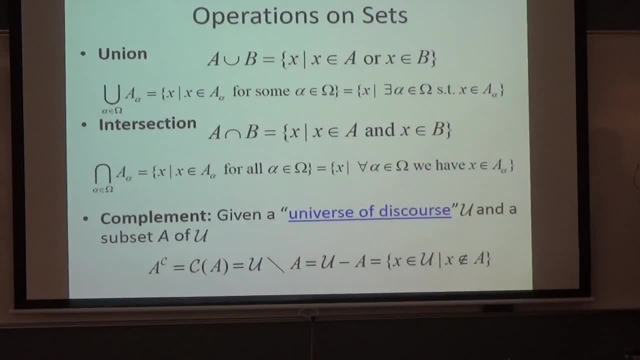 And the notation. A union B means the set of points that are either in A or B or both. 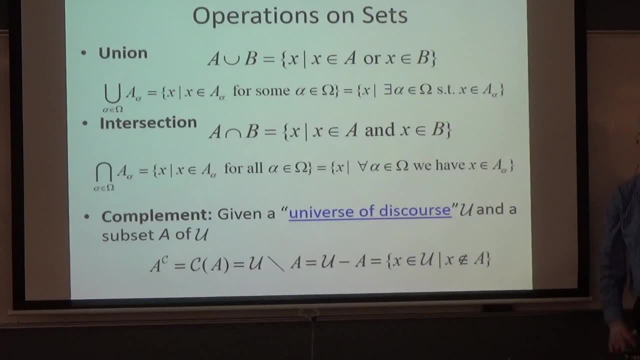 That's implied that it could be both. It's not an exclusive award. 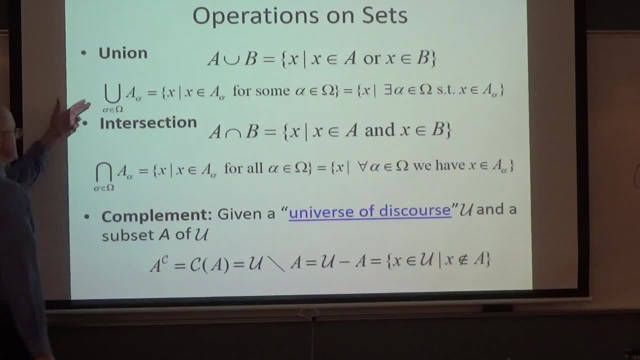 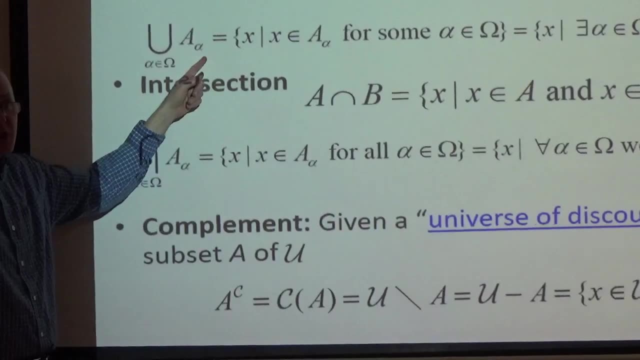 This is a little weirder notation. This is a general union of sets labeled A sub alpha. Alpha could be, for example, a positive integer. One, two, three, four, five, six, seven, et cetera. 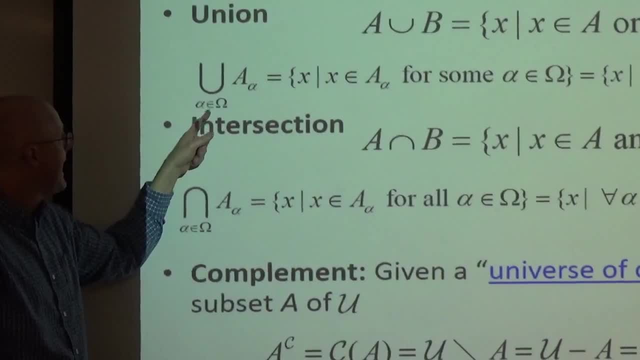 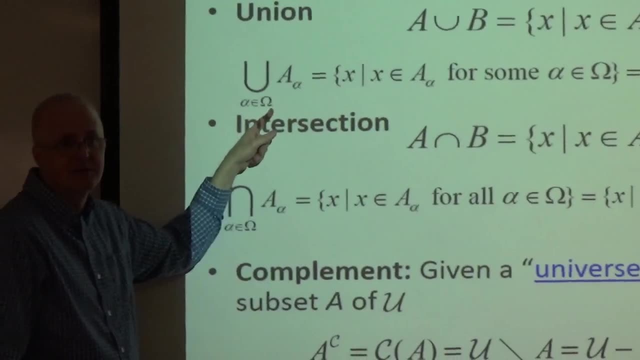 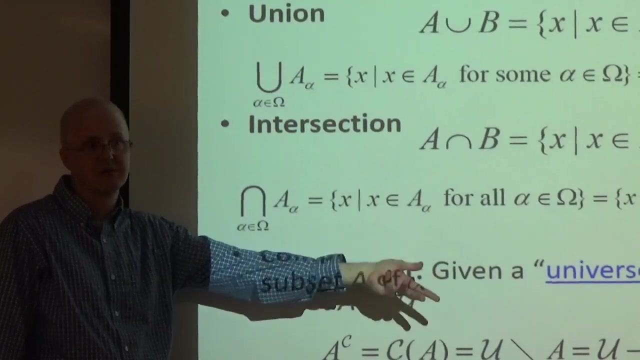 A natural number. As alpha ranges over this set, capital omega, capital omega could be the set of natural numbers. So it could be union A1, union A2, union A3, union A4, et cetera, forever. That's the most common thing to do here. 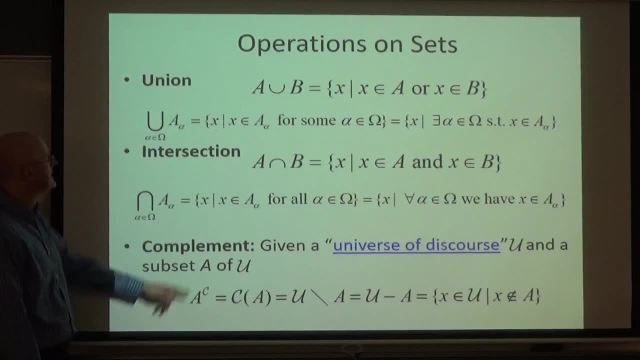 But in general, this doesn't have to be one. The key thing here is this is the set of all points that are in some one of these A alphas, at least one, maybe more. For intersection, it's A sub alpha. 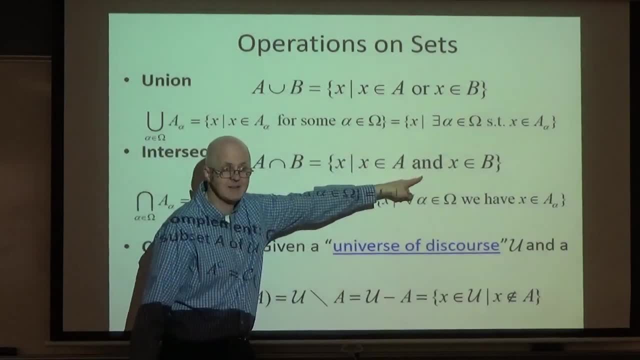 For intersection, you see the or gets changed to an and. The element has to be in both sets to be in the intersection. 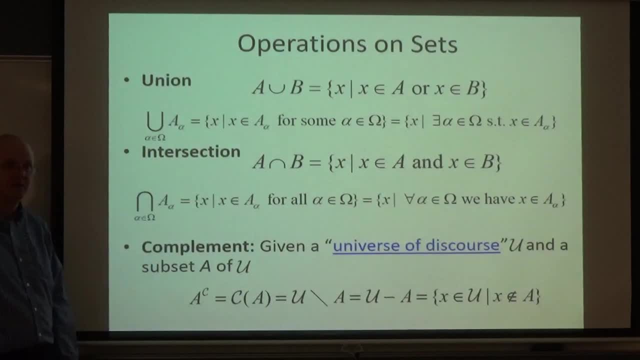 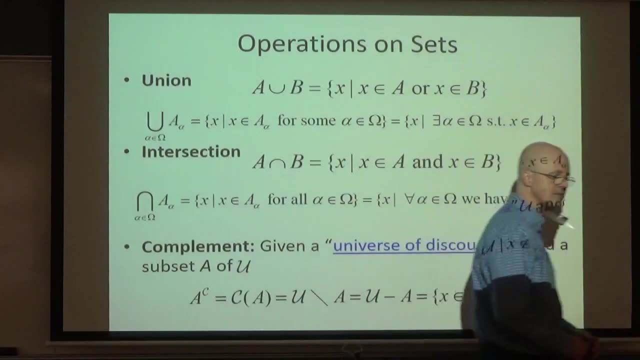 And here you see the for some to get changed to the for all. And I also use their exist notation in for all notation as well. And the complement. Given a universe of discourse, or just universe for short, U, and a subset A of U, the complement of A, which has got all these different notations. Those are just a whole bunch of different notations mathematicians use. 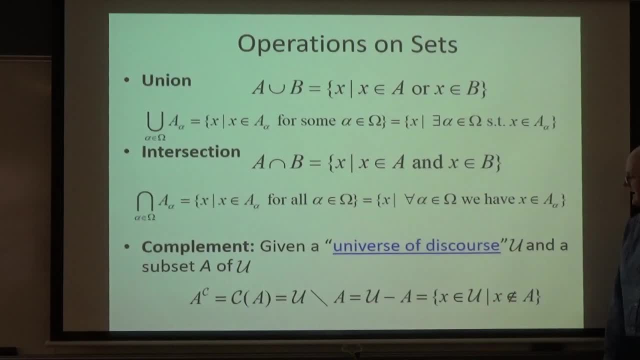 I'm not even sure what's the most common one. I tend to try to use this one, actually. This is the set of all things that are in the universe but not in A. In a Venn diagram, if U is represented by this box here and A is represented by this blob, then its complement is everything in U that's outside of A. Almost out of time. 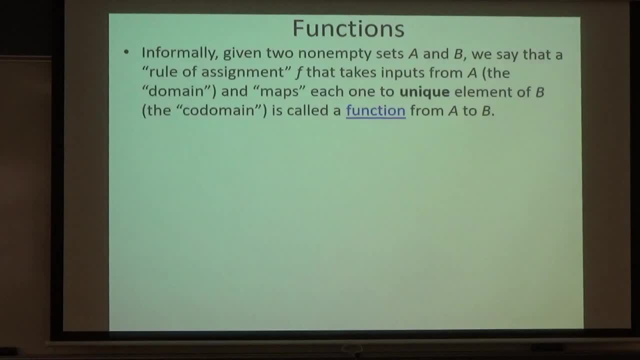 Let me just spend one minute talking about functions as quickly as I can. That's a lot. That's probably more than you can write in one minute. So maybe you should just listen. 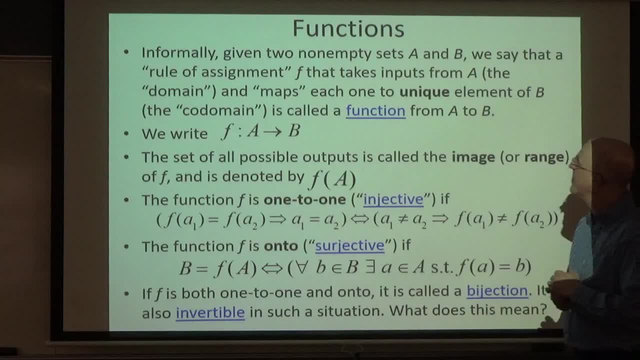 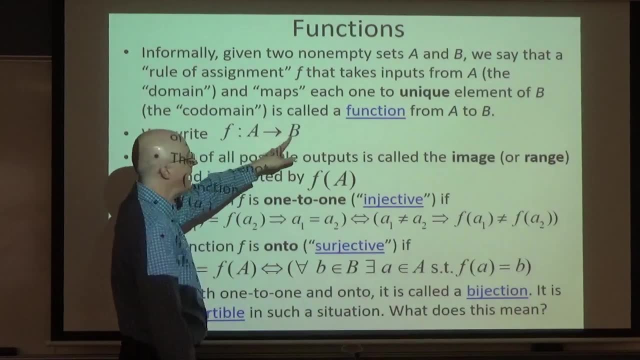 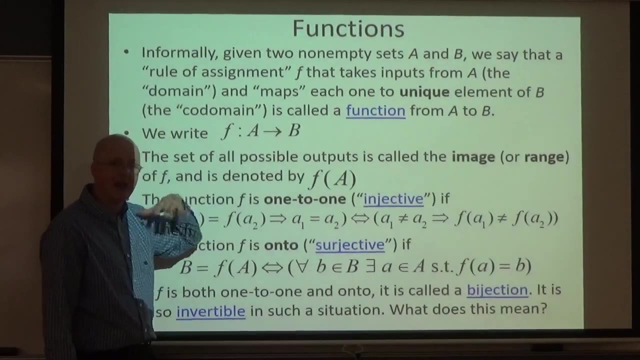 We're going to take an informal approach to functions that you learned in pre-calculus. A function is a rule of assignment that takes elements of some domain and maps them to elements of some domain. This is the domain A. This is the codomain. It's in such a way that it's a unique mapping. 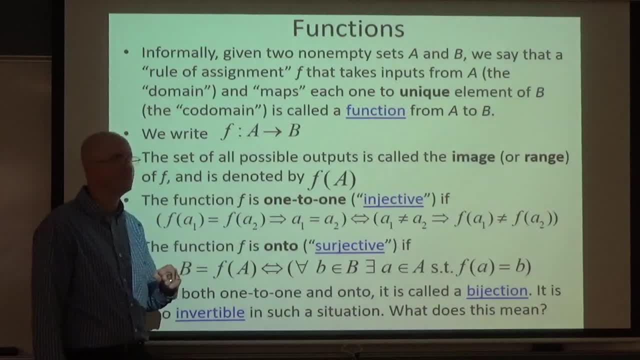 F of A equals a unique thing in B. The set of all possible outputs is called the image or range. 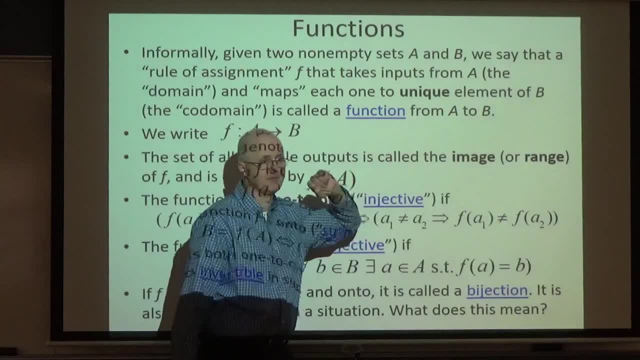 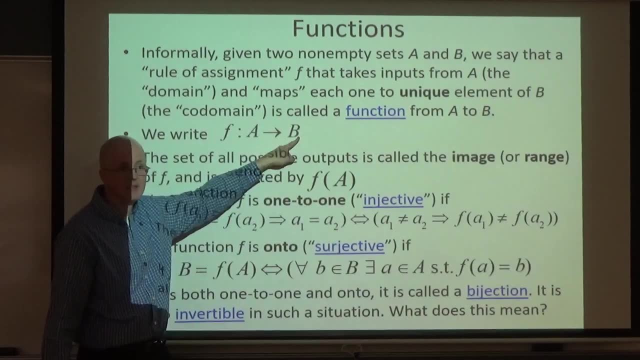 I will almost always use the word image. It's denoted by this. That's not necessarily all of B. If it is all of B, then it's onto. It's an onto function. 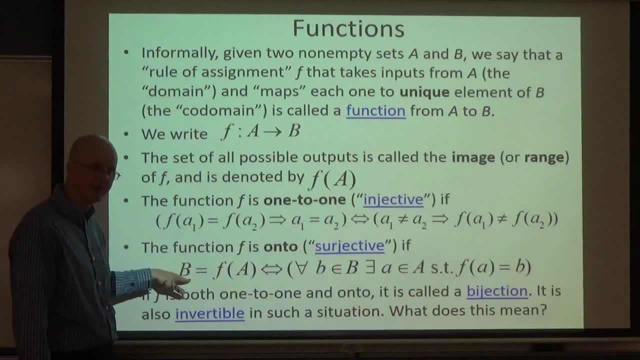 F of A equals B. These are sets of elements. 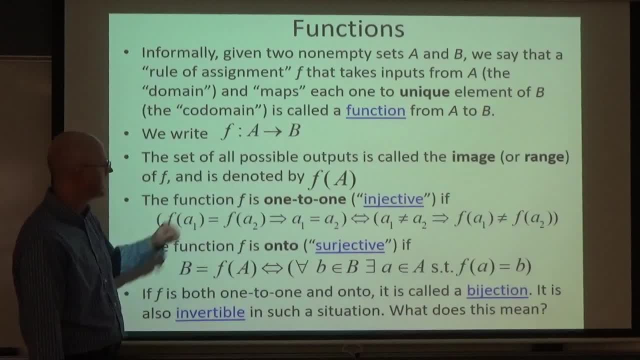 A more official name for onto is surjective. There's also a definition of one-to-one that you've seen before, also called injective. And if it's both one-to-one and onto, it's called a bijection and is also invertible. 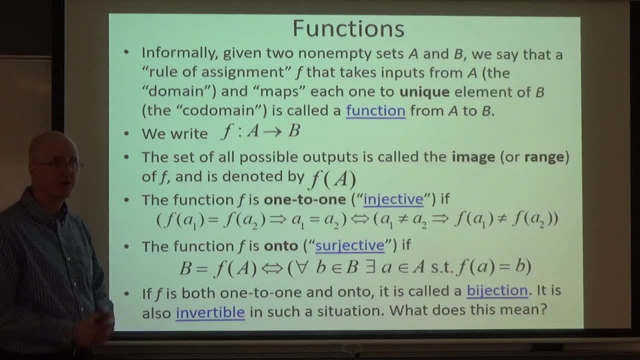 It's got an inverse function. These are all things you should have learned in the past. 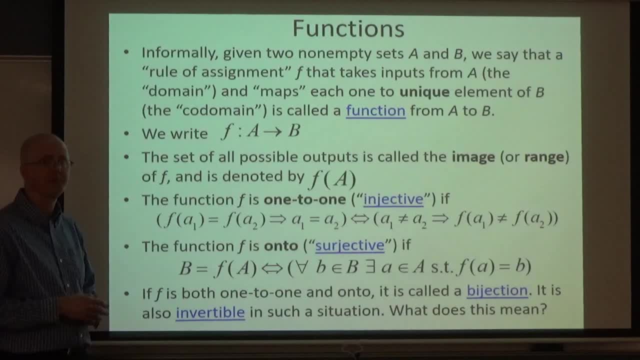 Discrete math. Maybe even precalculus. 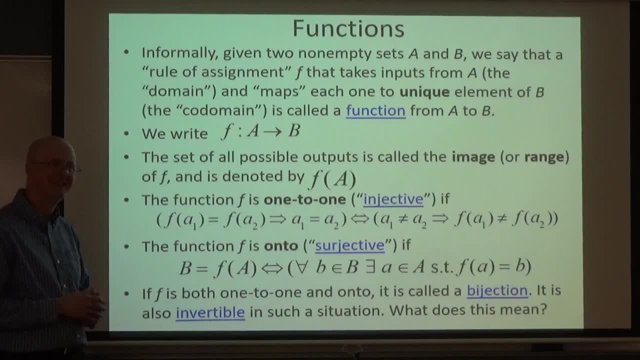 Of course, that doesn't mean you remember them real well. Your graded problems, at least one of them, 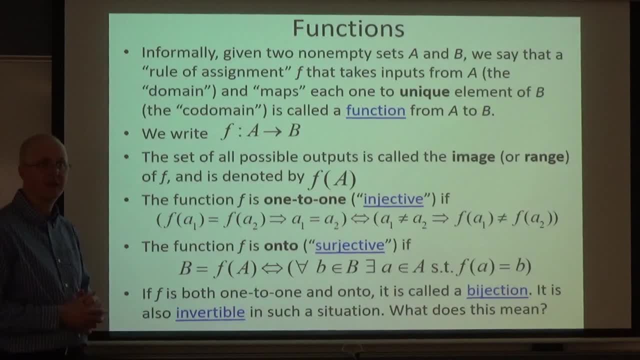 does involve thinking about the inverse function of another function and defining it. 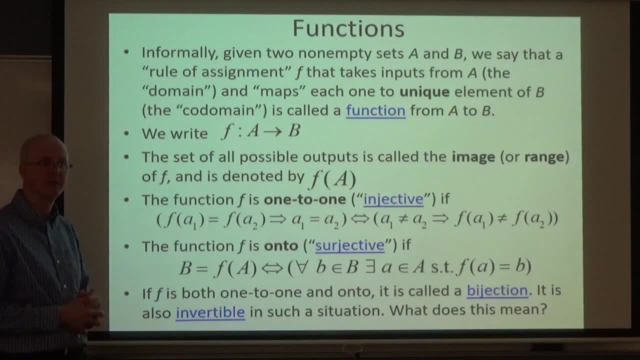 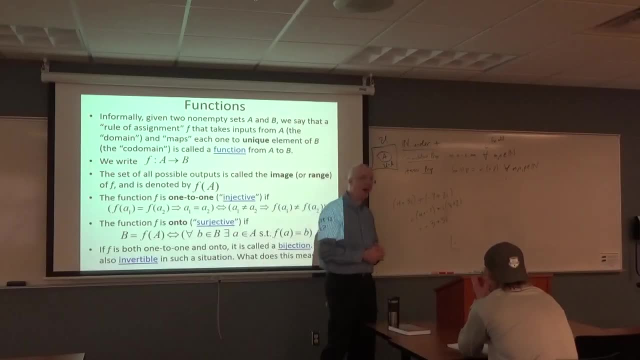 I do give you a hint about that on Mural. So, again, be prepared on Friday to take a quiz on one or two questions on the syllabus and probably three or four questions on today's lecture. I might give you a little bit more guidance on what to expect in the quiz. I might not.